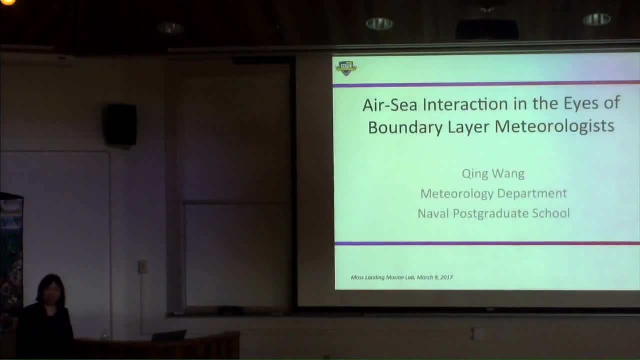 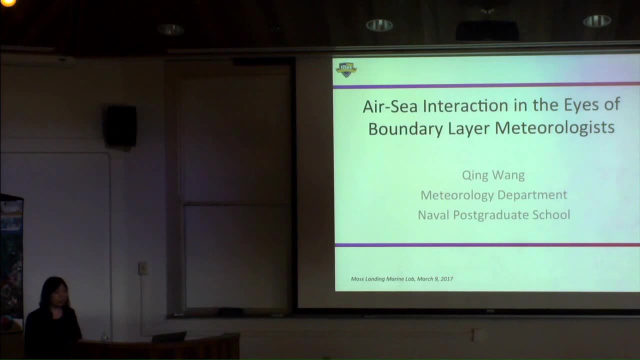 So, talking about the recent field project- and actually it's called Santa Ana Study Project- and we just wrapped it up two days ago. Actually, JD, I think, is still there in Moss Landing, if not transiting back, so that's very, very recent. 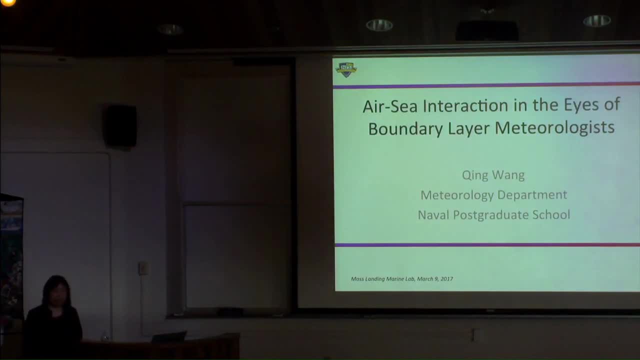 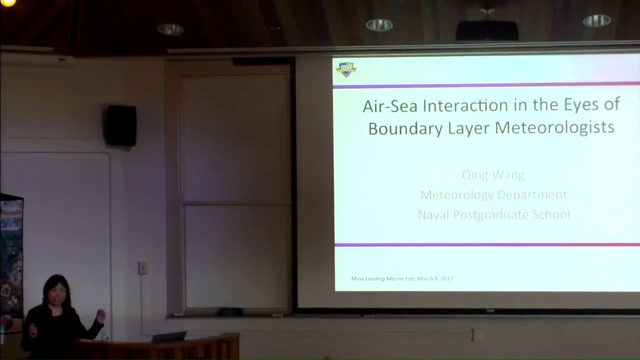 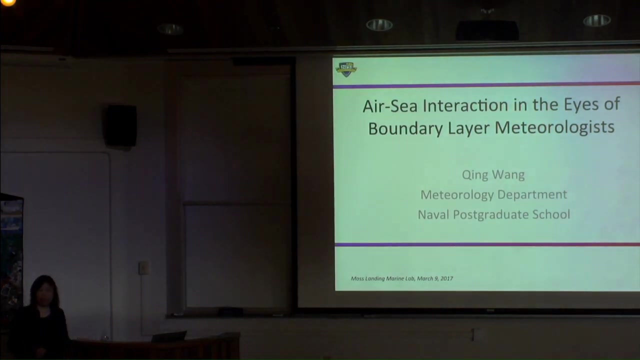 Now. so I want to take this opportunity to you know, introduce in a general sense my research area. so it's not just a name, so you actually know what I'm doing And so I understand you know most of you are not, do not have the meteorology background. 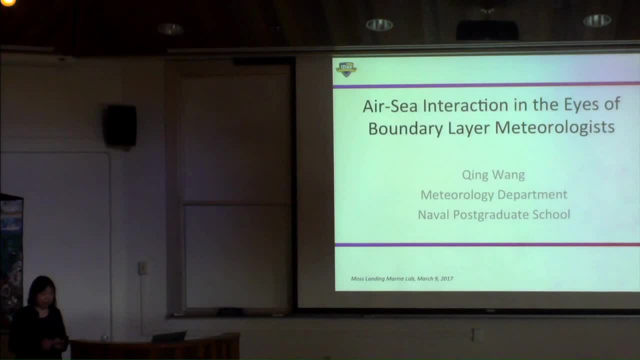 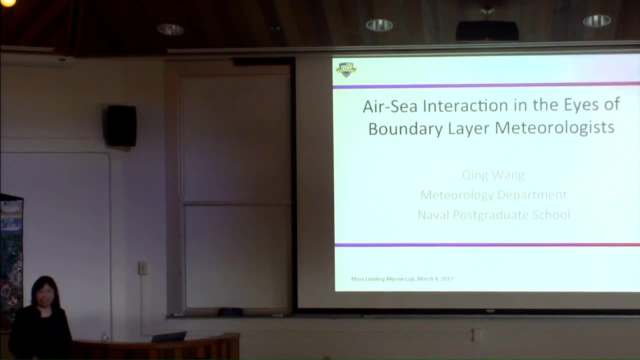 so I'm getting to some of the basics. so, and my research area is kind of broad and has been expanding forever, you know. so I'll try to stay focused with my recent projects. So here I'm talking about the key words. here, you see, is air-sea interaction, and in the eyes of boundary meteorologists, that's what I label myself, you know. 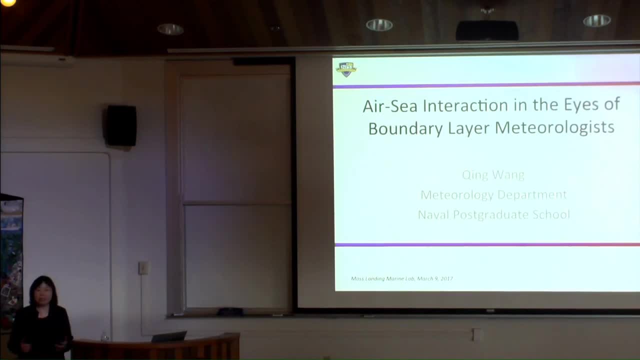 So when people know I'm a meteorologist, they will ask, oh, what's the weather for today? And I say, well, you know I'm a meteorologist. They will ask, oh, what's the weather for today? 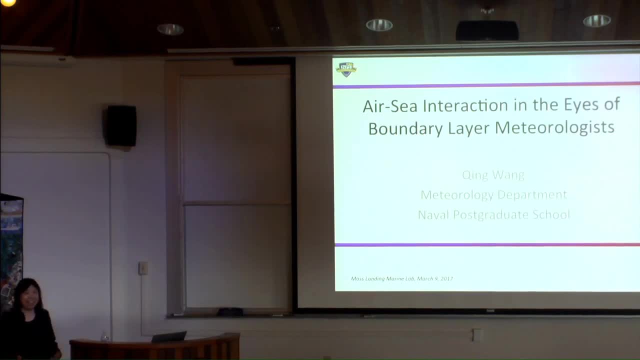 What is going to be a day tomorrow, And I say, well, check the web site, you know, because I'm a physical meteorologist and I'm a more – even more you know- a boundary meteorologist. So what exactly is the boundary layer? and so that's something I will talk about. 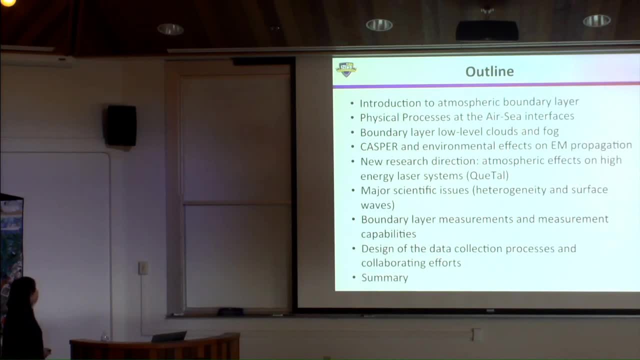 Now, here I will introduce an introduction to the atmospheric boundary. What are we talking about And what are the processes, the physical processes that we are interested at, the air-sea interface, And then I will talk a little bit about boundary, low-level cloud and the fog. 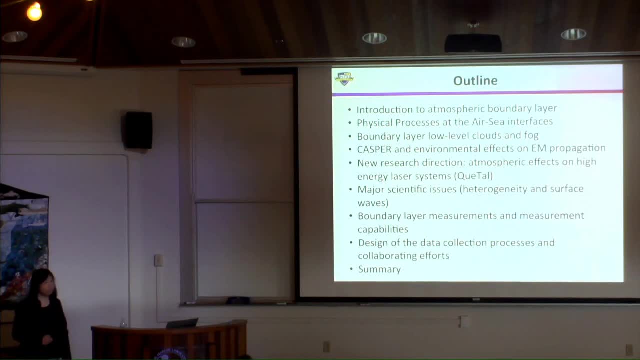 And this is where Kenneth and I identified our common interest. And then I will talk about my recent program, you know, CASPER, and environmental effects on the electromagnetic wave propagation, basically radar propagation in the radio wave range. And then I will introduce quickly about the atmospheric effects. 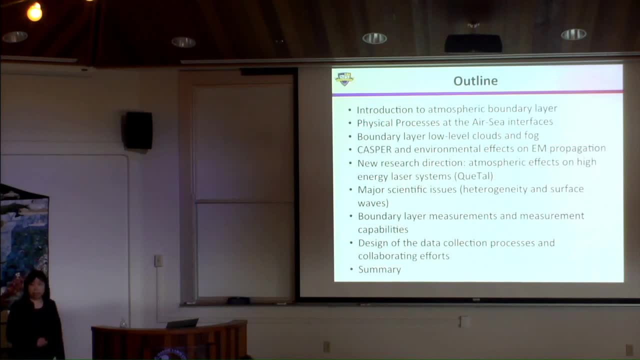 on the optical system and particularly high-energy laser. This is a new project that I was just notified like two weeks ago and funded a five-year project, And so I will talk about. what are we trying to accomplish? what are we dealing with in this boundary layer? 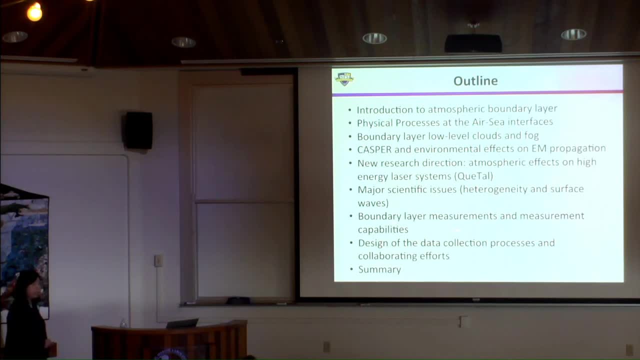 And then the importance of boundary measurement and what we do with the measurement and how we design the data collection process And sometimes we work with. you know new ships that are coming in, You know ships that are new to us, or you know? 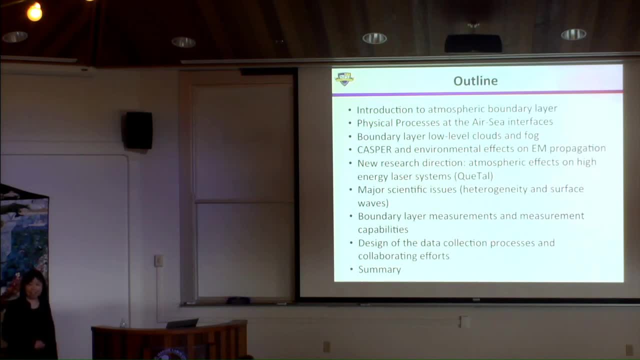 so they feel what we are doing are really bizarre. It's not the normal. you know doing a CTD cast, And so you know they will say what you want to do- a balloon on a small ship. And so we're doing some strange things, but it's all fun. 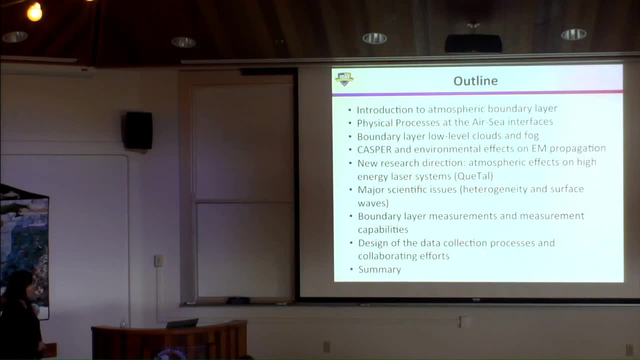 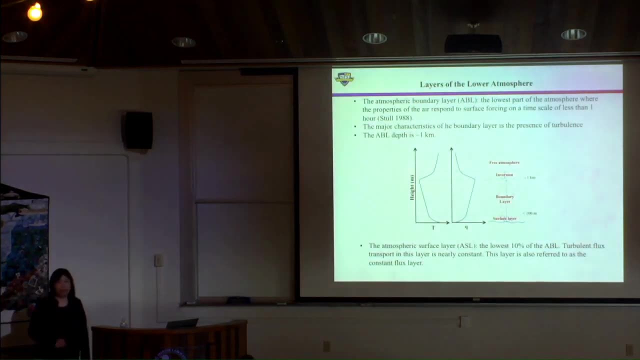 And so Alex can tell you So, and finally, I will give a summary. So now, what is the boundary layer? So, the atmosphere, okay, and invisible, but we can separate it into many layers, okay, And this lowest, deep layer is what we call the troposphere. 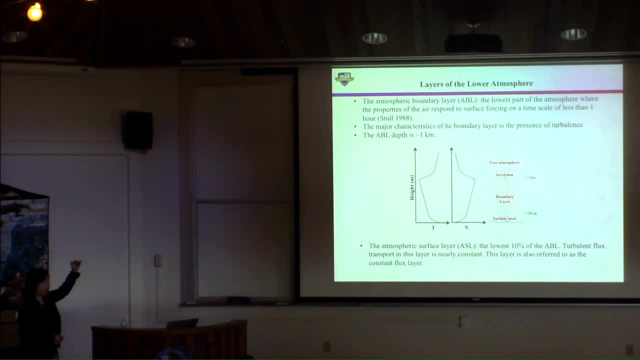 and many of you know Now, the boundary layer is the lowest, one kilometer of that troposphere and its basic major characteristic is in direct contact with the surface and, as a result, is turbulent. So what you know if we look into a layer? and we see it's not turbulent. and then that's not the boundary layer of the Earth system. Okay, so what? so that's the major characteristics of the boundary layer: it's turbulent. So now the formal definition of the boundary layer is: it's directly affected by the surface. 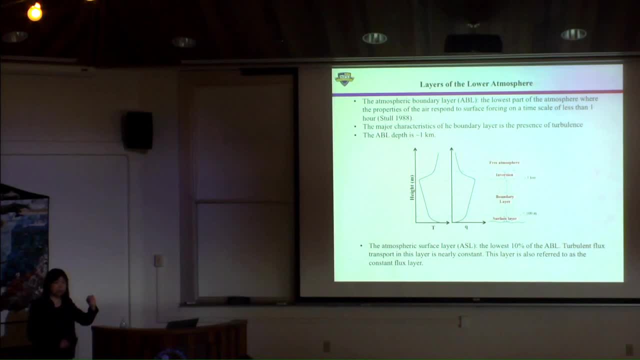 and also its response to the surface within an hour. So there's a. I'm sorry I forgot to Let me just. If that's for me, you just tell them. I'm busy right now. I'll just put it there. 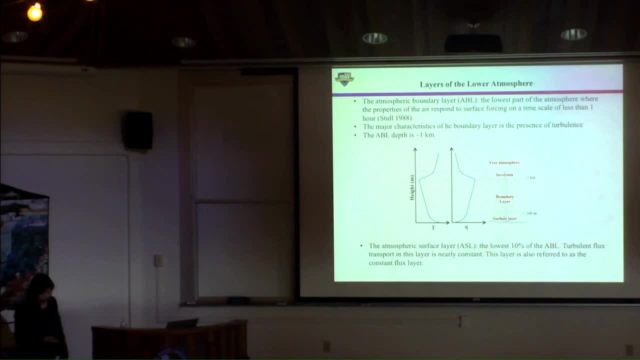 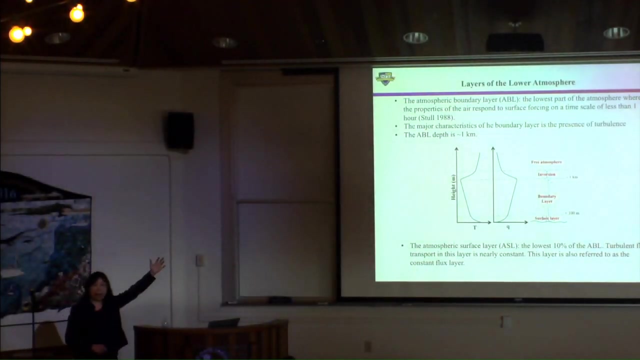 Okay, So that's the directly, you know, affected by the surface and response to the surface forcing within an hour. This time scale is very important because eventually, everything in the upper atmosphere is going to feel the effect of the surface and the ocean. 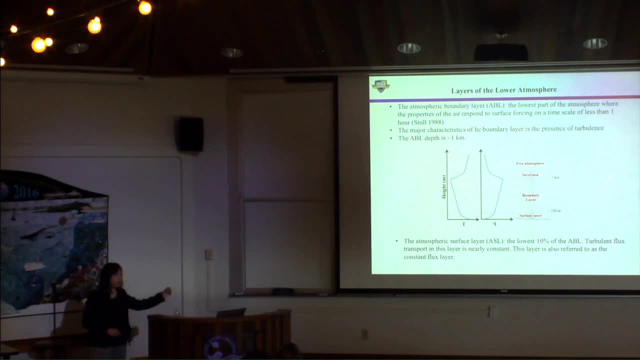 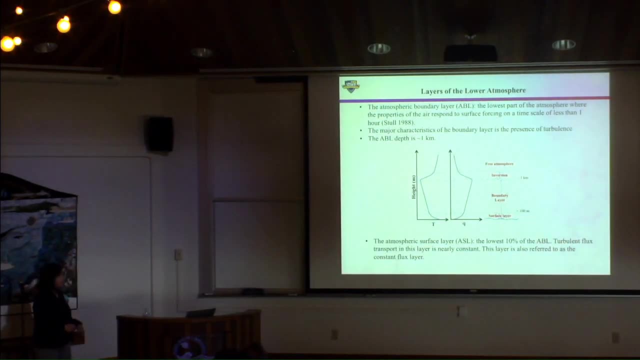 Okay, it's just a matter of how long. Now in the boundary layer, you feel it right away. basically, Okay, so that's where it makes a difference between the boundary layer Now in the boundary layer here, and normally we have something at the very top. 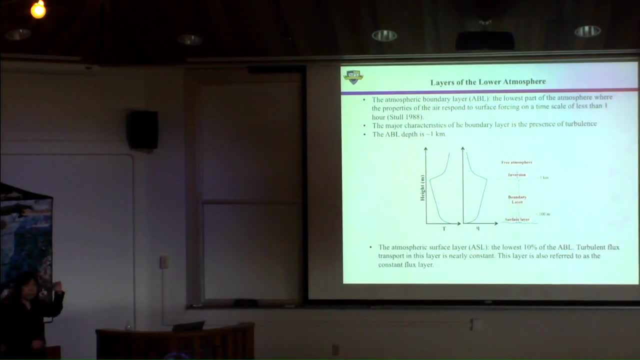 you know this has to. we call the temperature inversion. This is, you know, temperature normally decrease with height, but in this layer it's increasing with height. So we call it a temperature inversion And accompanied with that and we have the water vapor decreasing with height. 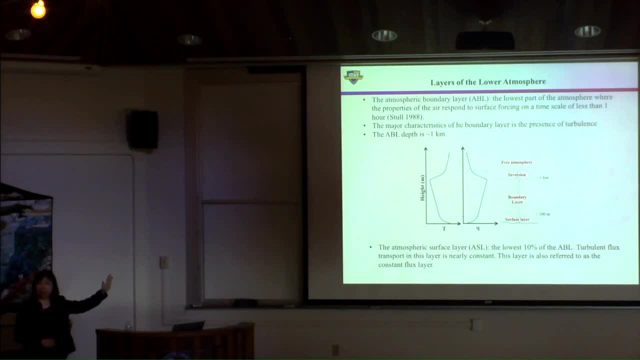 So it's getting drier above, And this is particularly true, of course, over the ocean, because we have a big source of water here, Okay, And within this layer, and then we also separate it into. you know, this part is called the surface layer. 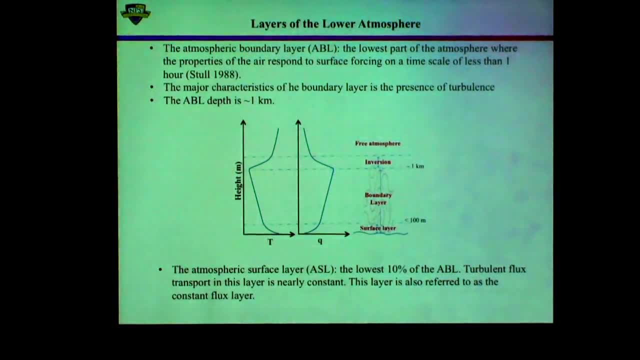 which is really directly in contact with the surface and it really feels what's going on in the surface, And this is normally like 10% of the entire boundary layer. So if we do the math, one kilometer is the normal height of the boundary layer. 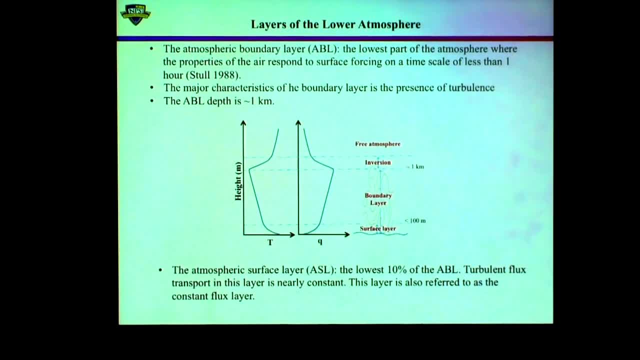 10% of that is about 100 meters. So we're talking about this lowest layer is 100 meters. Now, what you see here in this lowest layer, water vapor. you know we have a strong gradient, You know. so I think this labeled wrong. 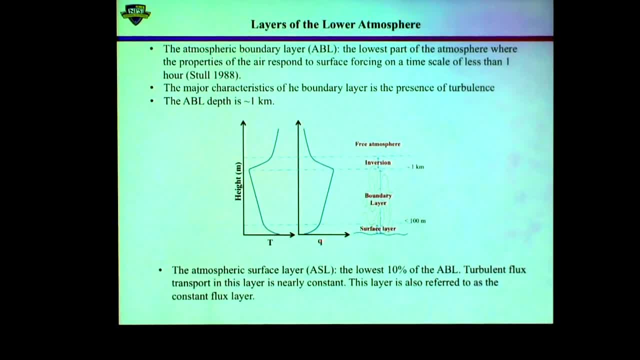 Hold on, Q is So, this should be Q and this should be temperature. So, anyway, in this layer, and we see the strong gradient. Okay, It varies with height significantly, And lots of times it's the vertical variation that we are interested in. 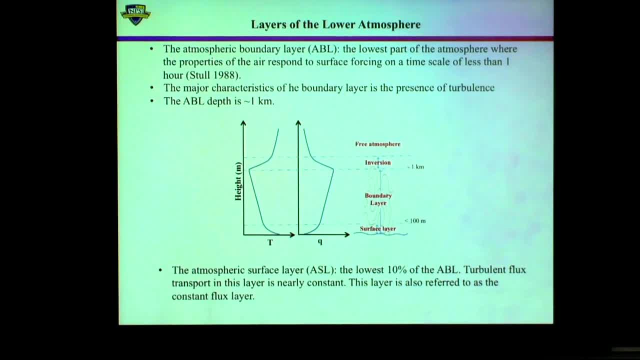 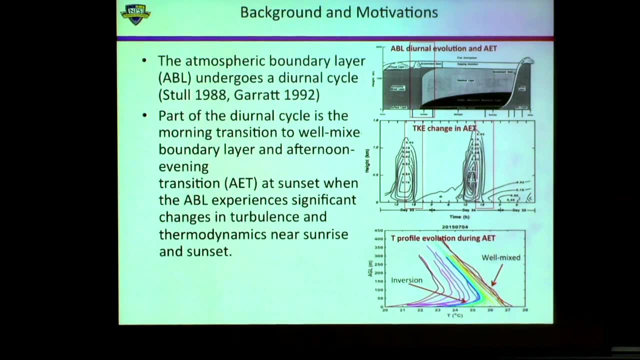 And we see that as boundary meteorologists. So now what's going on in this boundary layer? As a result, it's responding to the surface quickly. So we see the strong diurnal variation, So during the day when the sun rises, and then that's when we have, you know, 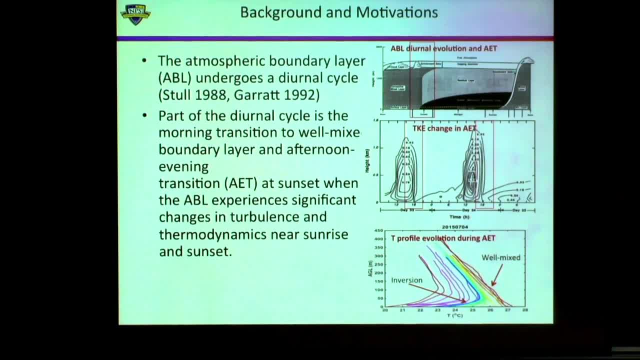 the boundary layer will evolve. You know, you heat up the surface and then you see you get lots of mixing and turbulence And then at night and the surface cools and you develop a different type of boundary layer. So we have this very strong diurnal variation. 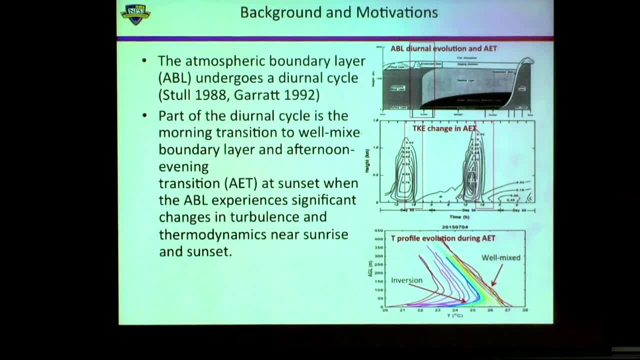 And at the sunrise and the sunset, and then we are going to see very strong, you know, very quick development of the boundary layer. Now this is not completely true over the ocean, because the ocean surface do not have such a significant diurnal variation. 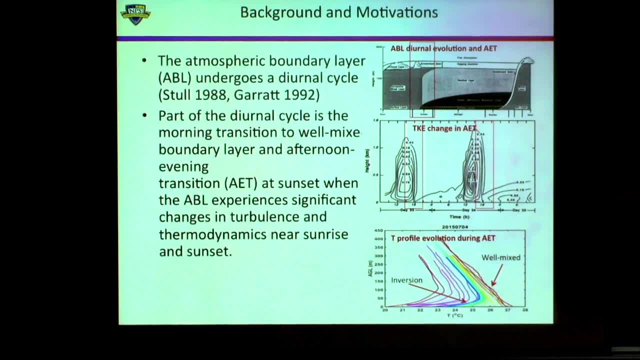 But over the ocean we do have some diurnal variation in the sea surface temperature And it's just not as dramatic, as you know, over land. Now this is from my measurement with the tether balloon over Kansas, So you can see, you know this is during the day. 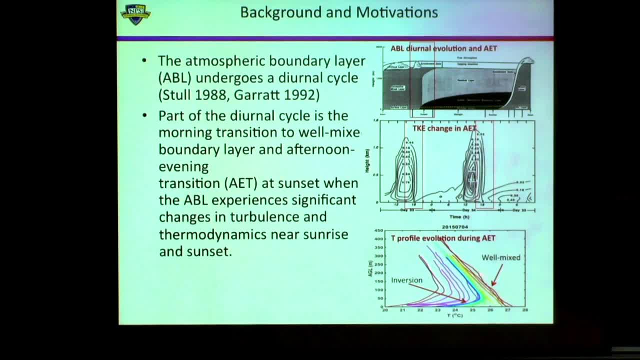 The temperature goes like this, And then right at sunset, and then now you start to see this development of the stable boundary layer because the surface is cooling very rapidly. So the temperature is cooling off very rapidly. So that shows, you know the response. 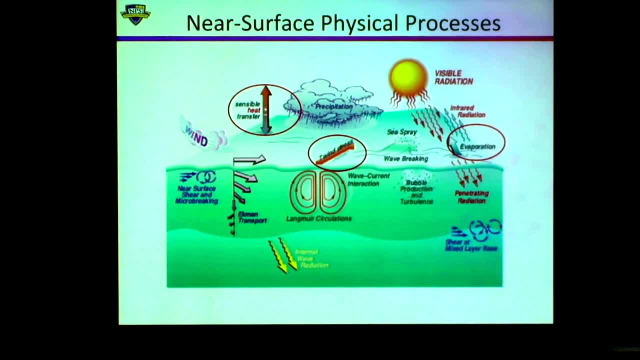 of this boundary layer to the surface, forcing Now, so near the ocean surface. what's going on? Oops, wrong button. So now these are the processes. we're looking at, the physics involved And, of course, in the upper ocean. 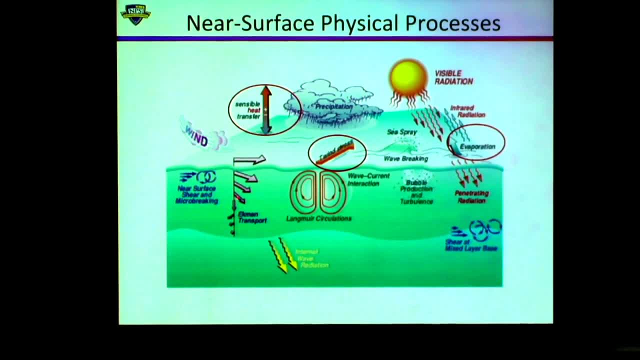 we have the circulations and we have the Ekman transport gradient and you know there's waves and all that, And then at the bottom there's the bottom effect. So Tom is an expert in that. Now, this is my territory when it comes to here. 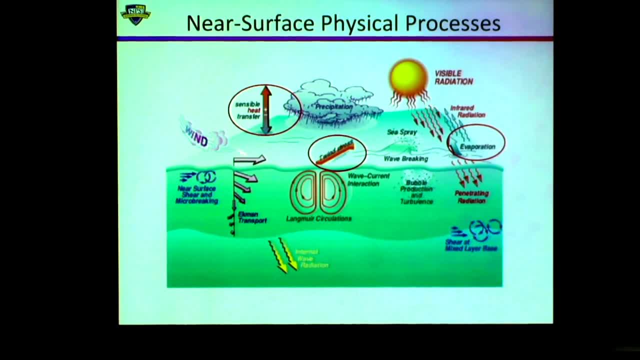 And so now, at this interface, now we have the wind, And then now this wind, you know. so this is the forcing from the atmosphere to the ocean And as a result of that, it generates this momentum mixing, So that takes care of the momentum transport. 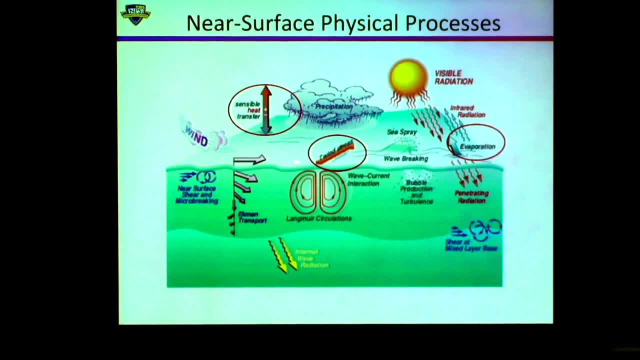 between the atmosphere and the ocean, And that's this surface stress part. And then we have also, you know, because there is an air and sea temperature difference, so you are going to have this sensible heat, you know, transporting Either way, it can be plus or minus. 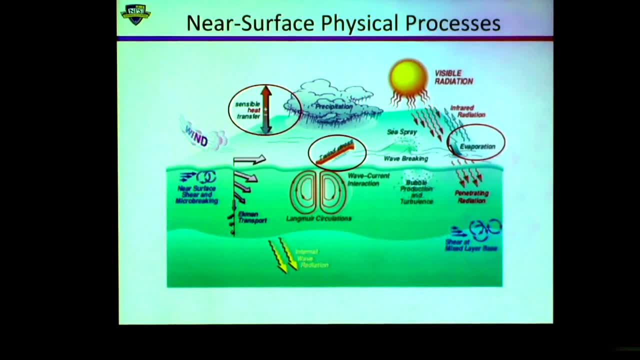 because when the ocean is warm and the air is cold, so you have the heat coming from the ocean, And when the ocean is cold, atmosphere is warmer and then you have the heat going into the ocean. So that's the two-week traffic. 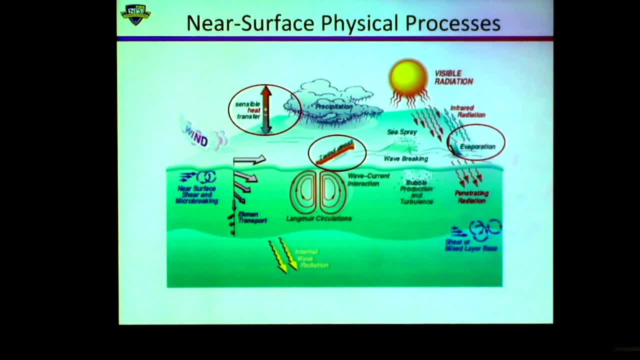 Now then, when we get into the evaporation part- and this is most of the time it's a one-way traffic- You know the surface is evaporation, So you have water vapor into the atmosphere. This is extremely important to atmosphere. 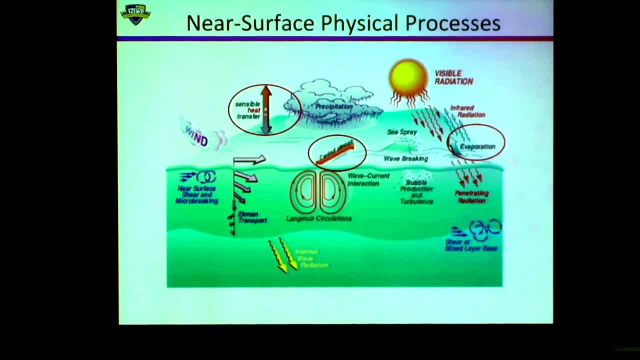 especially to the. you know, especially when we are talking about hurricanes, for example, because the precipitation and the rain development it depends on this water vapor. So the different ways you can model this and then that's going to change the intensity. 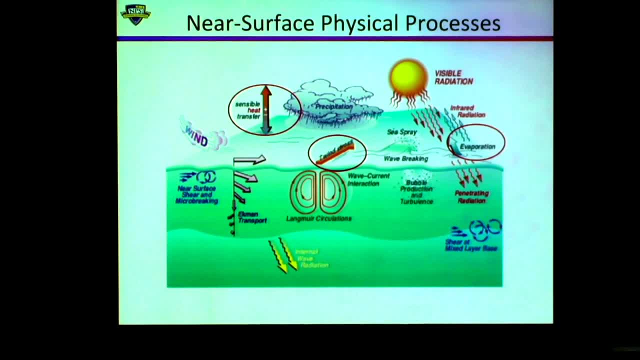 and also the track of the hurricane. So, and this accompanied with this evaporation, in addition to the water vapor input into the atmosphere, and we also have the heat, Because when you evaporate you need heat. That's the so-called latent heat flux. 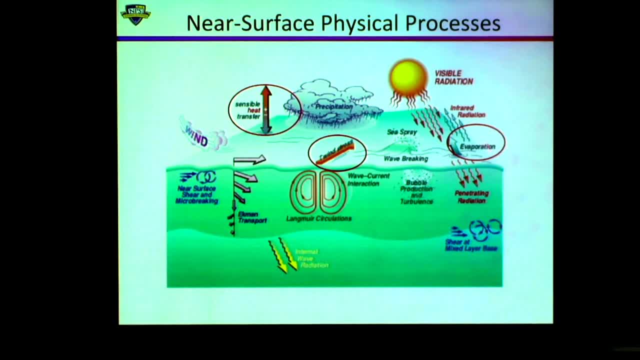 So now I have, all these three are circled in this and these are the ones we have been trying to measure. So when you see those sound anemometers, we put on the John Martin and we put some light core to measure the fast water vapor. 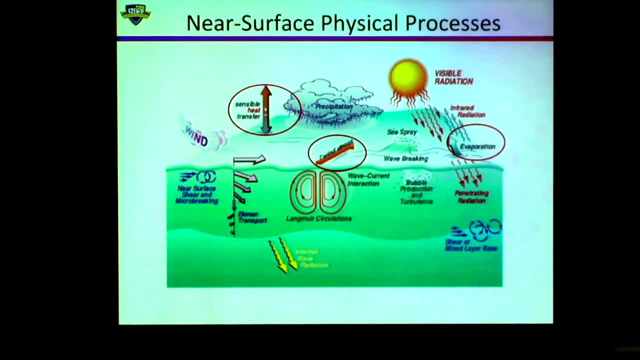 and those are really for measuring these three quantities. Now, why are they important? Okay, now, when we talk about how the atmosphere and ocean are coupled, and these are the couplers, So these are the mechanisms, and ocean and the atmosphere exchange momentum. 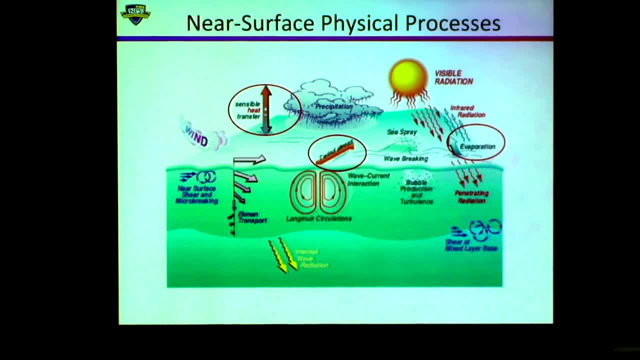 and sensible heat energy and the latent heat energy and mass of the water vapor. And some other people are interested in the CO2, and that's in the form of the flux, you know, from the ocean as well. So we I always measure CO2,. 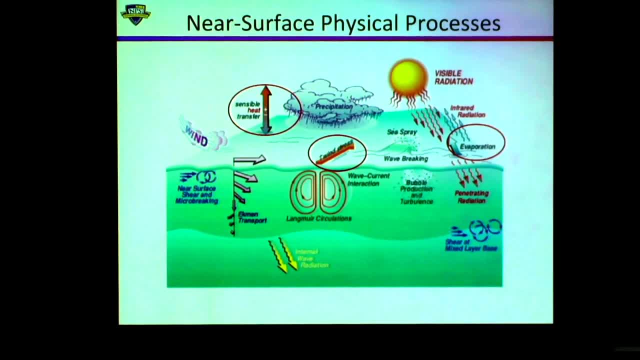 because that comes with the sensor, but I have no idea how to explain them. So, if you ever need CO2 data, I have lots of them, just I don't know what to do with them. Okay, so that's the ocean. 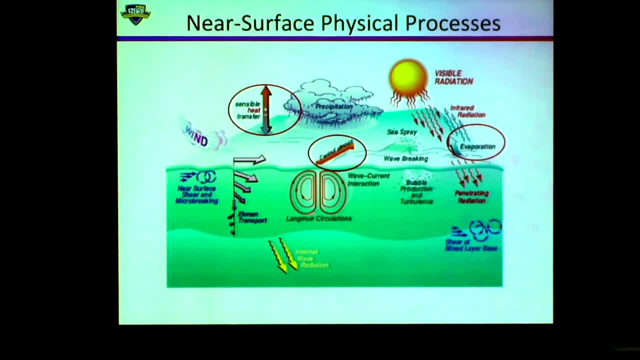 the air-sea interface. you know the processes And so in the forecast model, these are the three. So the forecast, the forecast model, need from boundary meteorologists like me, And so they want to be as faithful as to the true atmosphere as possible. 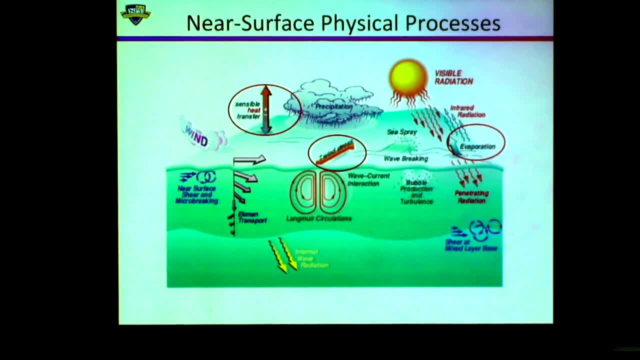 That's what we call the surface layer parameter, surface flux parameterization. So now this parameterization is an issue because there is a a scale mismatch, because these things happen at very small scale. So we're talking about millimeters, centimeter to meter and kilometer. 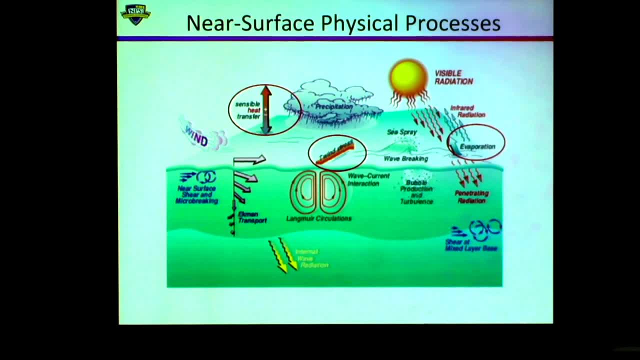 Okay now. so the forecast model. and they cover, like you know, the fine resolution. We're talking about three kilometer. you know operational forecast five kilometer. So all these processes are the so-called subgrade scale. 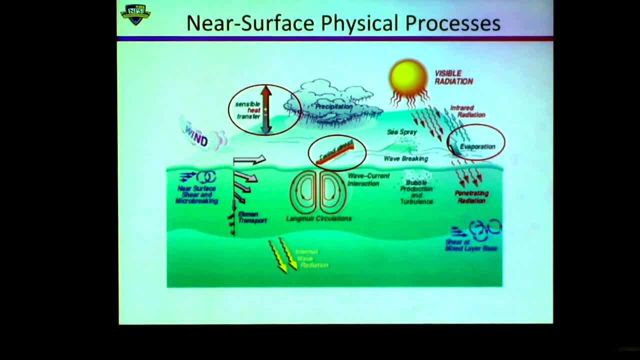 Okay, so the forecast are on this scale, but the processes we're looking at on this scale, So we somehow need to make the connection between what's going on here to what's being forecasted. Okay, so that's the flux parameterization. 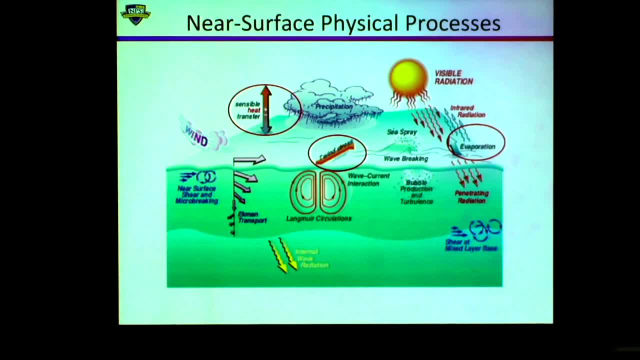 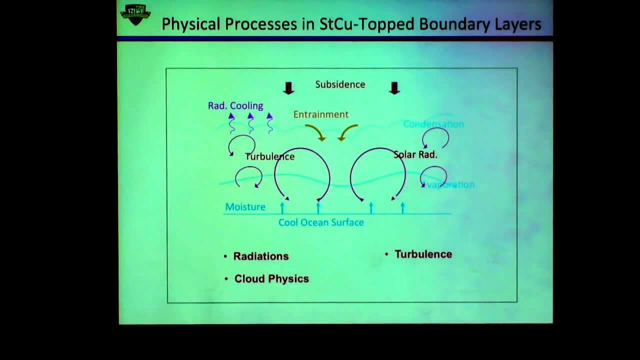 and that's where lots of the research has been done. you know about the surface flux parameterization: Okay. so now when we get to the upper boundary layer, okay, and then we get into the so-called turbulence transport and sometimes, and we have this layer of cloud. 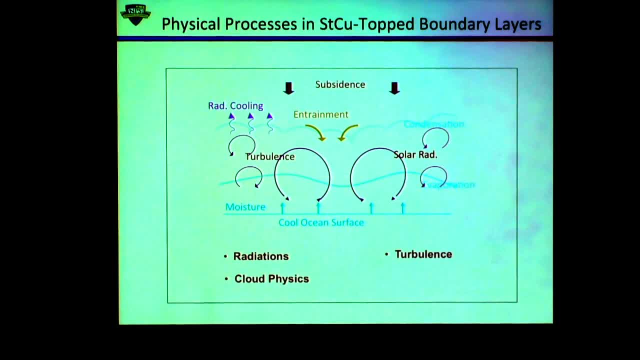 Now, when this layer, this layered cloud, when it gets really low, it will get down to the surface and that becomes, you know, what we know as fog, And we are particularly interested in these, you know, because we have lots of these. 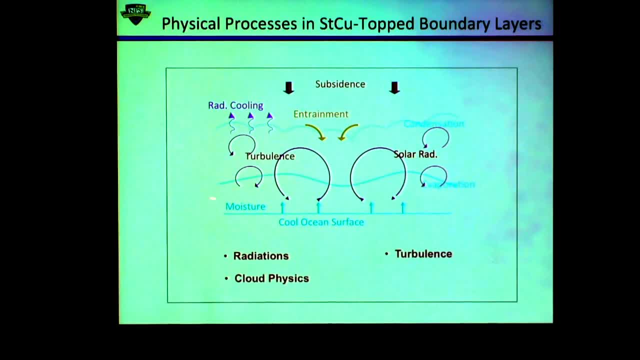 you know, on the west coast and particularly in the summer period. Now what happens here? you know, during that period the larger atmosphere has this large scale slowly descent. so it's just pushing the air, you know, slowly And then, but you don't see the atmosphere. 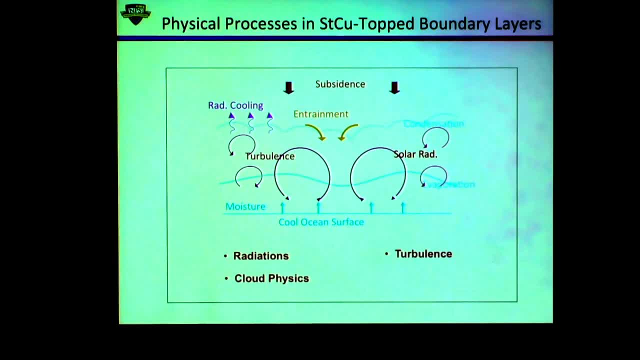 is being crushed to the surface because there's something going on in the atmosphere. now. what's going on here now you know, is that you know if you have a warm ocean surface and it's going to give some buoyancy. 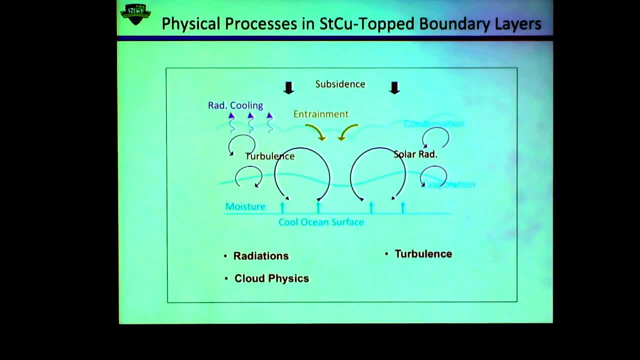 you generate turbulent mixing, so that's mixing going on Now if you don't have those. so normally what we have here- the ocean surface- are pretty cool Now, but we have this cloud Now. what happens here is the cloud, you know. 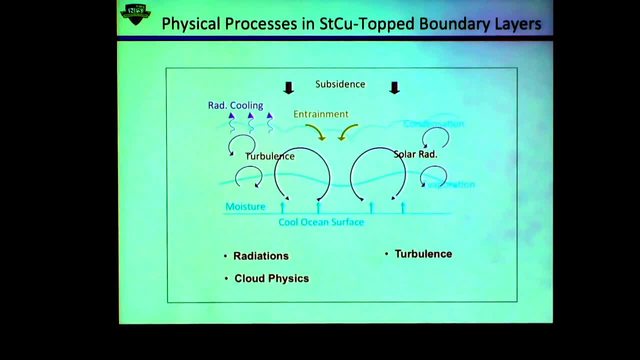 is, everything is emitting infrared radiation. So you, the chair the table, everything Now the cloud is emitting to the space and the same time you know it's receiving emission from the air. But you know the amount cloud emit is a lot more. 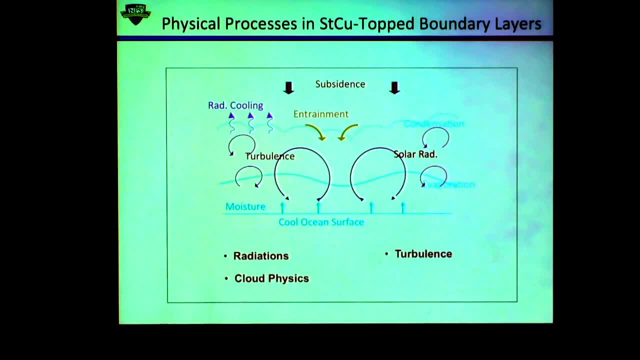 than what they can receive from the air. So, as a result, at the very cloud top, we're talking about meter to 30 meter range and there's a net loss of energy at the cloud top. So if you have a net loss of energy, 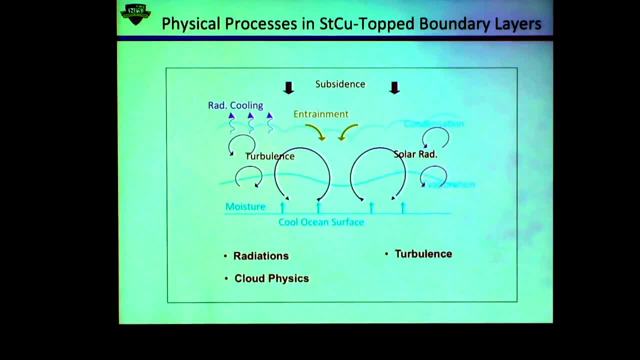 what's going to happen? it's going to cool. So if you have the air, it's the, you know it's top heavy because it's colder, and what happens is it generates turbulence. So the turbulence you see now when you are under the stratocumulus cloud, 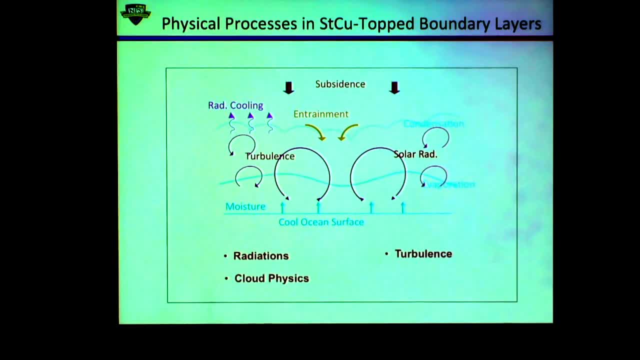 it's mainly generated by what we call the infrared radiated cooling at the very top, So that generates the turbulence here And so this in addition to that, and we also have, you know, the moisture supply from the ocean, and it's always there. that's important. 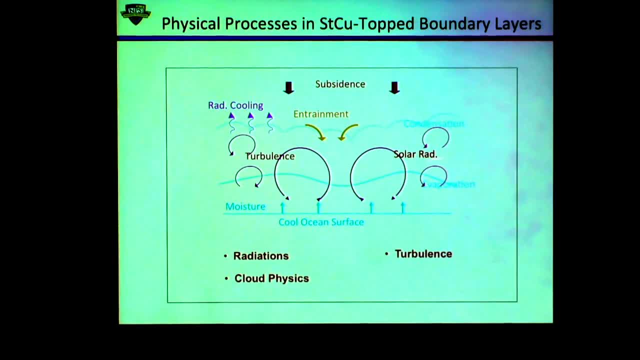 because that determines how long this cloud is going to stay there, okay, And because you know you also have the so-called entrainment process. Now you have all this quiet air above, and then you have all these turbulence eddies. 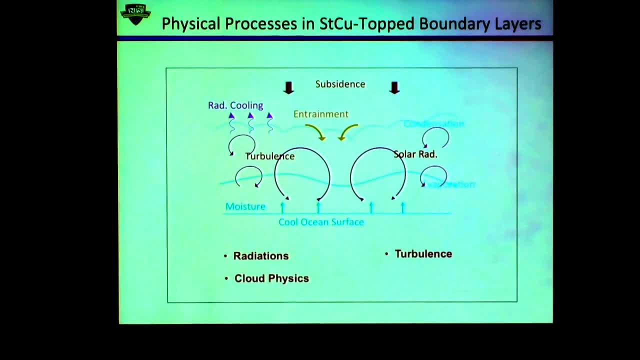 you know, in the boundary layer What's going to happen is all these eddies is going to scoop some air from above and incorporate that into part of the boundary layer. As a result, your boundary layer has a volume increase and guess what? 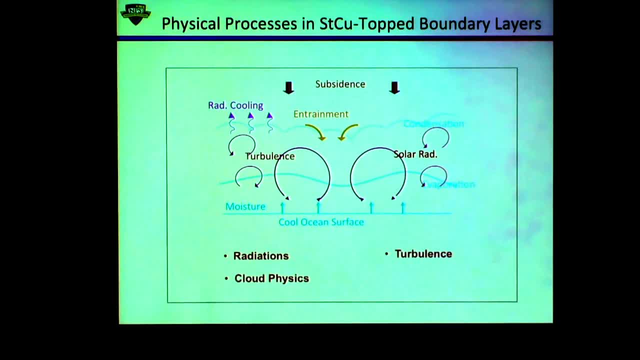 Your boundary height is increasing. That's why, you know, with this constant pushing from the larger scale, you know substance and we're. you know it's not pressuring the whole boundary layer to the bare surface because we have this turbulence. 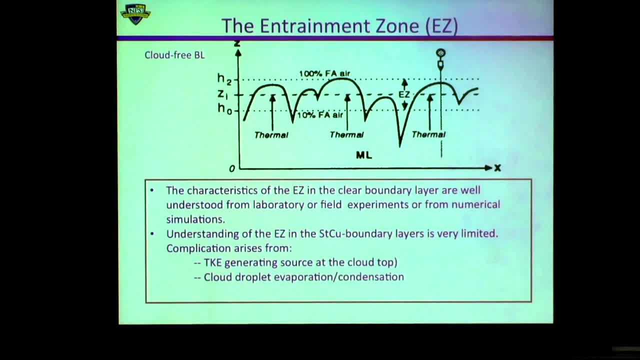 you know entrainment going on, And so this is a picture of the entrainment in the clear air and it's basically in simple words. it's just, you know, you scoop some air from above into part of your boundary, you know. 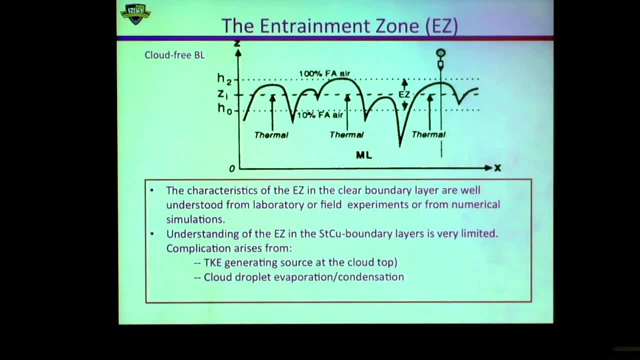 because you have turbulence motion And when you have cloud this is harder to deal with and you know this is part of my thesis research. you know, when I did my PhD and I continued to work on that for many years after. 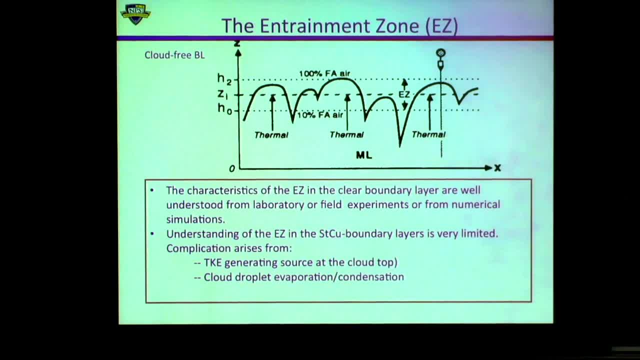 So when you have a cloud and then your source of turbulence is up above, but this is where you bring the dry air into. you know your boundary layer as well, So it become a lot more sophisticated than in the clear boundary layer. 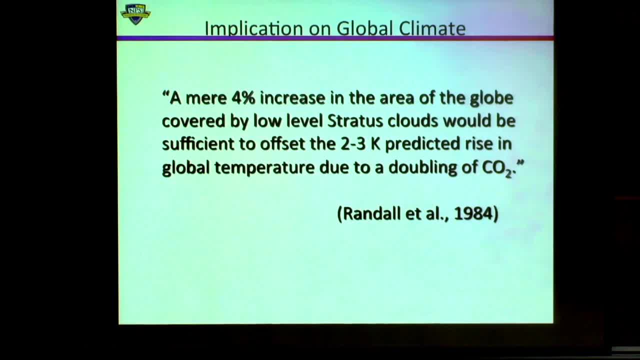 So lots of research are going on in there. So what's the significance of a boundary layer cloud? In the past 30 years also, you know, the National Science Foundation and also the Office of Naval Research, you know, and also DOD has put in lots of money. 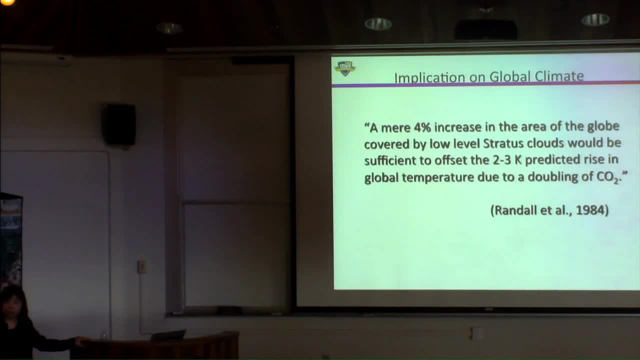 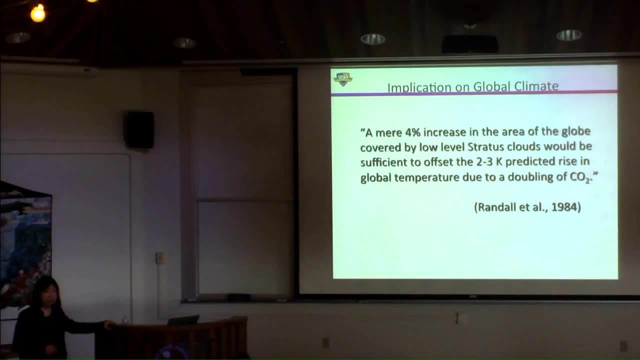 into studying the low-level cloud, like stratocumulus cloud, And which is good for us. You know that means funding, And so now, and lots of those were driven by climate change issues. Now, this was the research from back in 1984.. 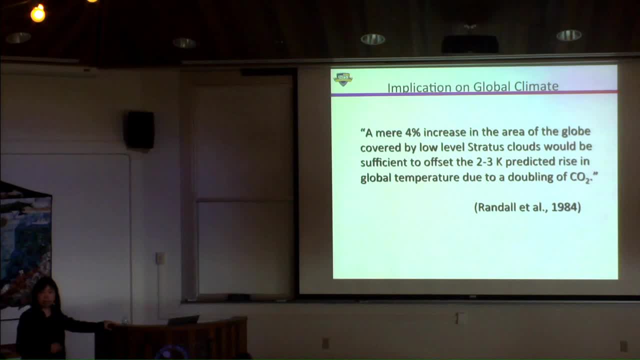 So they found now these low-level clouds. if they are the percentage increase by 4%, which is easily, you know, getting there, and then it's enough to offset the effects of doubling the CO2 for global warming. So these clouds, they have a cooling effect. 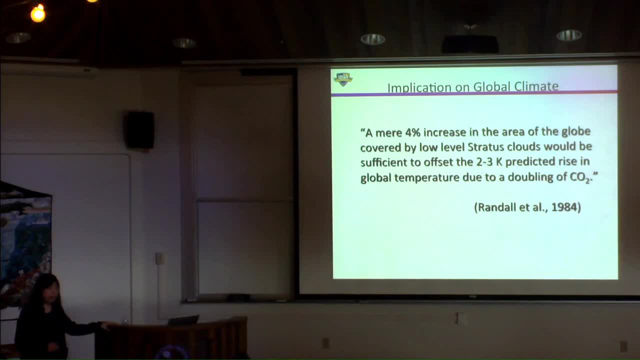 for the climate. Now why? Because these clouds are low, so the cloud temperature are not too different from the ocean surface temperature. So in terms of outgoing radiation it's about the same, you know, as you don't have cloud. 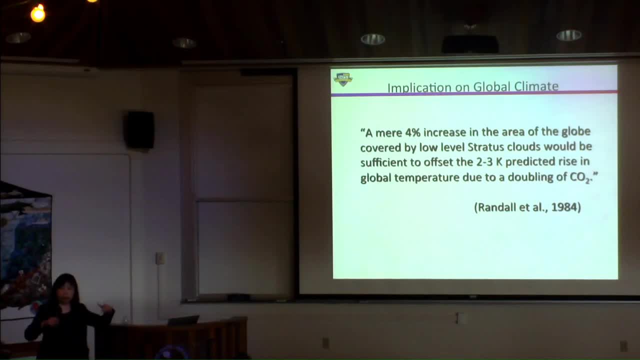 But if you're looking into the solar radiation and how much the Earth system is going to get, these clouds are much more reflective than the ocean surface. So, as a result, we're not losing as much of the infrared radiation, but we are not. we are getting much less. 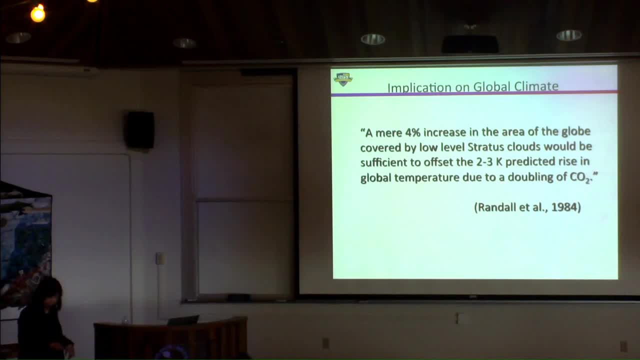 you know solar radiation. So as a result, climate-wise, you know. so you know it has a cooling effect. So that's the drive for many of the past: the research on stratocumulus cloud, Now the Navy, and you know lots of. 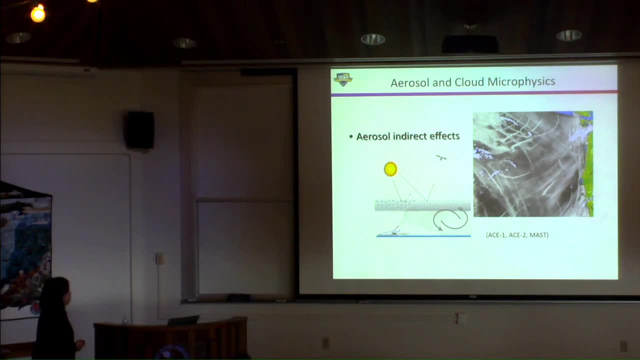 and DOD also have an interest in the effects of aerosol on the cloud microphysics Now. so what you see here is, if you have a ship plume and then, so that means now you have lots of small particles that the water vapor can condense on. 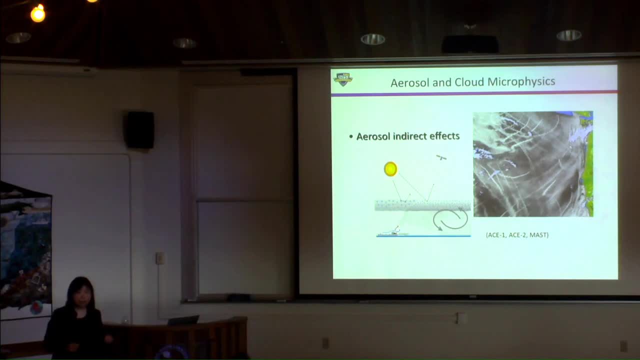 So, as a result, you generate lots of little cloud droplets, but then the amount of water vapor is about the same, So you have lots of them competing for the same amount of water vapor. So, as a result, you have the cloud droplets. 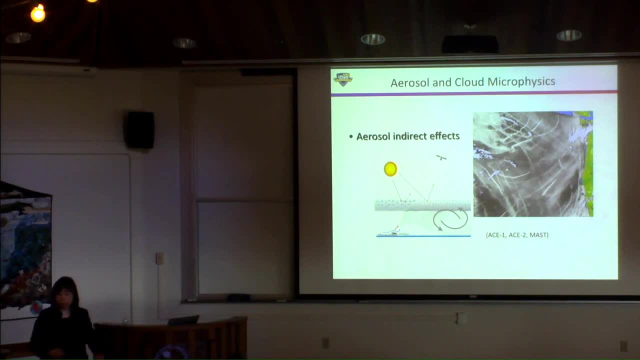 you know, are smaller when you have lots of aerosol. So what happens is- you know so- when they're smaller and then they're more reflective. So that's why you see all these ship tracks, So you can imagine, you know. 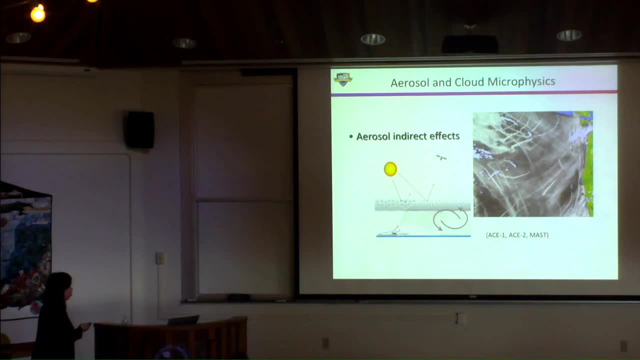 how this can be used by the Navy. Now, one of my colleagues, you know, working on satellite remote sensing and he has some clarified research and basically to figure out, you know, from measurement of these ship plumes, what they call ship track, 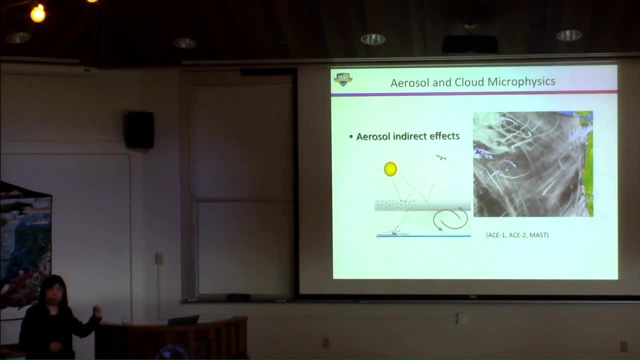 and so they can try to figure out. you know what kind of aerosol and the amount of aerosol and they figure out what kind of fuel and you know the aerosol that generate those type of aerosol and they can figure out. 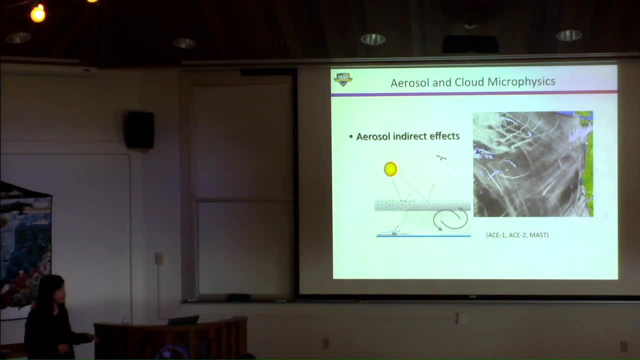 what type of ship is under there. And so now, because you know when you have the cloud cover, and then all your surveillance, you know, cannot go through the cloud in the visible part, and then you have to figure out something. 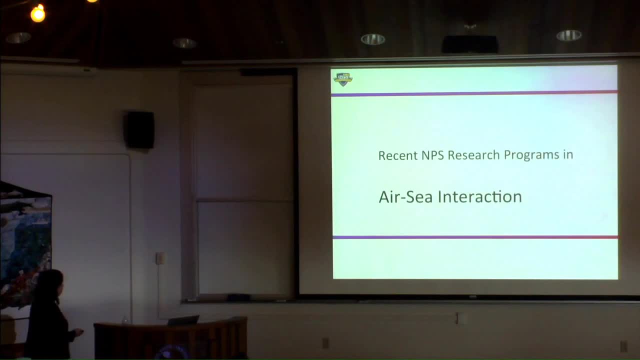 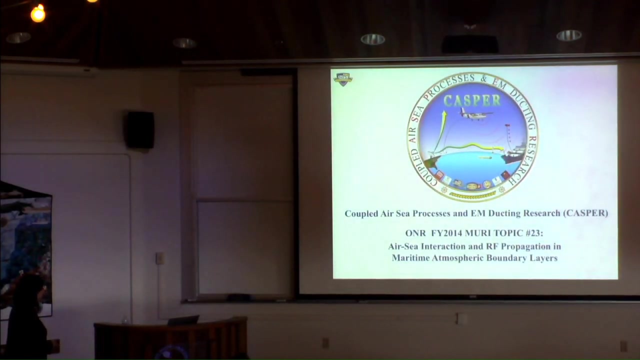 you know in that. So that's very interesting. So now those. so much for the basics of boundary layer and surface layer air-sea interaction. So I want to introduce my recent research programs in air-sea interaction. Now this one many of you probably heard about. 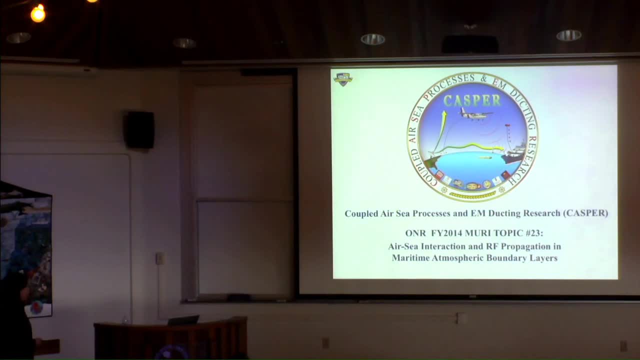 and this is Office of Naval Research MURI program. It's a multi-disciplinary university research initiative, MURI, and so I put in a proposal with six, five other university PIs together. It's a group proposal and we were lucky to get funded. 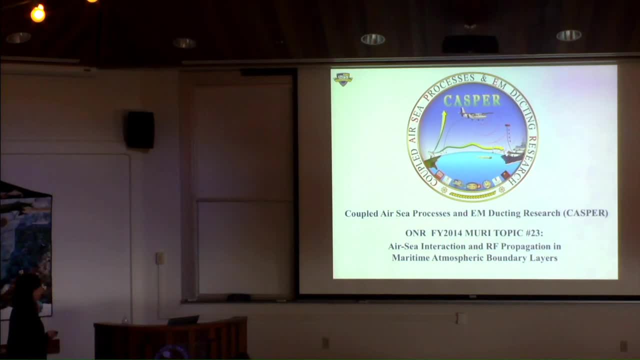 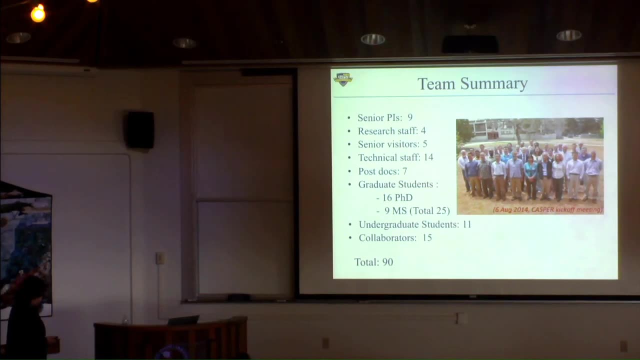 and this is called the Coupled Air-Sea Processes and EM Ducting Research, or CASPER, And so, and then this is a five-year project And so this has, you know, lots of collaborators and including PIs from different universities. 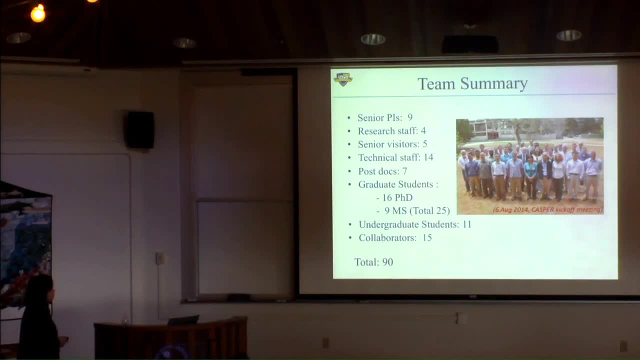 and postdocs and graduate students, and we keep getting collaborators, you know, because lots of people are interested, And so it grow to about 90 people. This is a slide I borrowed from the recent review at ONR, So it's very multi-disciplinary. 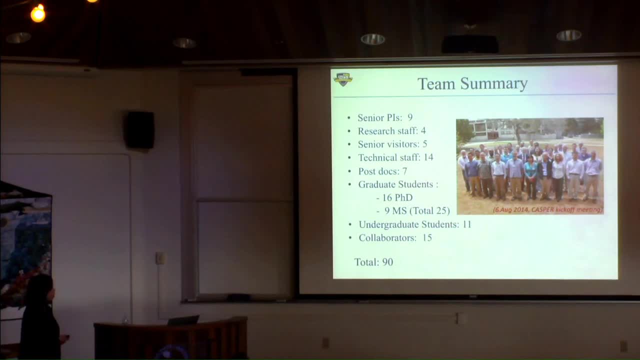 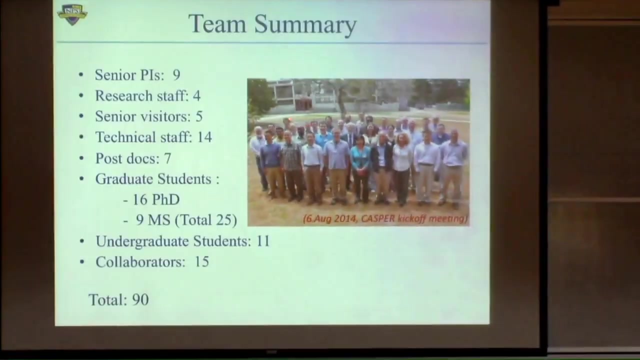 because I have people from the oceanographer and this is mechanical engineer. and I have people- this is mechanical engineering, and there is a civil engineer, this guy from civil engineering, and then there is some government double E here and this is oceanographer. 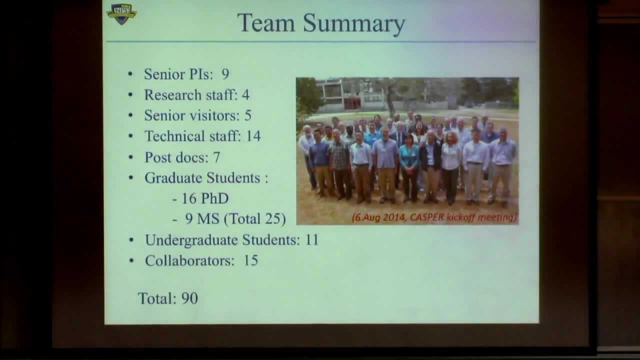 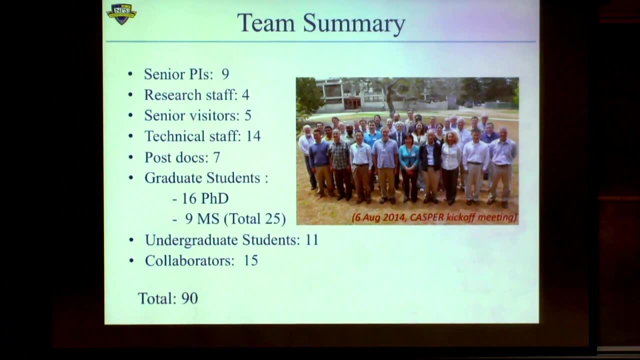 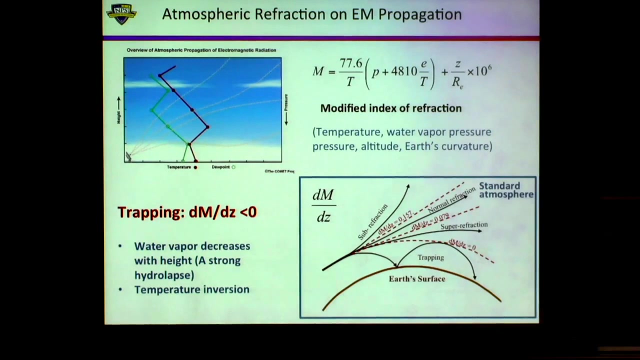 and, geez, not too many meteorologists here. I just realized that. So, anyway, it's a very truly multi-disciplinary team here, And some of those are my students there. So now, what are we dealing with? So we talk about gradients in the atmosphere. 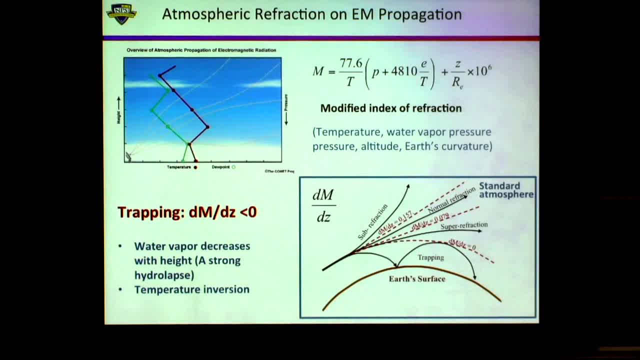 in temperature and humidity Now. so this project has to do with when you have a radar and you want to send the beams to whatever you want to detect, but you may not get there. And why? Because you know the atmosphere is in the way. 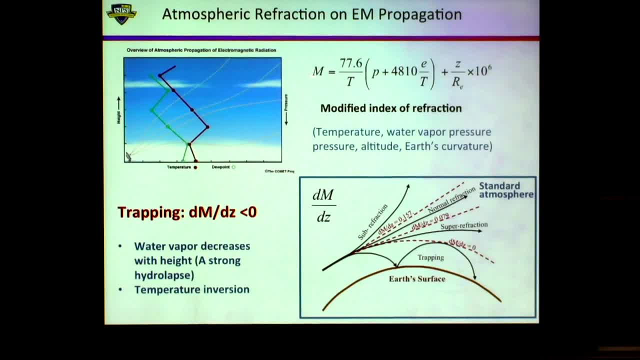 Now, when is it in the way? And it's quantified by this quantity called modified index of refraction, And you can see it has to do with the pressure and it has to do with temperature and this E is the water vapor pressure. 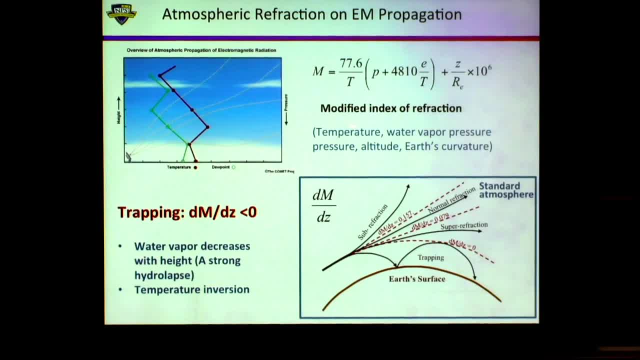 It's the amount of water vapor, And there are different regimes, and some of them we're less concerned, some of them we're more concerned. So think about this: This is the Earth's surface And so, in this situation, when the DMDZ, the vertical gradient- 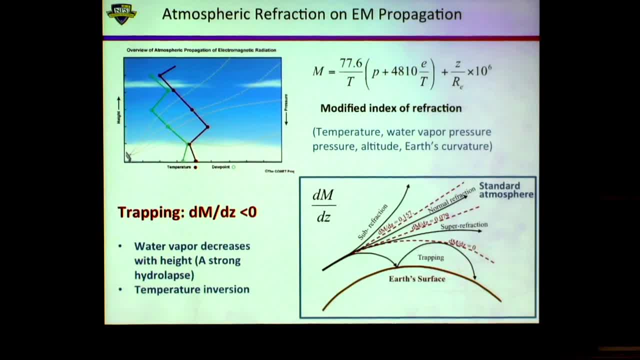 of this modified index of refraction is less than zero, so the beam comes out and is going to bend towards the Earth Now. so you see, this term has you know the Earth's radius index. It's here so we can see it easily. 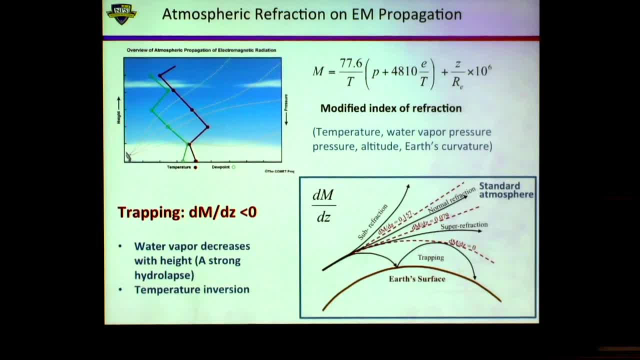 So this quantity, it bends towards the Earth. That means trapping, So it's going to come to the surface, bounce by the trapping surface and then go again. So this means you send the beam from here and you can see this. 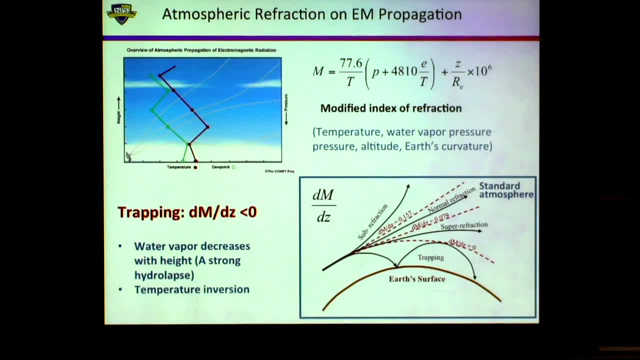 you can hear this from way. you know long, long distance. you know from here And so you know way beyond the line of sight. Now, in other situations you have, you know, send the beam. it's going that way. 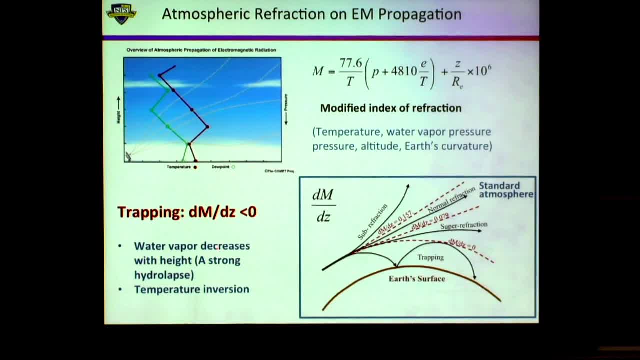 and this is for the standard atmosphere Now. so what's important here is: you want to find this trapping layer. where dm dz is less than zero, The gradient is negative. Now, in this whole formulation, the gradient is very sensitive to the water vapor. 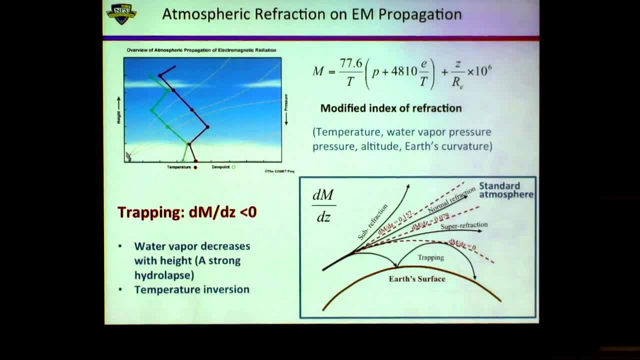 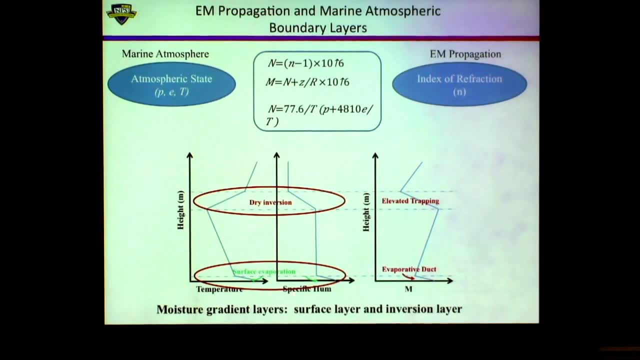 so we really need to nail down the water vapor amount, And so now you can see where do we have the gradient in the boundary line. One is near the surface and this one is labeled right, so they should go this way. 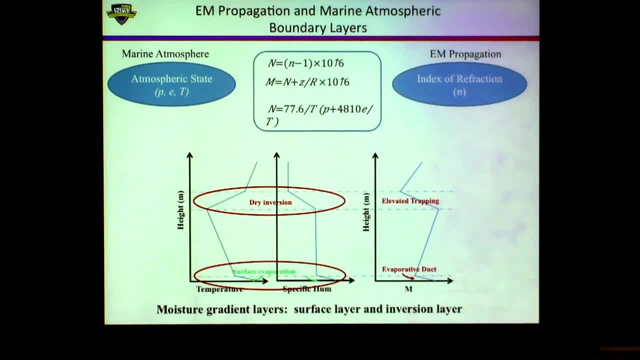 Okay, So you know, this is where we have the basic humidity and temperature, And then also at the top of the boundary line, because now you need to move to the dry atmosphere and the warm atmosphere. so you have the gradient. 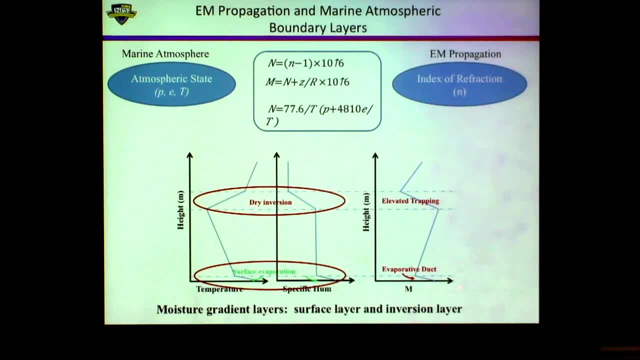 So this is where you know, we normally have a duct and then we call it the evaporation duct And this is another layer with the negative gradient and we call this the elevated duct. So moisture gradient is the most important. 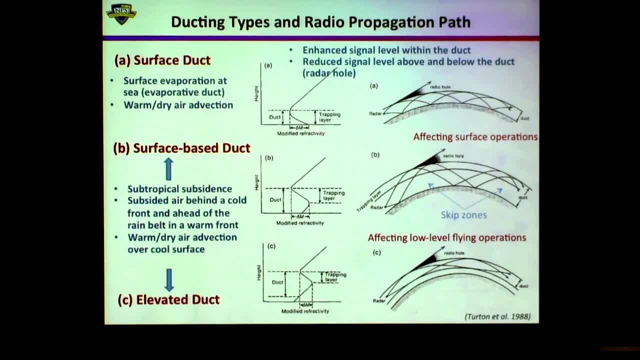 And this is a picture about the surface. different type of duct and this is the surface duct. you know. so the trapping layer is at the surface. So if your radar is here, okay, and then you know from far away. 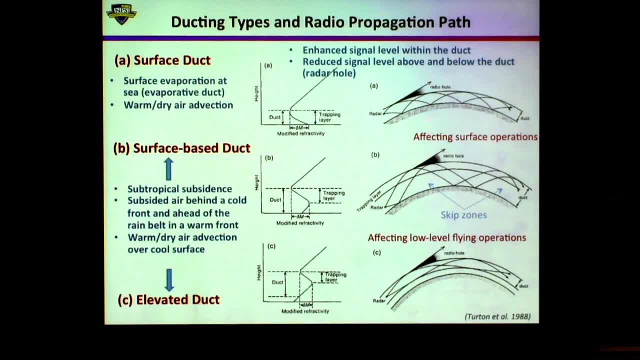 and you can still hear the. you know the signal, you can get the signal, but if you have a low flyer that's just above this layer, and then you wouldn't be able to hear it. Okay, So my student was telling me: 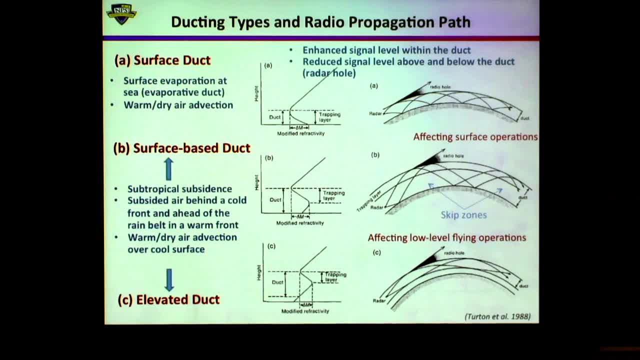 you know the stories about them on the ship, so they were trying to. you know they can hear the other ship, but then there is, you know, a UAV there. they couldn't hear it And the commander of the ship. 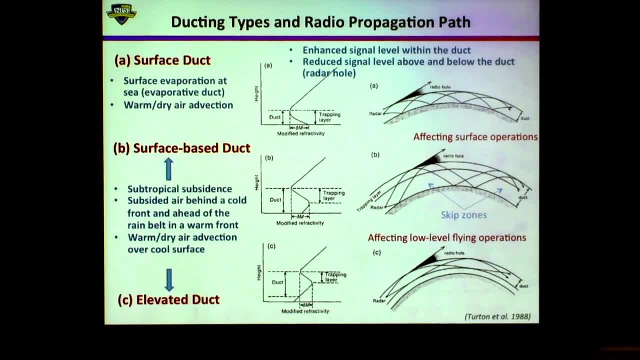 was really mad, said: what are you telling me? You know I can't hear them. and how come I can't hear this guy? And so they pull out this, and this is why. So, and now, in the situation like this, 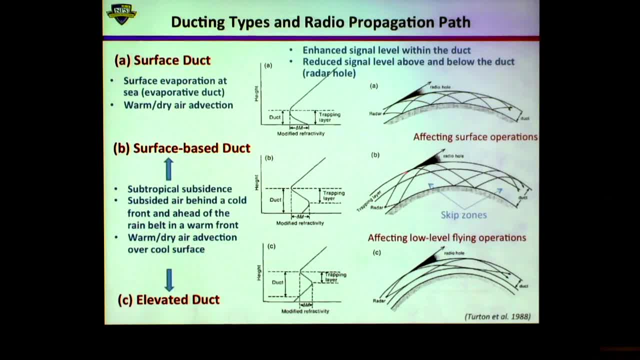 it's a surface-based duct Now. you can see the trapping layers here Now. so there are regions at the surface you have concentrated energy, and there are regions there's none. So there are lots of spatial variability in this. So you would not. 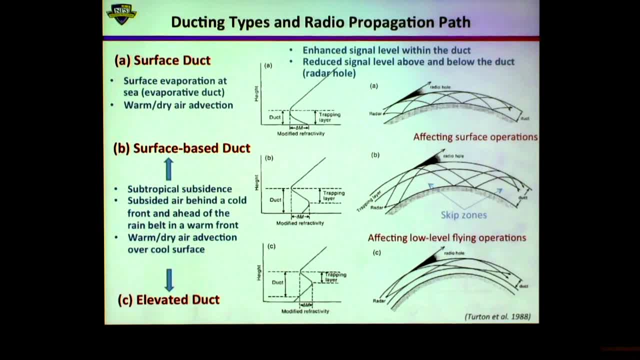 this is what they call the skip zone, And now, if you have this totally elevated duct, and then if you have, if you are inside here and again, you can hear, you know from far away or be heard from far away. 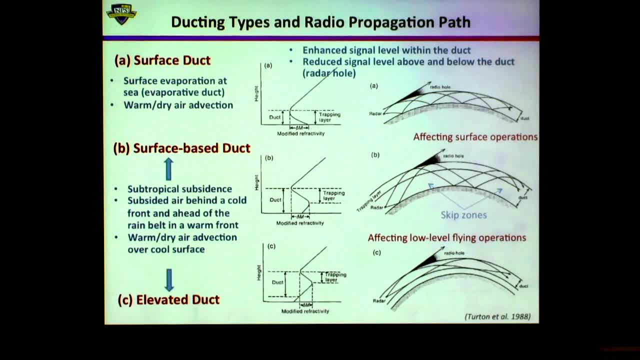 or you know, and if you are here and you are in that radio hole, So that's why the Navy is interested. And this also has the commercial implication too. you know, because you know all the communications nowadays. 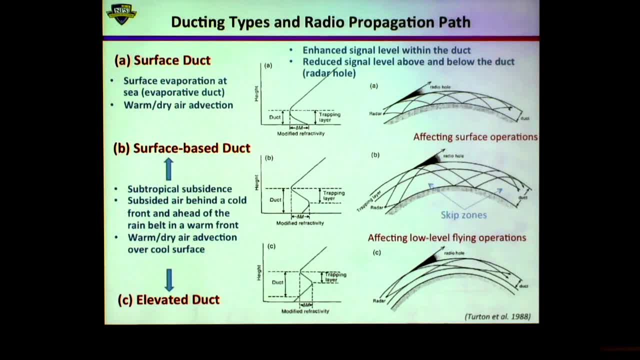 And the Navy. now you know why they fund this project? Because nowadays, everything it depends on what they call the EM spectra. Okay, And so what? everything is communication, And they don't do anything. you know not too much. 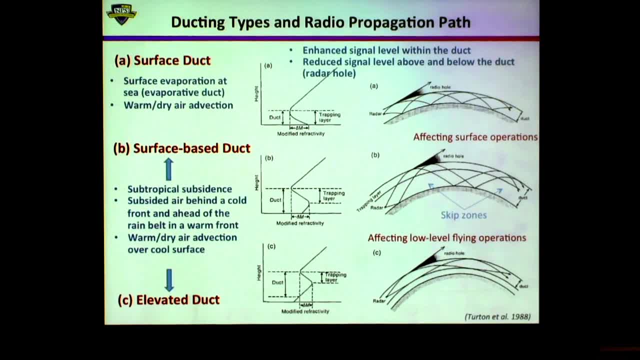 on the ship locally. So everything it depends on communication. So if you want to kill the enemy, you know the first thing you do is to kill their communication. So there are lots of engineering in these. You know. we are just. 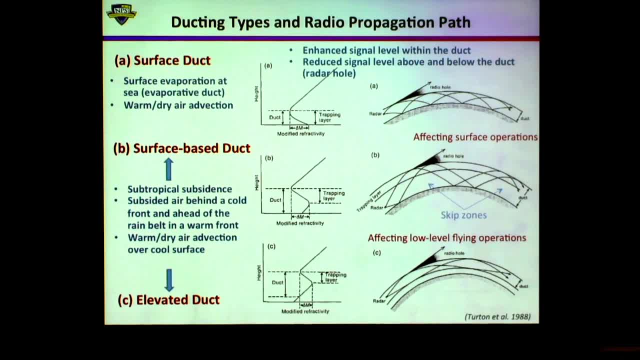 understanding environment. See, you know we are kind of passive. Understand the environment, see how they affect the Navy operation. But there are also other side of the research and they try to like a jam, you know. So they create some false signals. 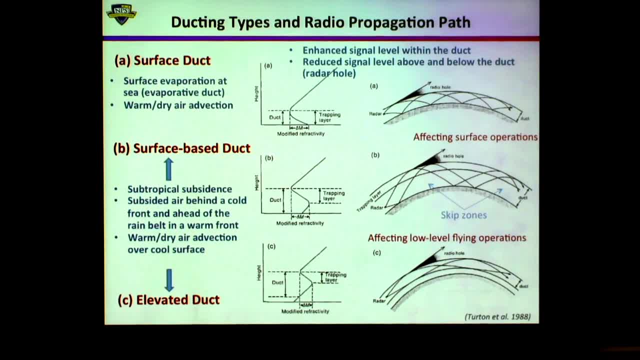 And, you know, like using a swarm of UAVs or, you know, wave gliders. So, and if you know, so send out EM signal from there, So the enemy may think, oh, the signal you know. 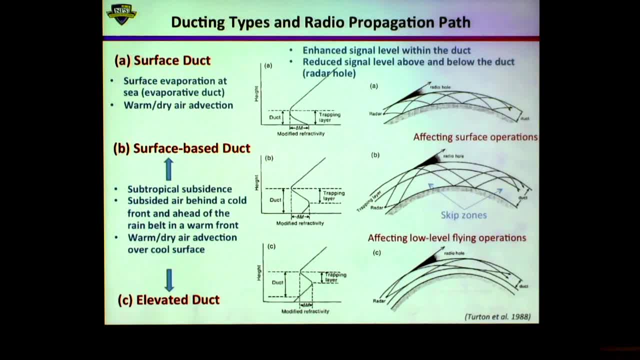 the fleet is right there, But it's actually a thousand kilometers away, And they can also jam and send different false signals. So there are lots of things that I don't really understand in there. Now, this is not a new issue. 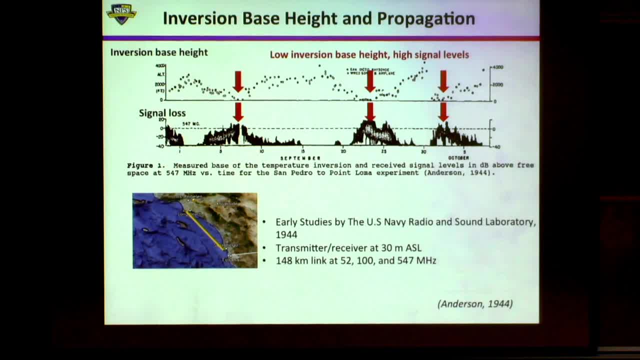 You know, back in 1944, and you can see here, and then they notice. you know, when they look into the beam. you know the propagation here, measure the propagation. they notice, you know, when you have very low. 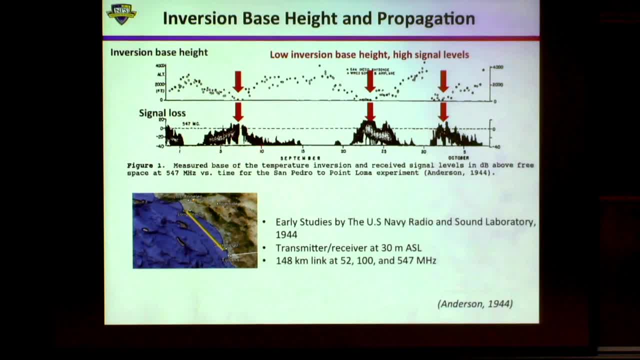 inversion height. that's where that trapping layer is low And then they can get high signal. So you see this very nice correlation. This was back in 1944. So in the old days, you know, this has been an old Navy issue. 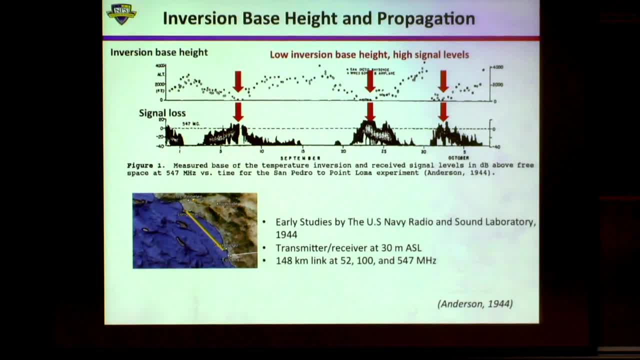 And but nowadays, because this has so much you know underneath you know, has so much of the air-sea interaction component to it, in the Bay Area we can't really do any basic research. So this now has become: 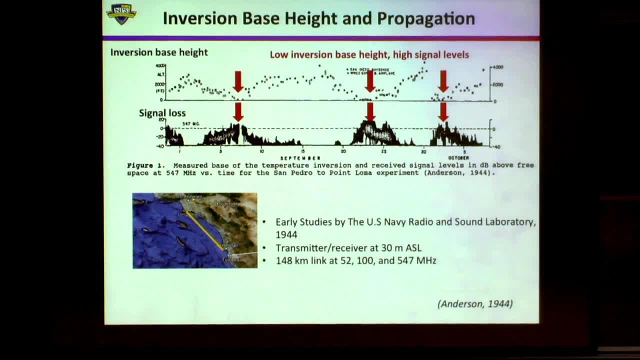 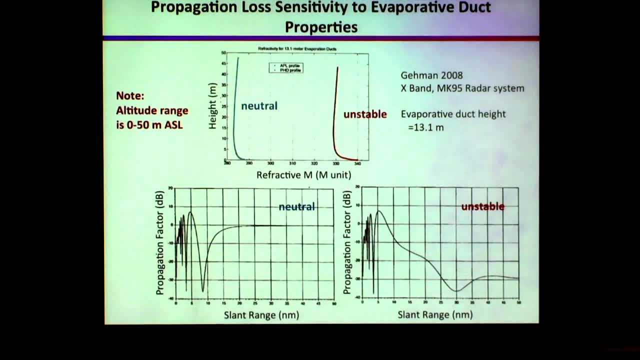 like a meteorology community and we are interested in this. So not just the Navy presence And this is a very subtle thing. You know, it's a difficult problem, As you can see here now I have like two profiles. 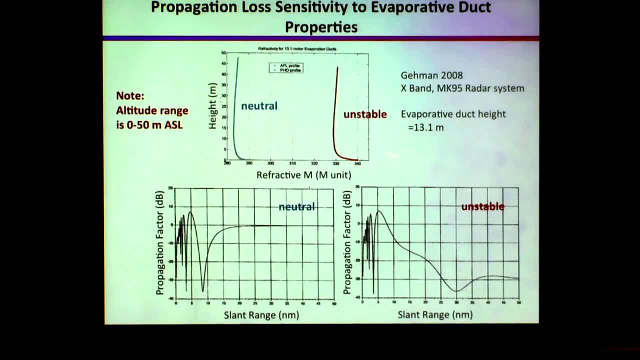 of the M profile, the M, And so now these two give the same, the so-called evaporation duct height, but their shape are a little bit different. But then you can see. now this is the propagation factor, And think about this. 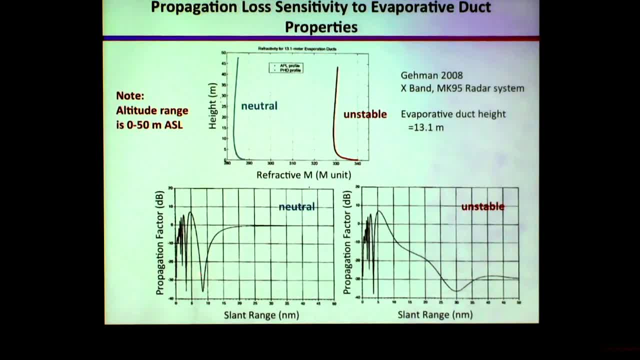 as propagation loss. You know, the lower it is, there's more loss. So you can see how different these two are. You know so, but the if you just eyeball these two profiles, they're not that different. 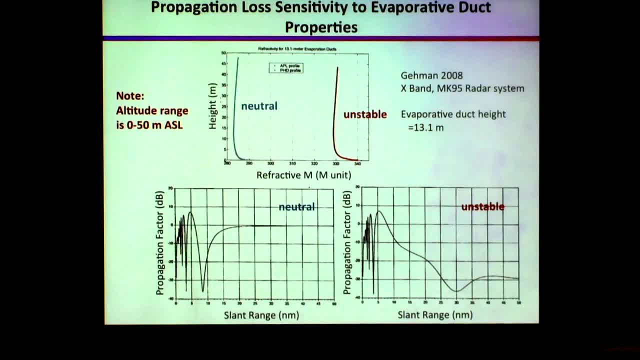 So this is the, you know, a subtle variation. It makes a big difference in the propagation, And so that's what makes it interesting, as also what makes it, you know, very important. you know, and very hard to do, 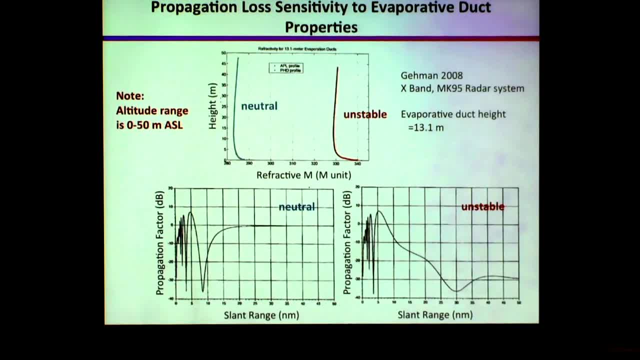 So that's why I'm being trying to use the small bows to get to the close to the surface and without any flow distortion by the ships. Okay, I don't like the big bows because you know there is a boat. 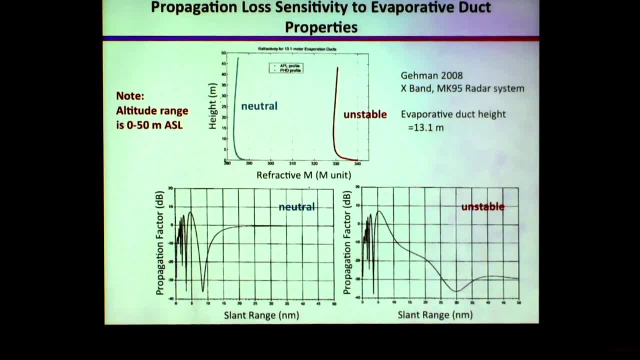 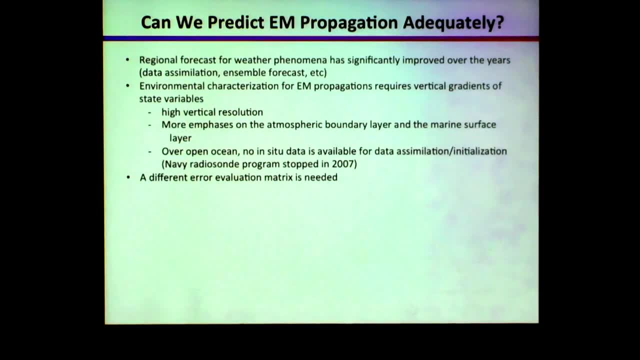 in the way And so they disrupt the very atmosphere that I want to measure. So the small boat, you know, works magic on that. So now the question is: can we predict that accurately Now in the past? 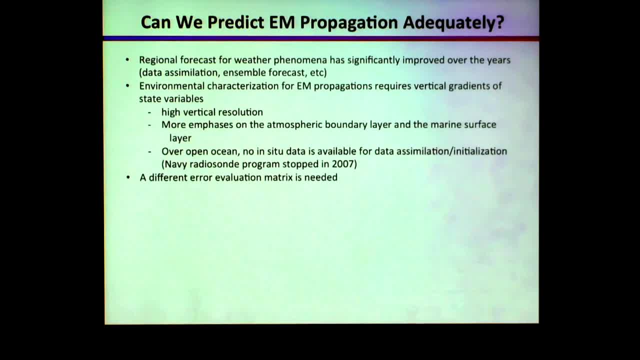 we're. you know, forecasting is more on the sensible weather. you know temperature, humidity, wind, precipitation, And so the grid scale that I mentioned is kilometer range. But all these, what I'm working with, you know, are the very small scale. 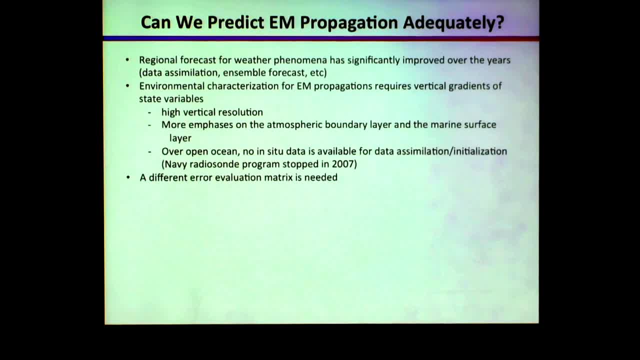 Okay. so are we equipped to do that? You know, not really So. and even you know how we should evaluate the model performance. it's a different story, you know, because now we're looking in the gradient. 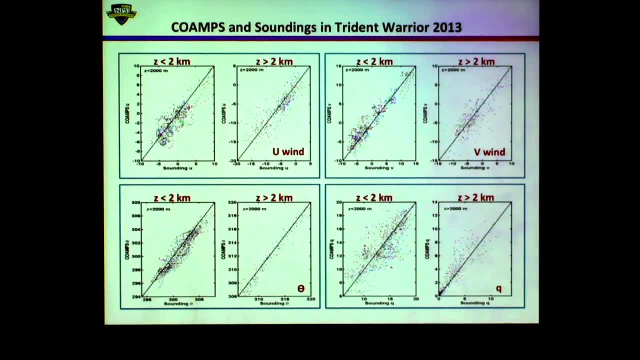 Just to give you a little feel of this, this is from one of my students. students' work, So when we do like, this is from the sounding, And so which is balloon sounding, and we get the data And this is. 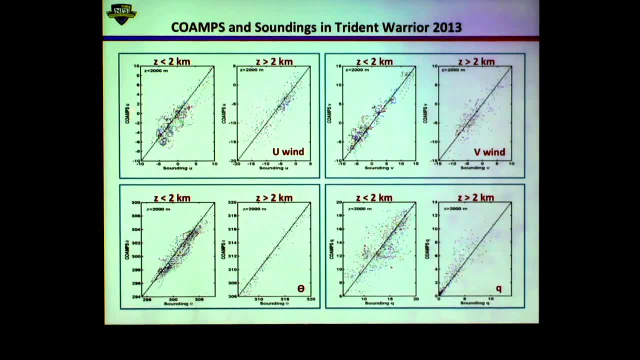 this is from the Navy's coupled model, the operational forecast, And you can see, you know nowadays, forecasting-wise we're doing a pretty good job. You know it's mostly on this one-on-one, you know around that. 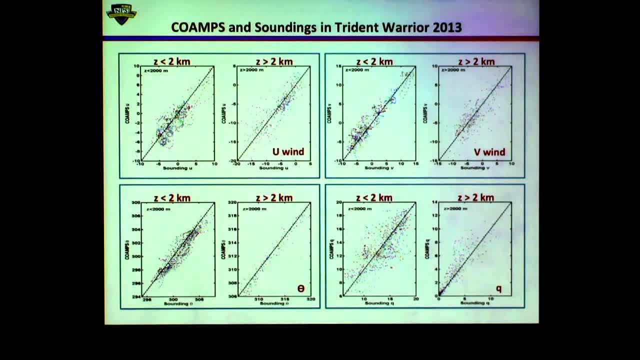 So statistically, it's a good job, And for a specific day it may be- you know- larger deviations, And so this is for. so think about this as temperature, as some other temperature that we normally use, And this is the amount. 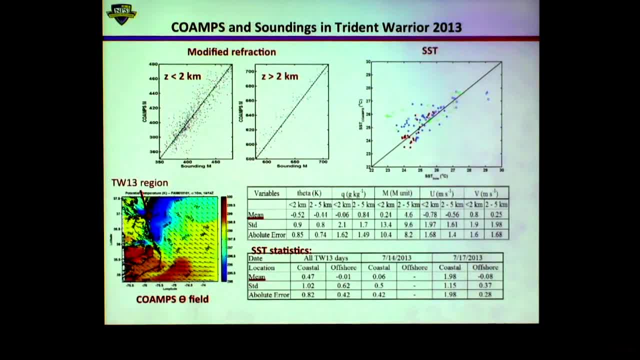 of water vapor and the wind. And then you look into the, that M quantity And if you look at just the M it's not too bad. Sea surface temperature, you know, is actually one of the most the hardest thing. 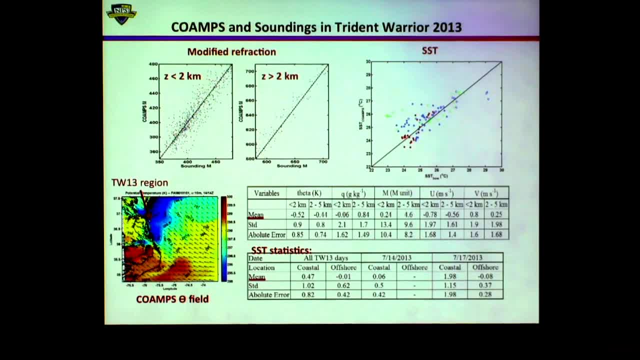 to get accurately And we've been struggling a lot with getting correct sea surface temperature. But you know, overall it's okay. So these are some mean statistics And for this particular project. And now if we are looking into the profiles, 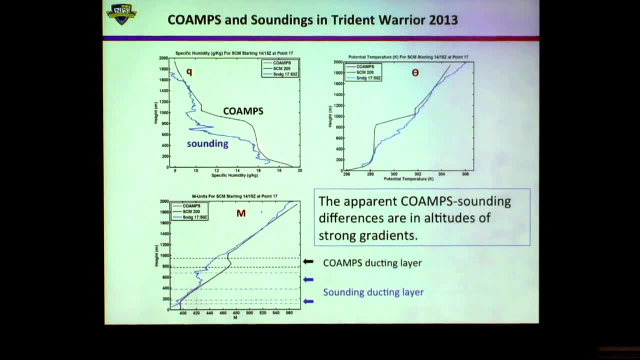 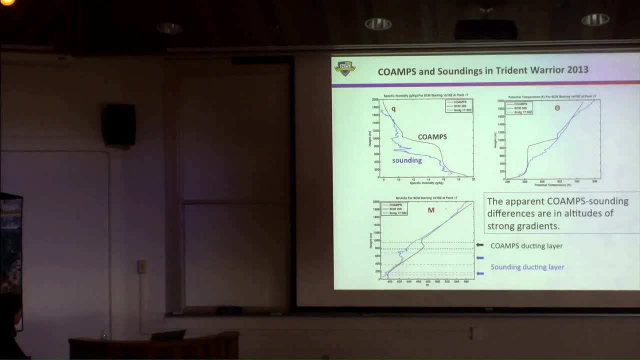 where we want to identify the ducting layer. So now you can see. this is what the model says. So you know. this is what the sounding says Now. so this is where that gradient is. And now, 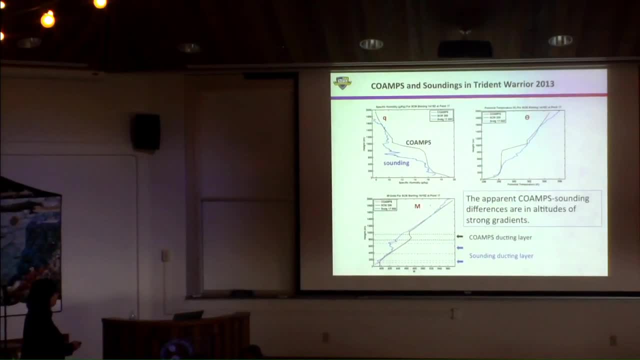 the sounding shows. you know, the measurement shows the gradient here Now. so you look at the M from the model And this is where you have that trapping layer, And from the observation you have two of them. This is one trapping layer. 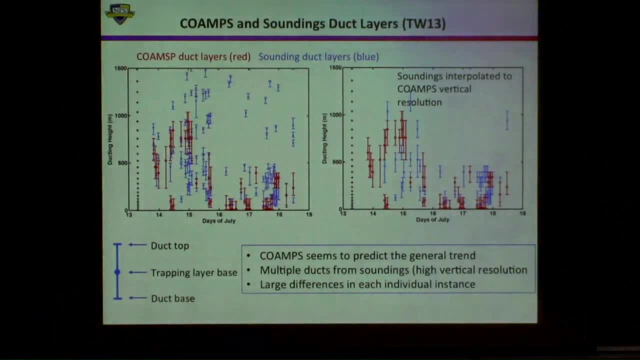 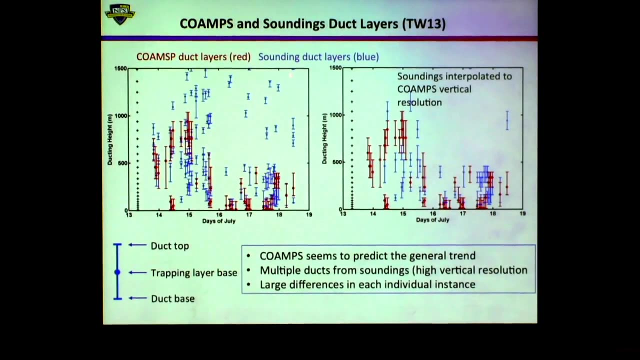 This is two trapping layer. So when you compare the trapping layers and the ducting layers Now, the blue is the observation, blue is the- I forgot you know- blue is the sounding and red is the observation. So now, 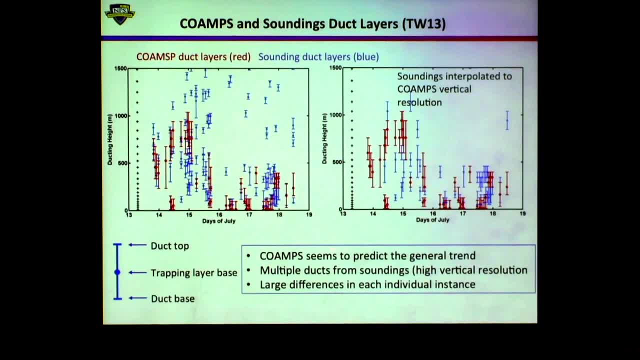 you can see the co-ed model And now you can see huge differences, you know, in the gradient, Because now we're looking into the gradient And then we can say: well, you know, your sounding has much higher. 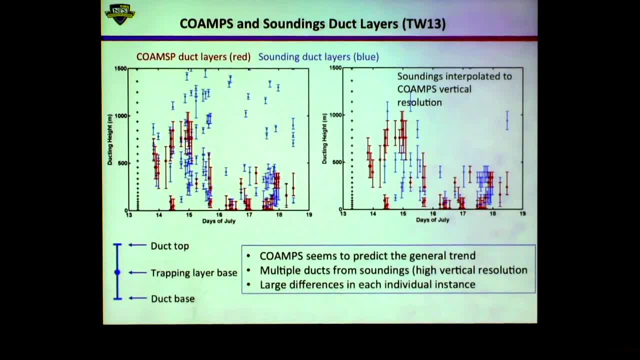 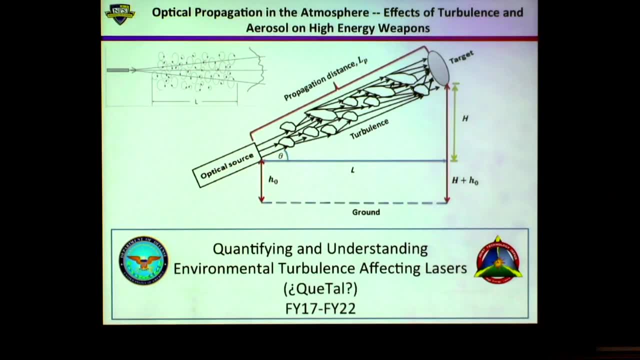 you know vertical resolution, So how about we sub-sample our sounding into the same resolution as the forecast model? You still see a significant large deviations there. So that means you know the forecasting is much higher, and that's the whole. 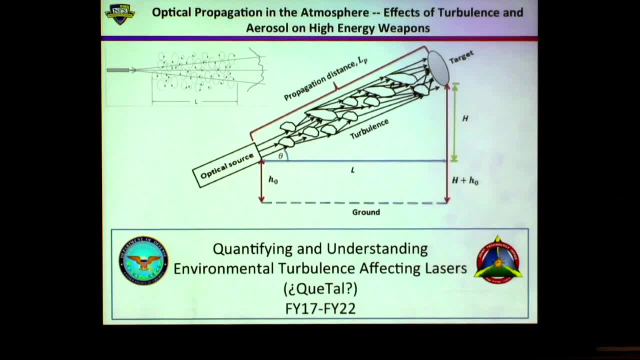 motivation behind. you know, supporting Casper. Now this is my new project that I just learned I'm funded, And so this has to do with the atmospheric effect on the propagation of the optical wavelengths. okay, much shorter wavelengths. 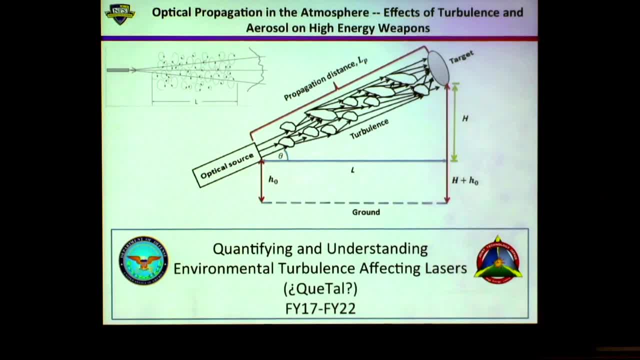 So the issue here? it has to do with the laser, you know. so you probably heard about high energy laser weapons. okay, So now you know, you can see that the laser is coming in here in there. 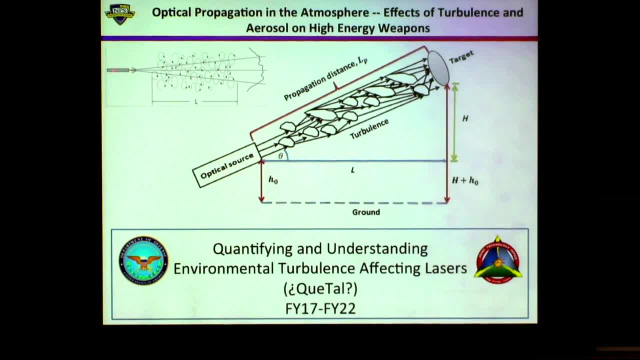 and so what's the? you know the boundary and that's turbulent. So when you have the turbulence, this is the perfect wave coming from the laser source and going through the atmosphere and you can see this distortion of the phase. 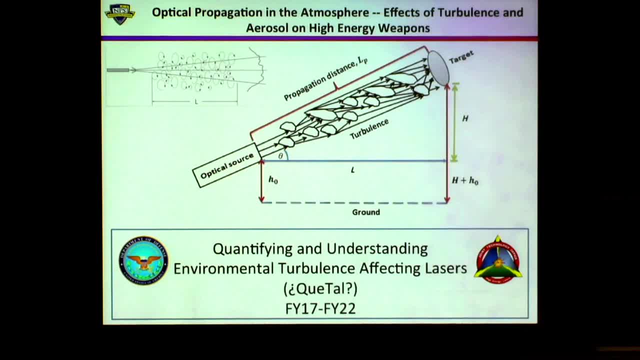 okay, Now what happens with this turbulence in between? now, when it gets to the target and it loses its focus, and there's also an issue- is going through the atmosphere and there is attenuation, okay, So this effect of the turbulence is called scintillation. 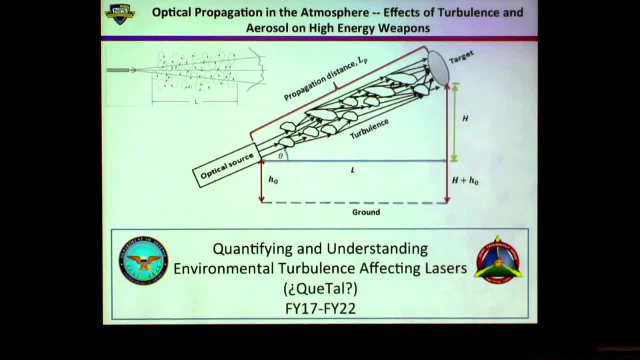 Now. so on a hot day, if you drive, you know, and then you can see the air in front of you, like you know. so that's the effect of scintillation, and this is more affected by the temperature. 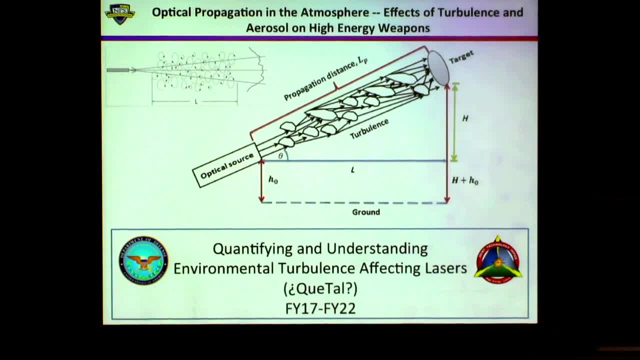 and you know, in turbulence, in the small scale turbulence range, Then the attenuation and then there's also scattering and there's also aerosol. okay, Normally now we consider the gas absorption for the solar radiation in the atmosphere. 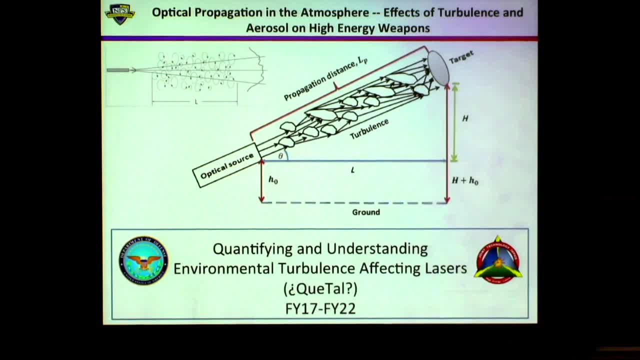 is pretty small. So, and you know, for some applications it's very important, but if you do the energy budget, you know that's pretty small. Now this is different. when you come, you have a laser source, because now 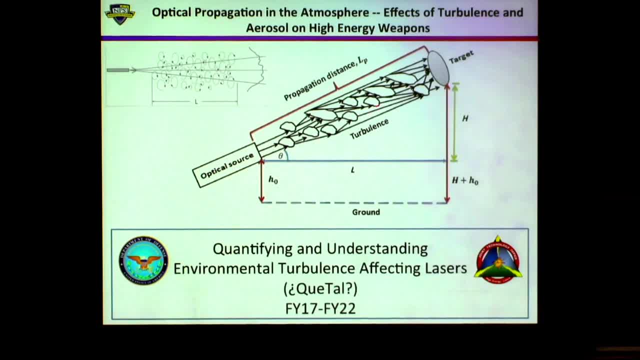 you have a huge source. So this absorption is going to be large and large, to the extent you know, to the atmosphere and generate local turbulence, and then these turbulence, will you know, go like this, and so what? downwind, and so 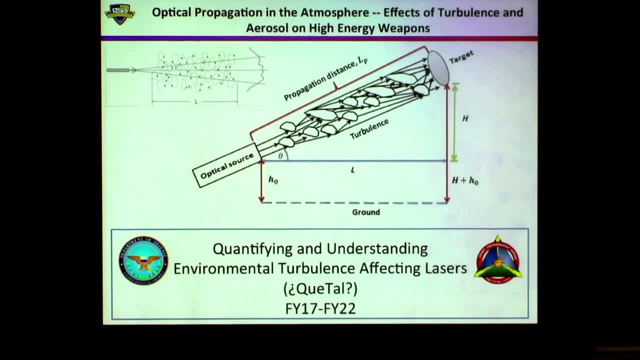 you will see this laser beam kind of deviate towards downwind and I learned that you know the first time. you know when I the first time I learned about that. it was very fascinating to me. you know it's called thermal blooming. 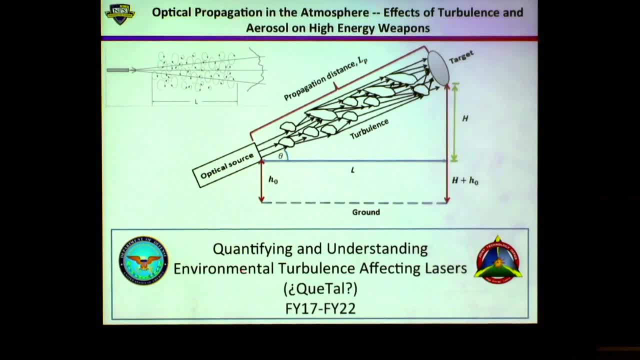 which I never thought about. So quantifying and understanding environmental turbulence affecting lasers. So one of my colleagues suggested: oh, you can make it into CATAL, and which means what's up. So I like, okay, you know. 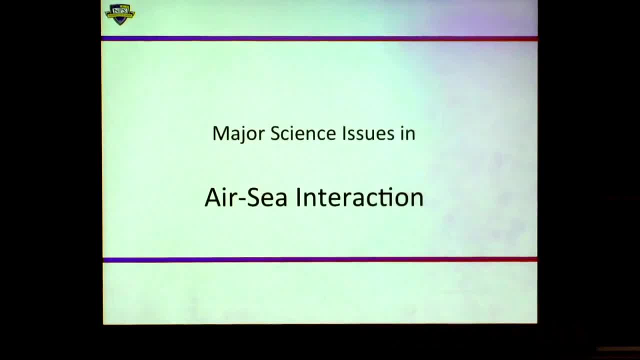 I wouldn't be able to come up with the fancy name, but you know, oh well, that's good and maybe that's the name that got me funded. So anyway, the first one is the. the ocean surface is not homogeneous. 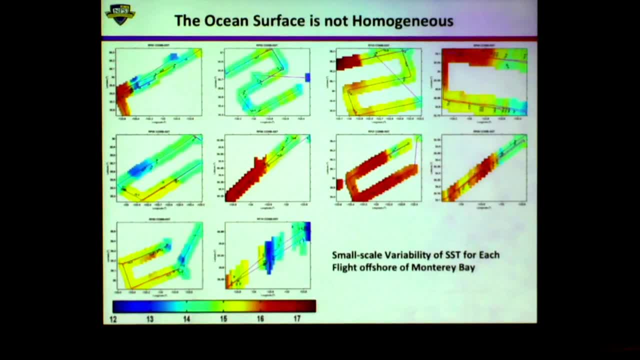 and so it appears homogeneous. okay, now so, but it's actually not, and this is from some aircraft measurement we did, you know, offshore here, and so you can see now, along the path we can measure the. 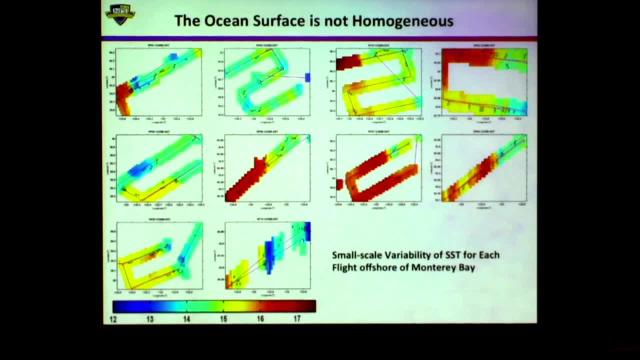 measure the sea surface temperature and you can see how much variation there is, and on a day-to-day basis. there is also lots of variation, okay, So now, why do we care about this? Well, the theory that we've been using again. 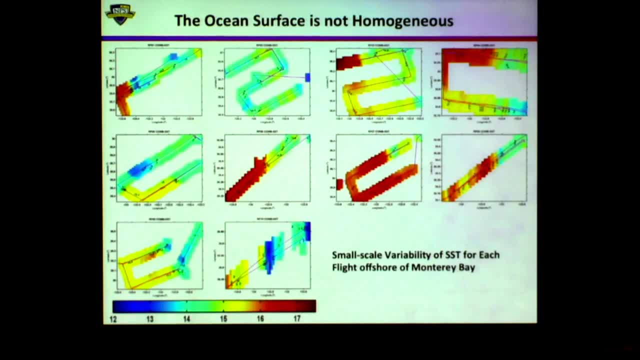 and again is called the Monning-Opko similarity theory, and you don't have to remember that, and it it's basic assumption is it's all horizontally homogeneous and so, but we don't know if you have a surface that's not homogeneous. 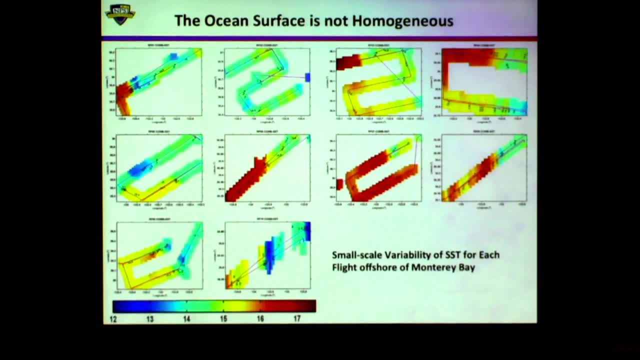 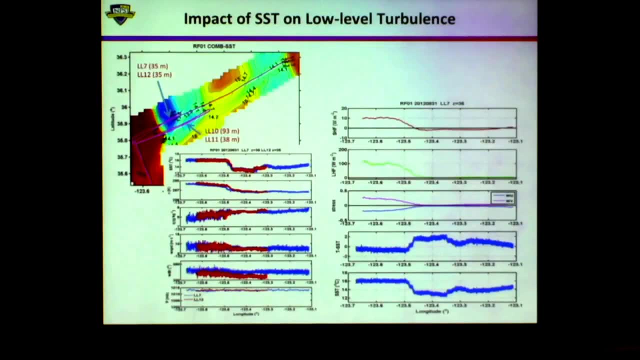 what's going to happen? and also, we don't know at what point this inhomogeneity will kick in and then become, you know, invalid. So these are all the questions that we don't know. So, when you have this gradient, 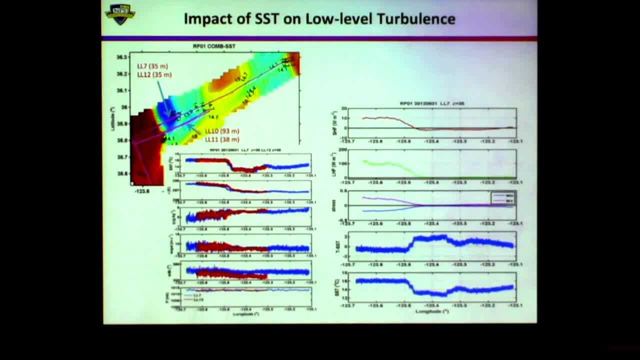 in temperature. okay, now this is the sea surface temperature. So you see there's a a sharp jump of 16 here, so this is like 13,, so 3 degree, and this is within a very short distance, and 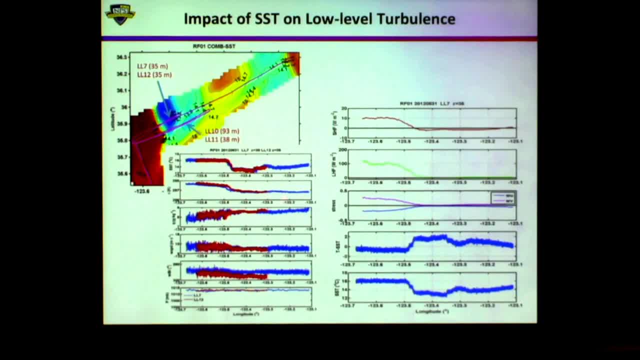 so you see it's turbulent here and you can see it's so obvious. and then it's less turbulent here. you know, when you get into the cold water region and if you look into the, the fluxes, you know the coupler. 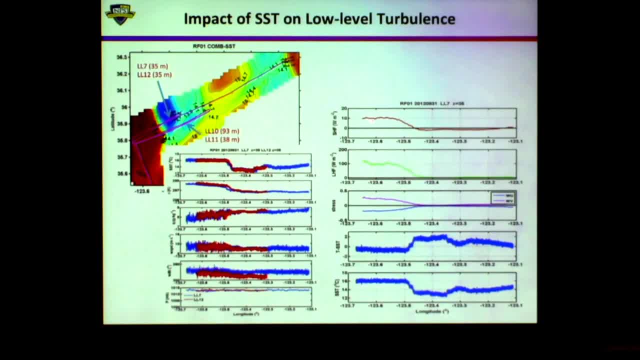 that I talk about. this is: this is sensible: heat flux: it's positive and 10, and now when you get to the other region, it's negative. So this means that you get heat from the ocean and here it means you input heat. 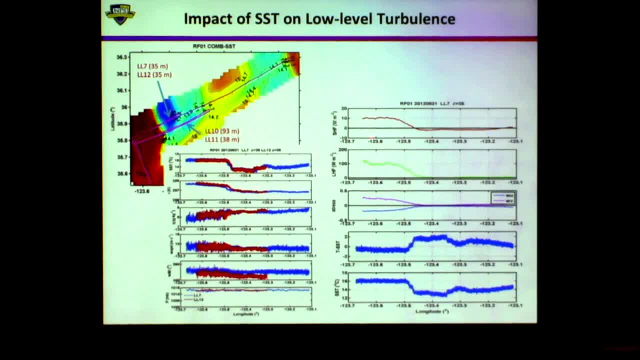 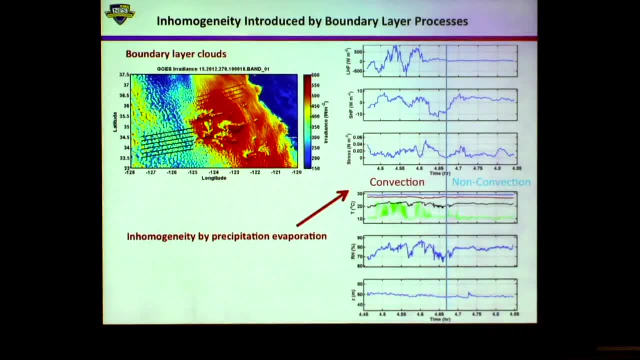 to the ocean. okay, So you, you are looking into very different air-sea interaction process around here, and so that's why we are interested Now: the cloud and everything that's happening in the atmosphere, like the boundary layer cloud. 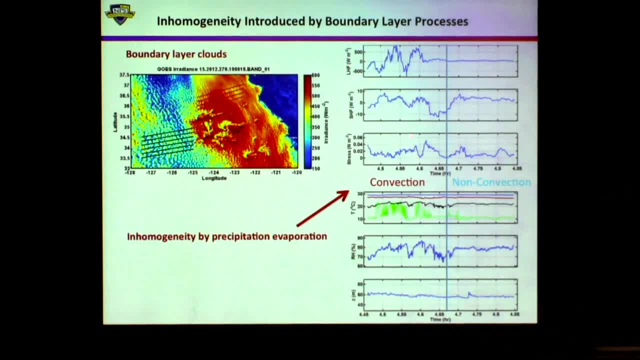 or precipitation, also have very, very high interfacial inhomogeneity as well. So you can see here- this is from one of the- the- the thesis study as well, you know. so the fluxes just varies, you know. 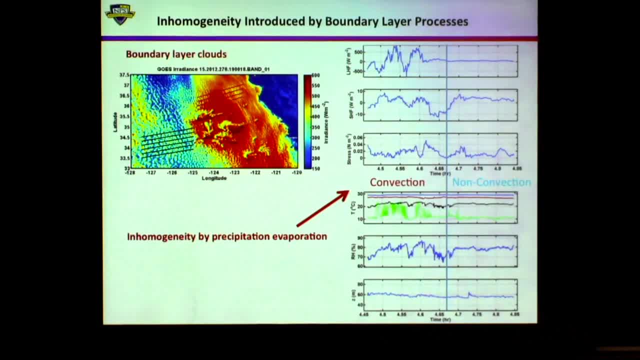 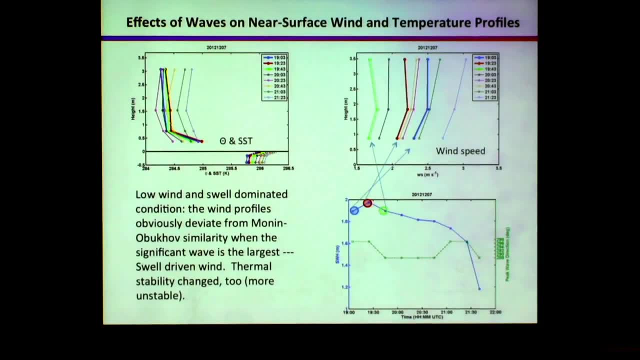 from this end, you know, to that end, and corresponding to these convection and no convection region, So atmospheric, atmospheric phenomenon itself, introduce the inhomogeneity in this and for this EM propagation. so now normally we say the wind is driving the waves, as 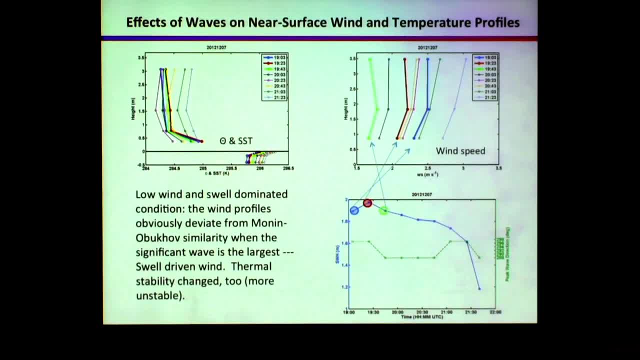 the wind wave right. so now, when we have very low wind and then we have strong swell, and that's the case, the swell is going to push the wind. that's when we have momentum coming from the ocean to the atmosphere. and now, if you look into the measurement from my small buoy now, in those situations, now the normally we 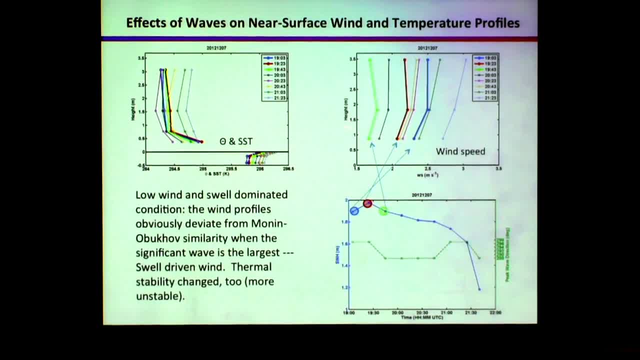 have like a wind speed increasing with height, but in these situation you can see the wind speed increase and then it decrease with height and the temperature gradient. you know it's very different here in these three situation. so we need to understand what are the effects of the waves and also that morning up of 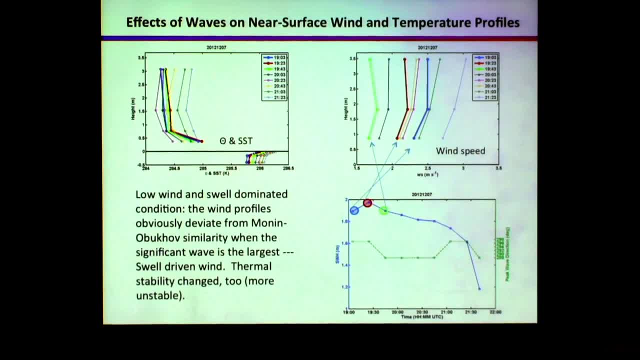 similarity theory and we call it most, and that theory and it was developed over land, there's no waves over land- and now we have a moving surface that is moving from the surface to the surface and it's moving from the surface to the surface, to the surface to the surface. so now we have a moving surface that's. 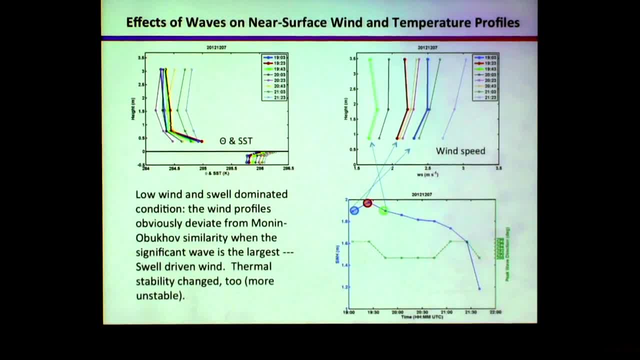 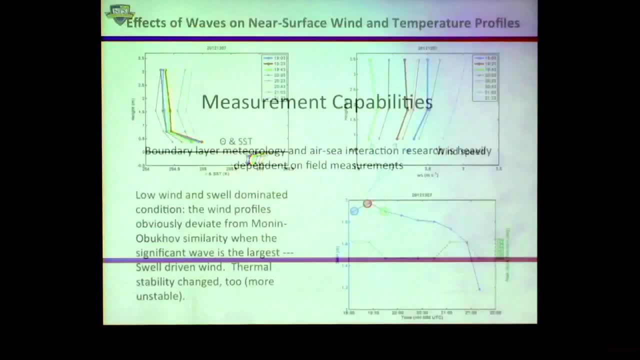 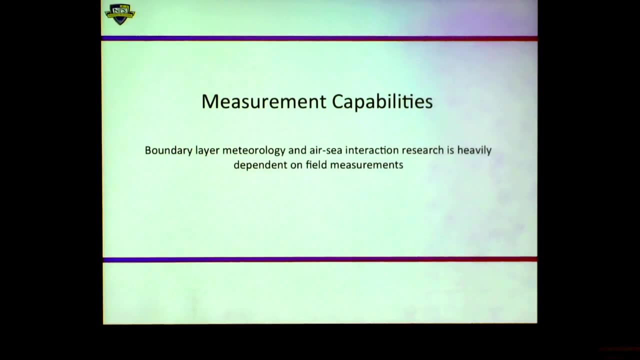 responsive to what's going on in the atmosphere. we're really talking about air-sea interaction. so when, then? what's the outcome of this interaction? how is it going to affect this profile? and these are the basic science question that we need to answer. and so the because of the stochastic nature of a 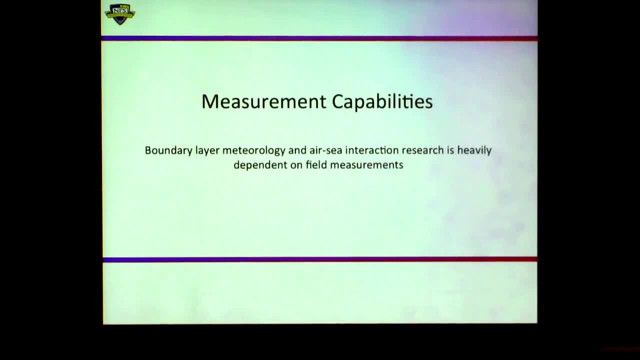 turbulence, and you know we don't have a theory, good theory, and it varies all the measurements, so what? that's why I'm out into the sea or on the airplane. you know I'm just traveling to do all kinds of field work and that's the nature of 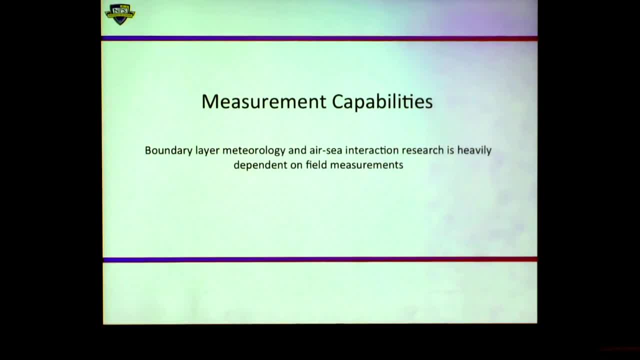 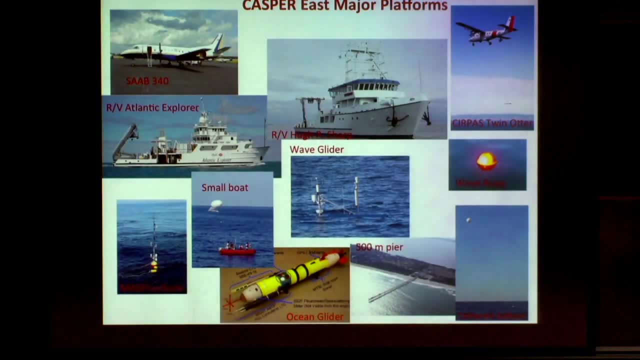 boundary research. so I want to talk about a little bit about measurement capability. now we use these different capabilities tailored to different, different field programs. this is what we use in Casper East platform. so now we have two airplanes now. this way, you can see, it has a drum, is fully instrumented. 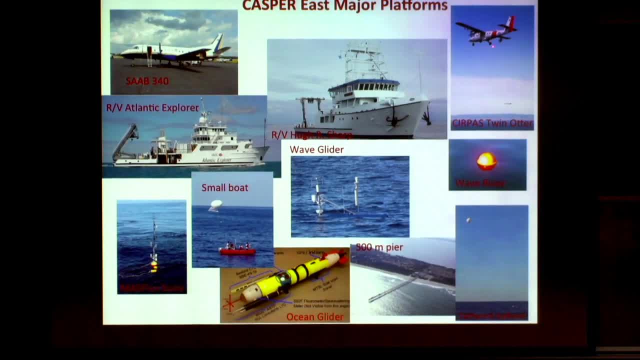 and so this is our measurement, and we can measure it, and we can measure it in the air, and we can measure it in the air. it is operated from off marina, here by the Center for interdisciplinary remote piloted aircraft study, Surpass, and so this drill is fully instrumented now. so this aircraft, the manned aircraft, the 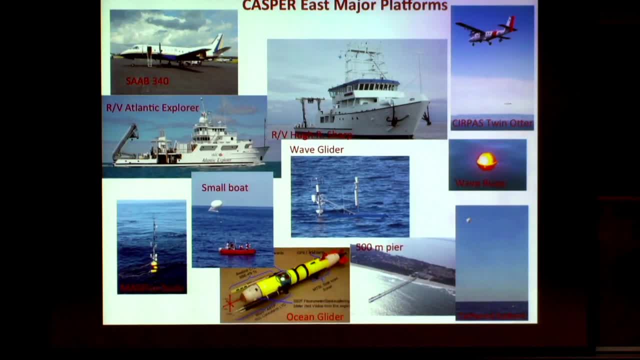 lowest level we can fly by. regulation is a hundred feet and we do that quite a lot, hundred feet. when you are on the airplane the first time, it's a bit scary, you know. all in a sudden you realize you can see fish. yeah so, but you know that's. 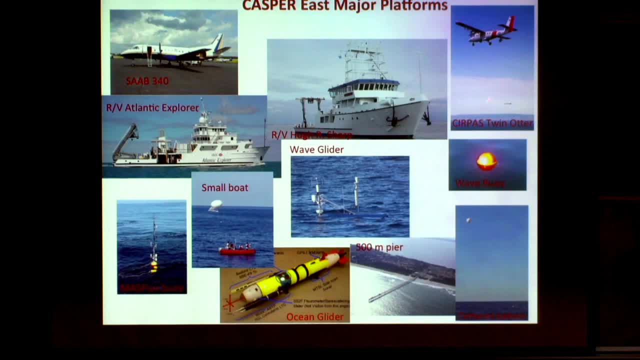 really low. And what do we do? So this drone was developed so it can be, you know, reeled up and down, And so we can. so we get measurements from two levels, or we can just use this to go up and down. 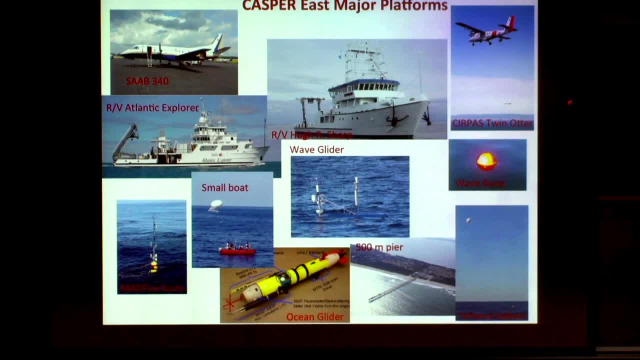 And this one can go up, to go down to 30 feet, which is 10 meter, which is so much better than 100 feet. So, and then this aircraft has lots of the remote sensing capability. It measures the surface waves, measures the surface temperature, and so it gives us a larger 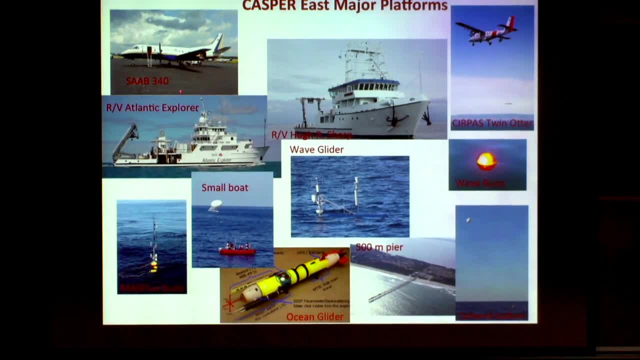 area survey of the ocean. And then we have two ships involved, And then we have all these small platforms, and so this is the ocean wave glider. I have another project working on instrumentation for the wave glider, And you recognize the small boat and tether balloons. 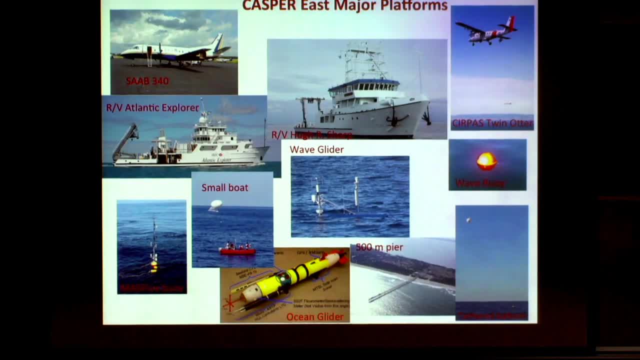 And then we have these small buoy. So you see, for these I'm going small. Why? Because I don't want flow distortion, you know, And I don't want the thermal heating effect by the platform itself. So we're going really small. 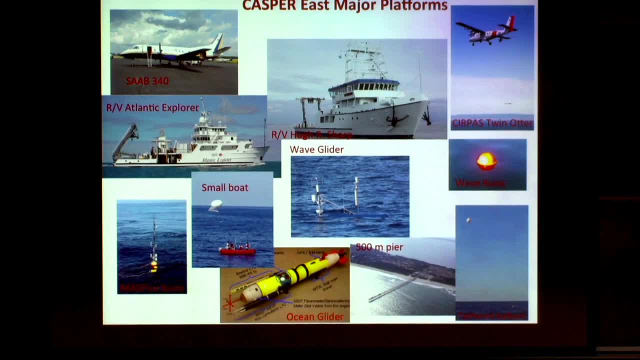 And this one when Alex and the folks doing it- I asked them to get the sounds you know all the way- to push it to the surface and then release it, because the lowest few meter is very important. That's where we have this sharp gradient. 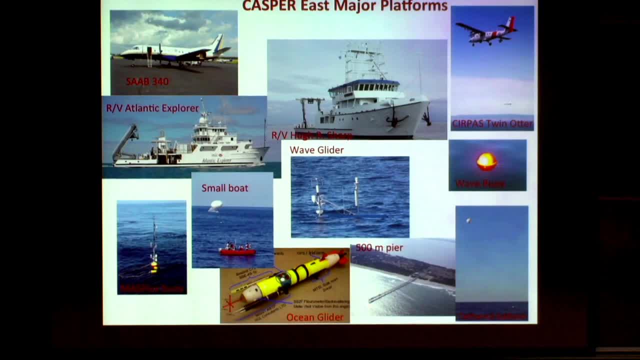 And so and there's, and we also use the pier, And this is a 500 meter pier. in at Duck, North Carolina, You can see the pier. It goes all the way in the water So and there are some underwater gliders. 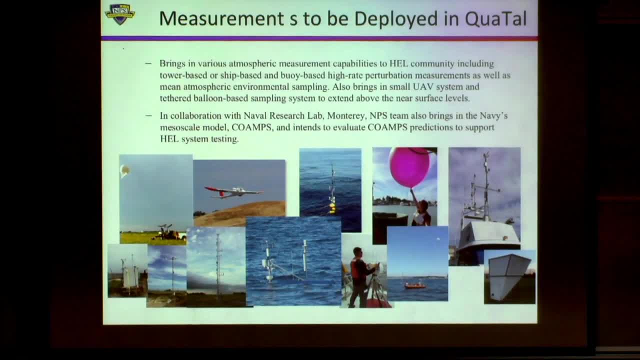 Now. so this is the you know in Quetel in this new project And now we are focusing on the optical turbulence. So we're using some land towers And we have two field camping we're going to do over the water one and another one over. 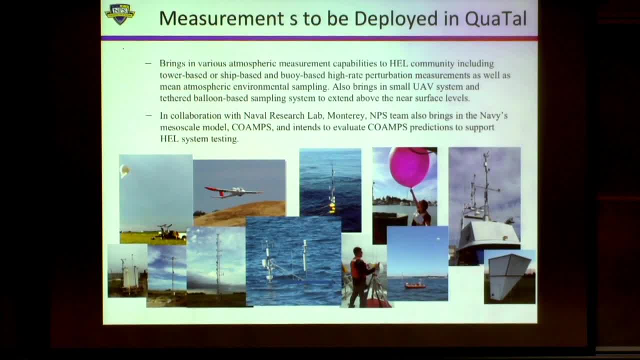 land. Oh, you recognize this is Holly doing the balloon launch from last year And so, And we would like to use the small balloon and the John Martin mast- you know, the ship mast for turbulence measurement, And so we have different levels of a mast. 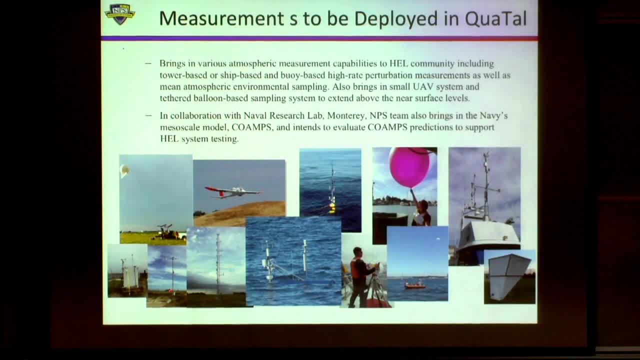 You know small ones and you see this- I believe this is the one at the aquaculture lab- And or the more beefy ones- you know this, go up to 50,, 52 feet. And then we have you know more, much larger tether balloon on this mooring system. 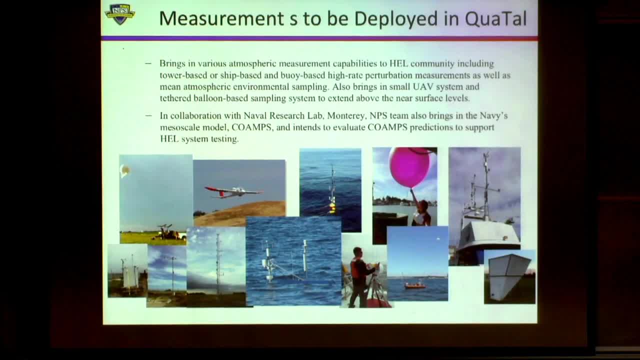 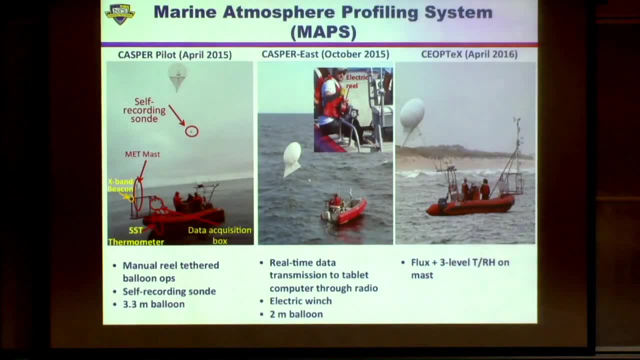 You know, there's a truck for it And this one we can go up to like a 500 meter, So it goes a lot higher, have a much larger payload And now so, and we try to develop, you know, measurement capabilities and, as needed, 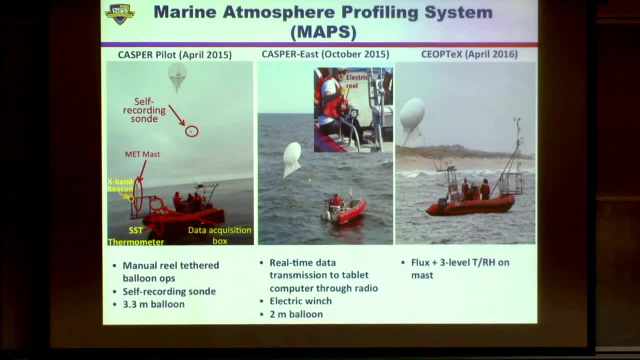 As you can see the evolution of this small boat. this is the John, this is the Mars landing rip. So, how we evolve from the initial, you know. so you know the initial concept in April 2015.. And then to 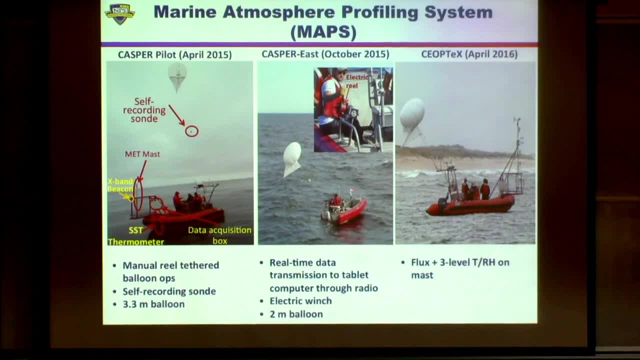 You know, October 2015.. And so here we have the manual reel, And then, you know, this mast is kind of a small, just proof of concept measurement. And then when we get to Casper East and we realize you know, this is lots of manual. 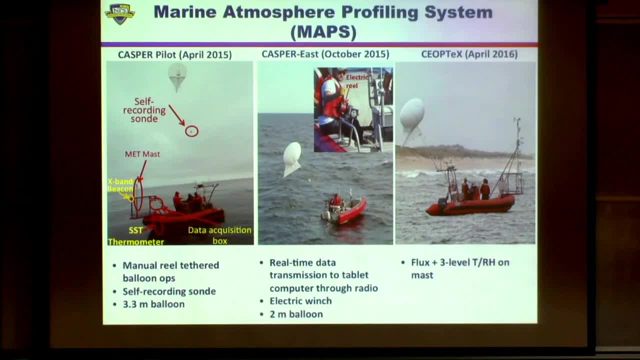 work, you know. so we really need manpower on that one. And then so we turn it into actually, Ryan, my instrument engineer, turn this into electric reel, And that makes it so much easier. And then we came back, you know, last year, and we need to do more. 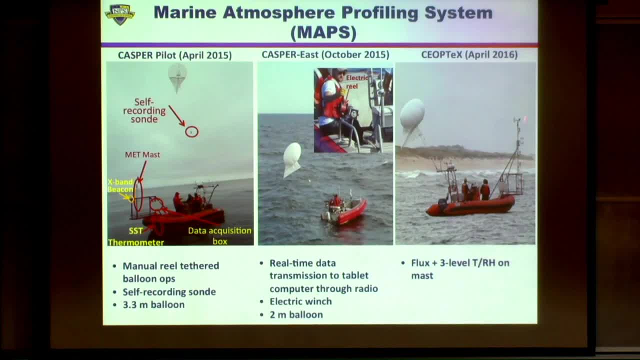 And we get back to the rip, and then you can see now this mast is much more hectic than our humble beginning at the early, you know, a year before. So this is how we are trying to perfect our measurement, you know, step by step. 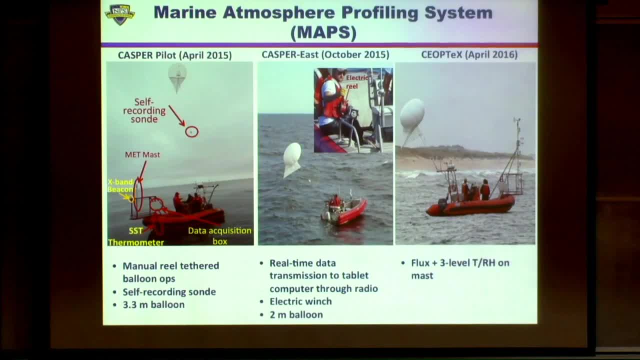 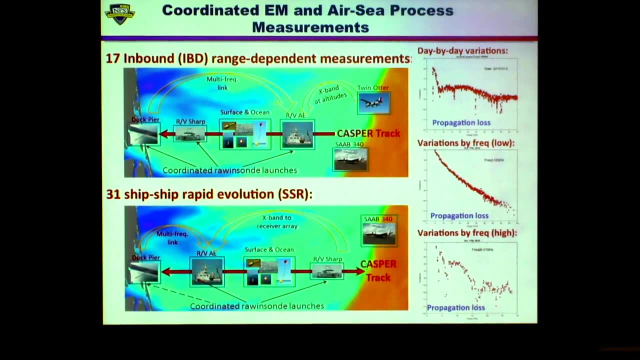 I think Alex knows every step of this. Yeah, Okay, So now in the field, program was all these different things, And then we need lots of coordination And we want coordinated measurement. So this is: you can see all the dance that I, you know all the this is our orchestra. 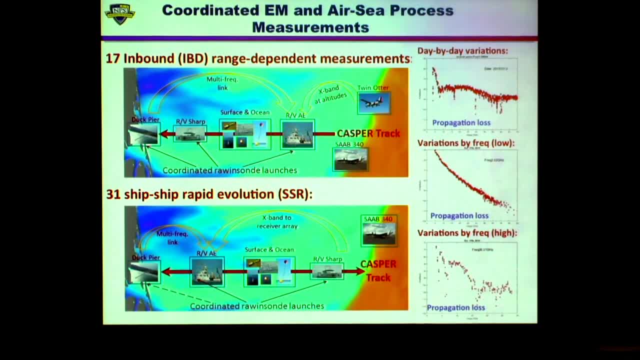 that we need to conduct during the field program. So we have multiple ships, you know when the ship is going, where, which direction, And so for the EM link measurement and the link between the ship and shore and ship and the aircraft, and this ship is in the middle doing the environmental measurement. 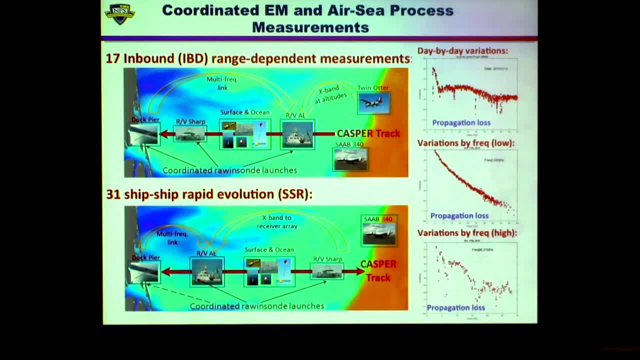 And also we have these coordinated radio sound launch And we see at certain time, and then boom, you know the shore, this ship and this ship were launching radio sound at the same time. That way we have the concurrent measurement, you know, of the atmosphere. 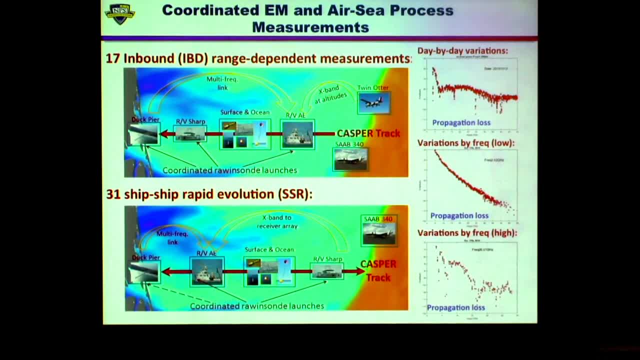 And this is a different type of evolution Now, and so this is a ship to ship And this one here. let me see if I can get this to play, does it? No? Okay, So this shows, you know, the propagation measurement is on the day to day. 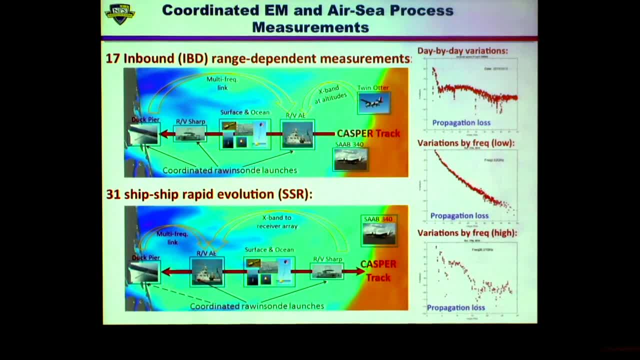 And this is supposed to be a video. It can go, like you know, from different frequencies, And this is for the lower frequency, This is higher frequency, So you can see what we did in collecting this EM signal. So the idea is we collect all these EM signal and we also collect the environmental measurement. 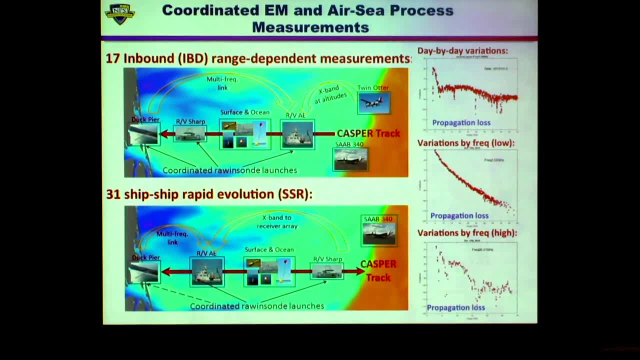 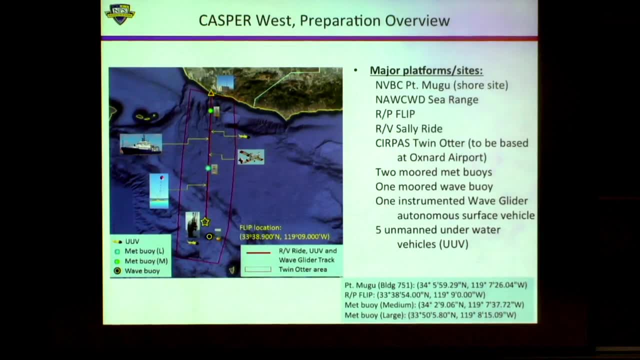 you know at the same time. So we know what's going on in the atmosphere that result in these EM signal And this is what's going to happen in Casper West And that's going to be offshore of Point Magoo, And so in this project we're going to have this guy. it's a flip, you know. 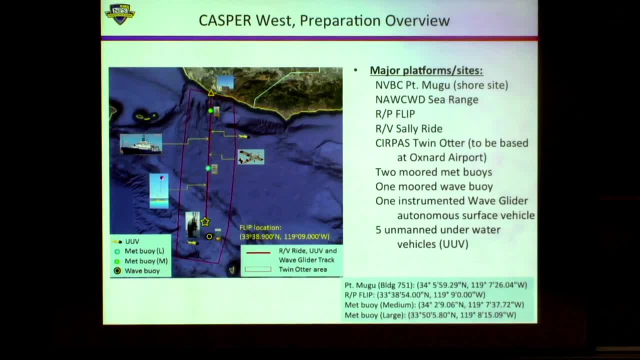 So and so this is a ship. when it's in transit and when it's on station, it's going to flip like this. So we use it as a stabilized platform. it's very stabilized. And then you know, it has arm, long arms. it's now going this way now. 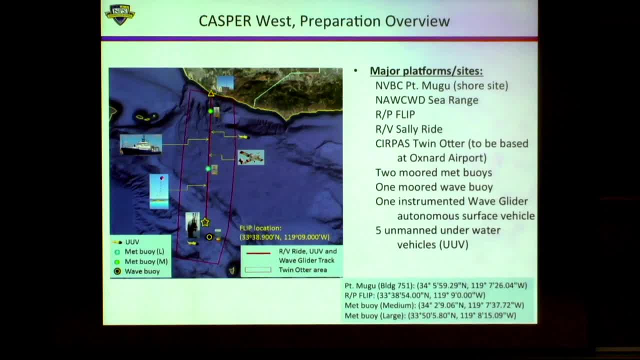 It has long arms to get into the water So we don't have flow distortion And that's what we need, you know, for measurement. And then again, you know we need to coordinate and we have this new boat, new ship, Sally. 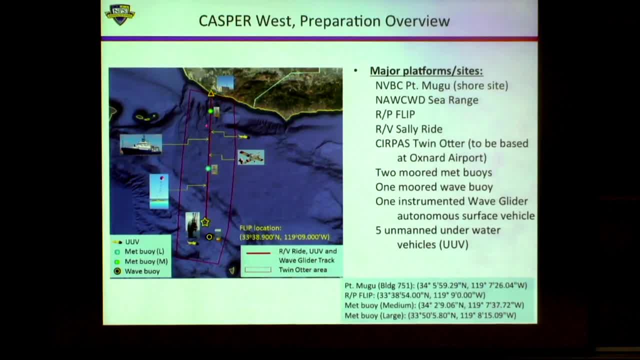 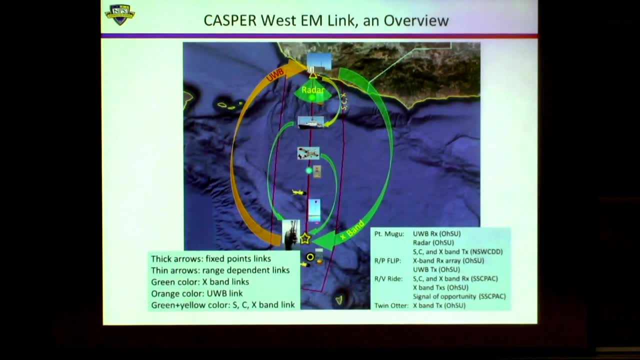 Wright is going to go in between here. The surface side will be here, And then we need to make plans about all the EM links so you can see all these. So this time we're doing it differently. You know, we want to measure lots of the fixed distance link and in different wavelengths. 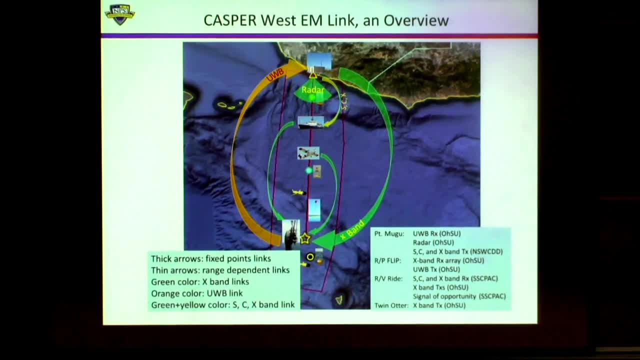 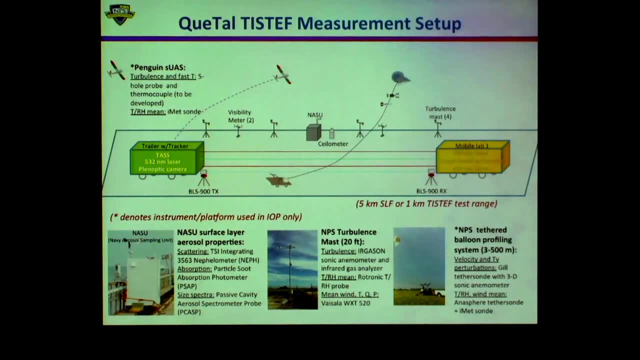 And then we also have the range-dependent links, you know. So there is going to be lots of orchestra playing in this project, Okay, And then we're going to have a lot of coordination as well, Now, so in Cattell, and so it's a different game. 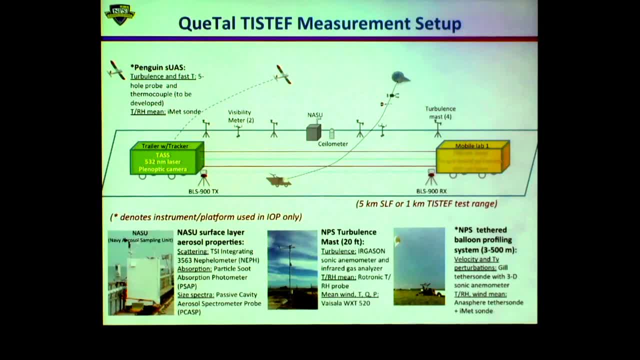 And this is for the optical and laser, And so this one is planned, you know, at the landing facility at Kennedy Space Center. So we have this 5 kilometer long landing pass and it's all corrected for Earth's curvature and everything. 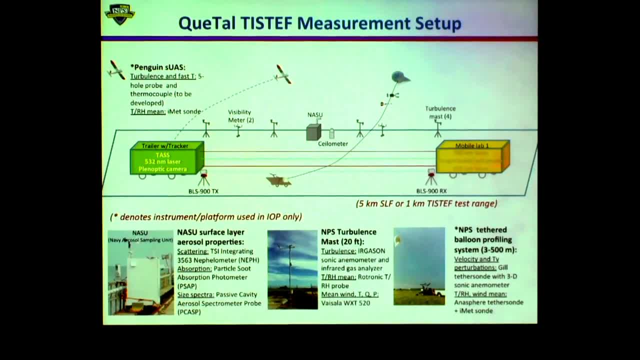 And so, and we want to put in the mobile systems- you know that- for laser. And then we want to put, you know, measure the atmosphere. We want to measure the atmosphere properties along the pass. and then, you know, use my tether. 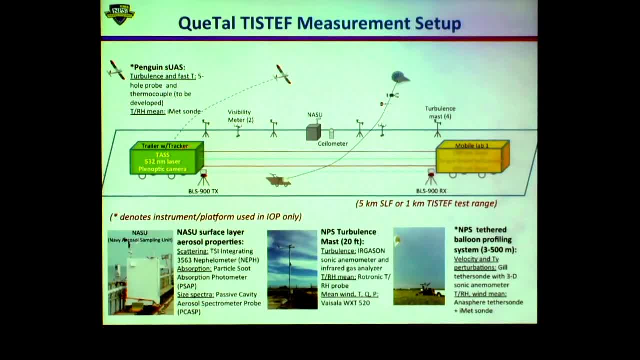 balloon and go up-down and then for the turbulence measurement And hopefully to use my small UAV as another project we're trying to develop, you know, using those toy-like UAVs you know from the hobby market And they're like only $200 a piece, so we don't care about losing them. 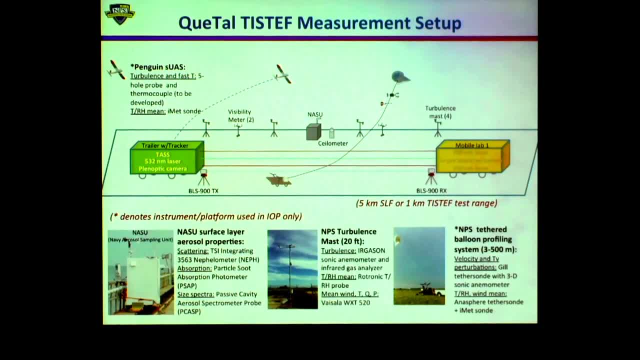 And then it's like radio sound, but you know we it has some reusability. So while we try to instrument these for turbulence measurement, if not turbulence, we at least we want to do the high-rate temperature measurement. so we can, you know that can help to support. 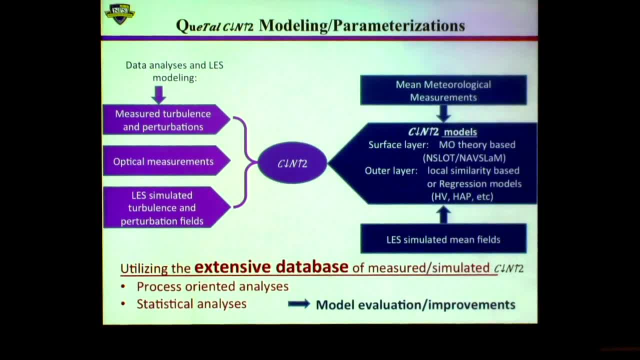 this high-energy laser project, And what do we do with this data We get? we better do something. Oh, this doesn't come out. well, This is C, and square and square should be on top. So now we have the measurement, and so this is like the plan, you know, for this one. 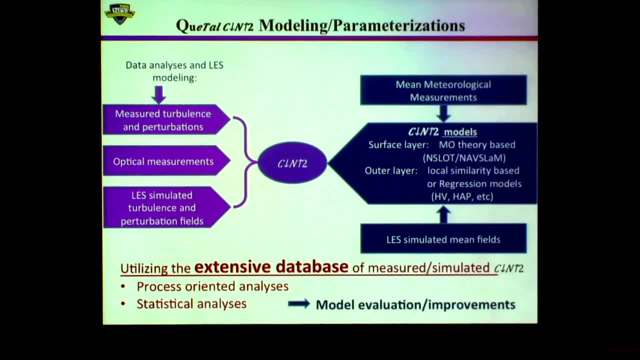 So measurement on one side And we also have this. So this very fine-scale model, its resolution is like a 20-meter or 5-meter resolution. It's called large eddy simulation model. They're trying to resolve the turbulence in the atmosphere. 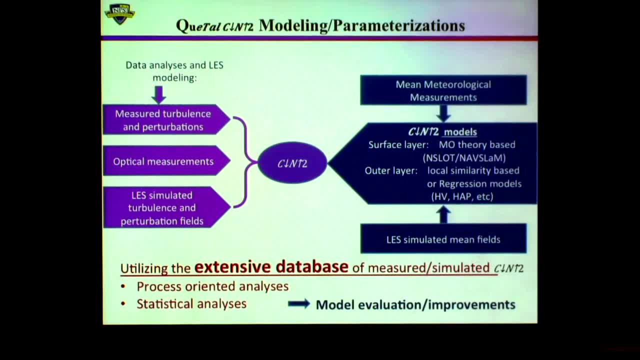 And of course, if they have such a high resolution, they cannot cover a large area, So it's only domain is probably two kilometer-ish, But that help us to understand the physical processes in the boundary layer, So we use that as data. 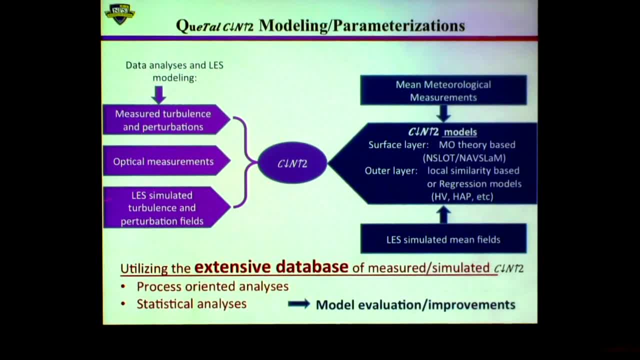 So we have the measurement of turbulent perturbations And optical measurement, The laser measurement, And then we put into this- This is the key variable we need to look into for scintillation- And then we have, you know, the other measure, the meteorological measurement. 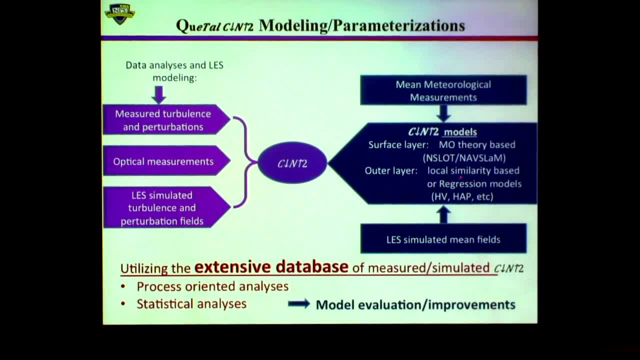 And it can go into these models, And then we can see what comes from the model you know. And then there's also the mesoscale model, the forecast model, And eventually we all come together to see how we can do the C and square better. 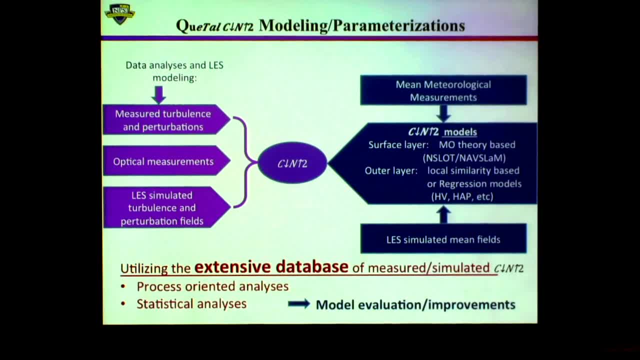 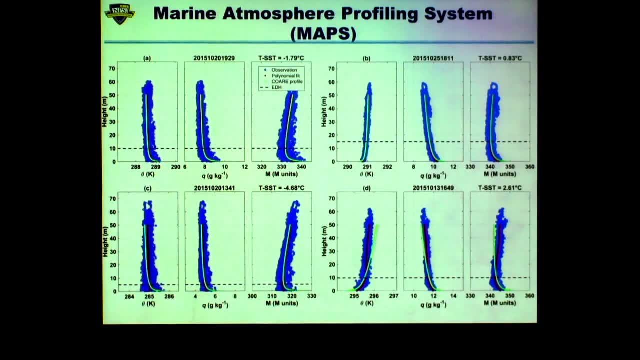 So that's basically the purpose of making measurement in this. Okay, And so now- and this is the measurement we did from the yoyoing on the small boat of Mausolini-Rib or the work boat in Casper East. So now I ask for seven up and downs each time. 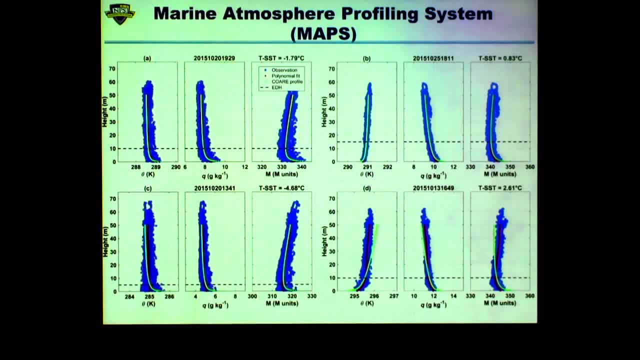 So this is what you see. Why do I want to make seven, you know, or more? Because you know it's a stochastic process. Every time you're going to measure something differently, Okay, So I cannot rely on just measurement from one. 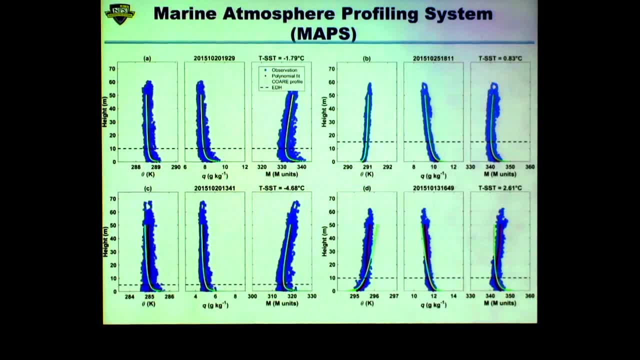 Because it's just one realization, One realization out of many happenings in this. you know stochastic process, So I need many, And then I want to get the mean. So you can see this green, the red line is actually is the mean. 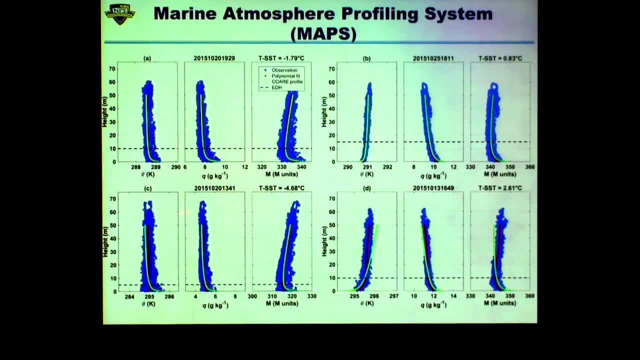 It's a polynomial fit. And then the green is a model, You know that, the one that I said most, the Monning-Opko similarity theory, And so you can see, in some cases, hey, the theory works pretty well. 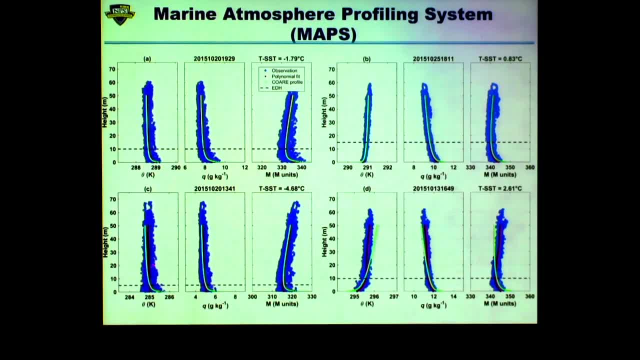 So we're all happy. But then you can see other cases. now the theory does not work very well And in these cases it happened to be: if you can see, the air-sea temperature difference is small: Positive, negative or positive. 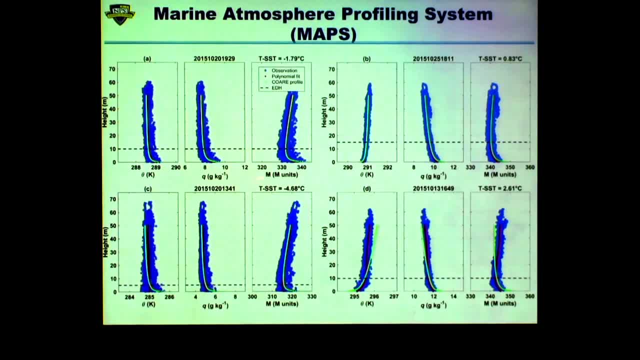 And then that's when the theory seems okay. Now, when this quantity become larger, and that's when, especially this one, this is the so-called stable condition. This is the exact condition I was trying to catch in the Santa Ana project, Because when you have the warm and dry, air comes in and you know so, you create the. 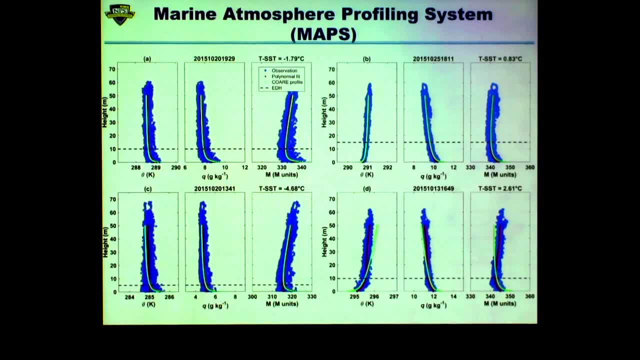 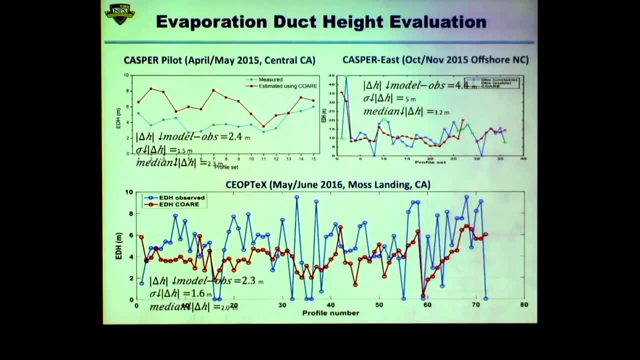 stable condition, And then you can see the significant difference. And so we use this and we can derive for the first time the measured evaporation duct height, Directly measured, And then we can compare with the model, which is this one, the core. 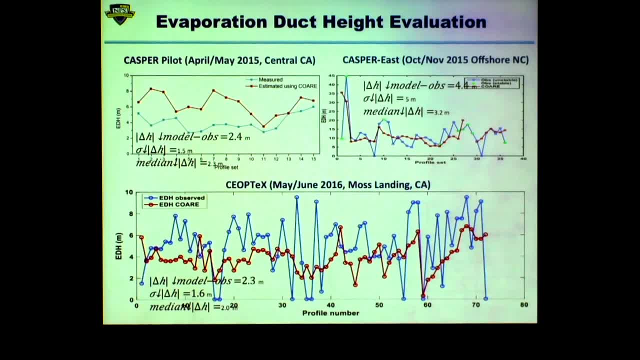 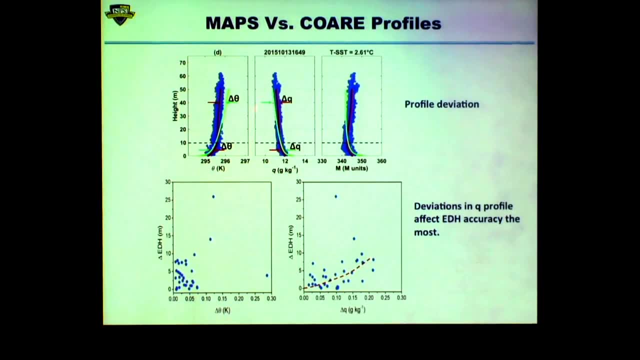 And then we can look into, you know, have a good evaluation of how the model is doing. And then we also, you know, to look into some theoretical study, to look into the differences And you know how this difference, you know, related to the temperature. 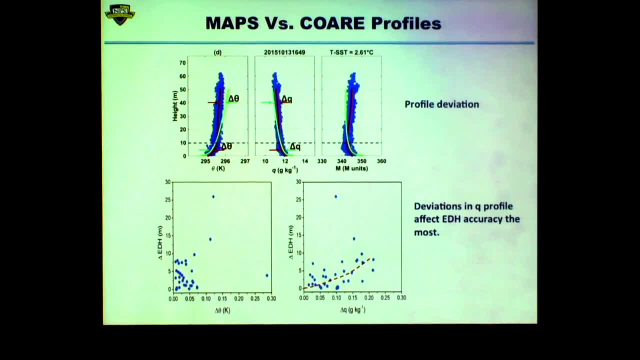 Related to other quantities in the atmosphere, For example the low level water vapor difference versus at the sea surface temperature at the sea surface. So we do some of these analysis, So we're not just collecting and leave it somewhere. So we've been working with it. 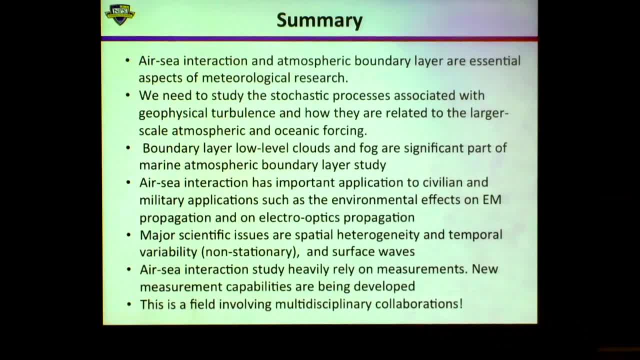 So come to the summary here. So air-sea interaction and atmospheric boundary are essential aspects of meteorological research. So meteorological research is not just forecast. There are lots of forecasts, There are lots of things going behind the forecast, you know, and to improve the physical, 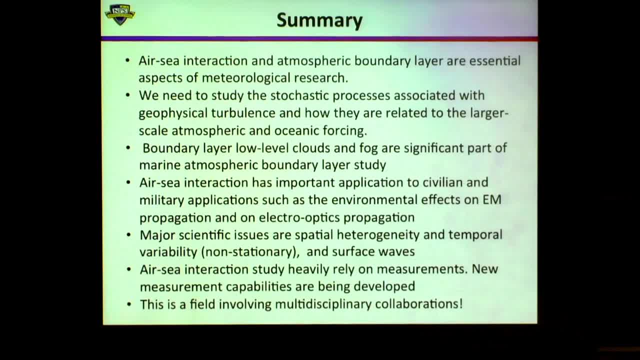 parameterization. I'm sure in your field of research it's similar. So improve the physical parameterizations and how we can forecast this thing better. And so now we need to deal with- you know, in the boundary layer research, the stochastic processes associated with geophysical turbulence and how they are related to the larger scale. 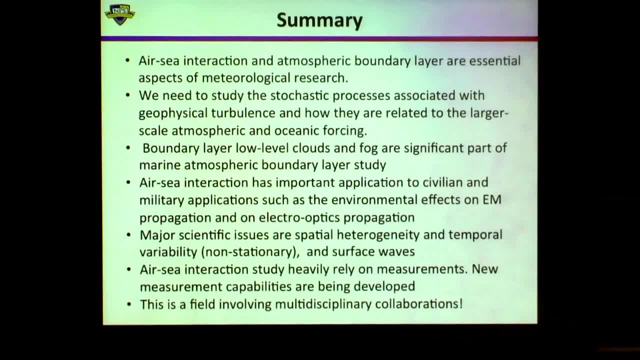 atmospheric and ocean forcing Because, after all, it's what's happening. What's going on in the surface is changing. you know what's going on in the atmosphere, So we want to make that connection. And boundary and low level clouds and fog are a significant part of the marine atmospheric. 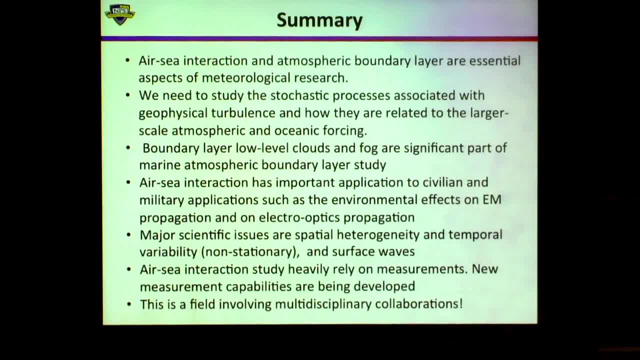 boundary study. So I will continue with those on that and we'll work with Candice on that as well. Air-sea interaction and has lots of important applications to civilian and military use, You know so, for example, for the EM propagation and for the. we call this EO. 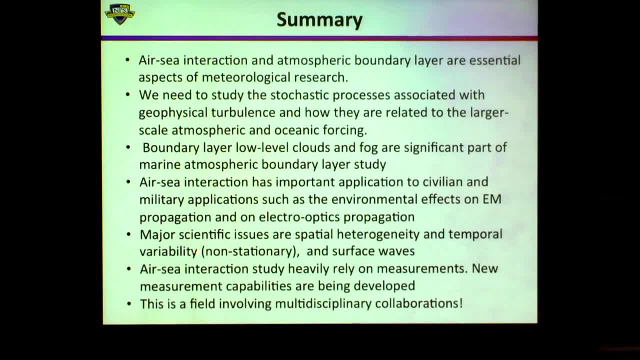 Electro-optical propagation. And so now the my major problem now is I need to deal with the work with the heterogeneity of the surface and non-stationary, which is, you know, along the same line, And you know spatial, horizontal inhomogeneity and temporal, you know, variability. 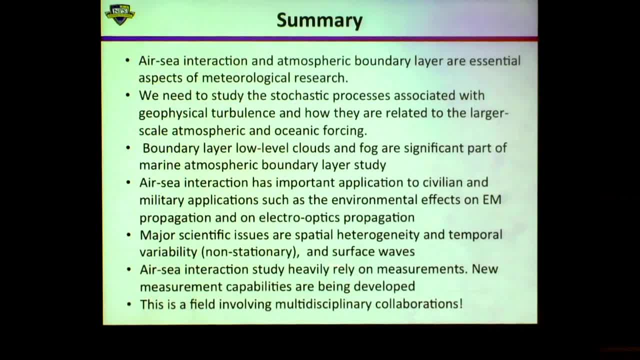 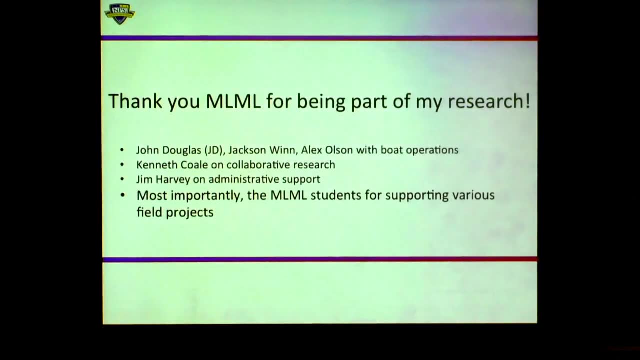 And also we need to deal with surface waves, And so our study are heavily rely on measurement. So we need to develop these capability as much as we can, And this is a field of truly multidisciplinary, you know- research, And so we need to involve a lot of people from other different areas. 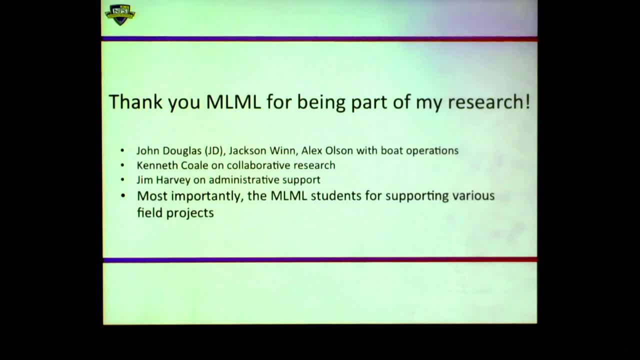 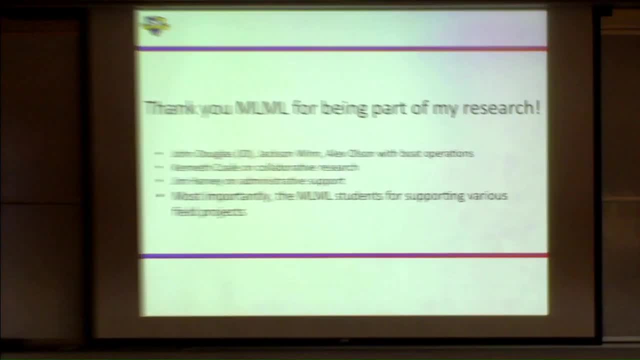 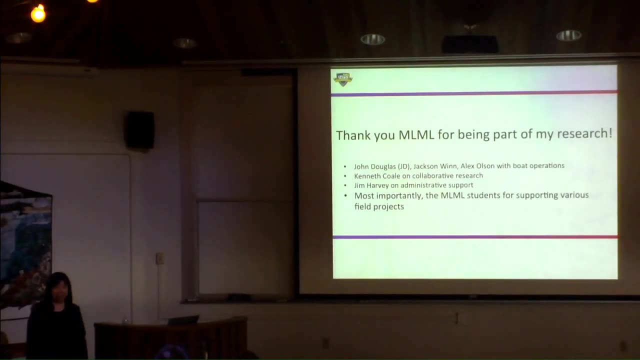 And finally, I have my big thank you to Moth90 for supporting my research. So I have a list of JD, Jackson, Alex, you know so, and they work really hard on the ship to get what we want And they are the best crew you know from all my experience, you know because they. 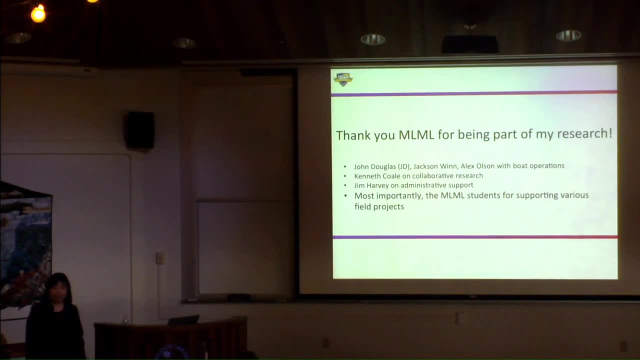 don't mind to go extra miles to get what we want. Thank you, And I think JD is even part of the science team. Sometimes I forget about stuff and he will come to me and he will say: hey, Chin, don't you want to do that? 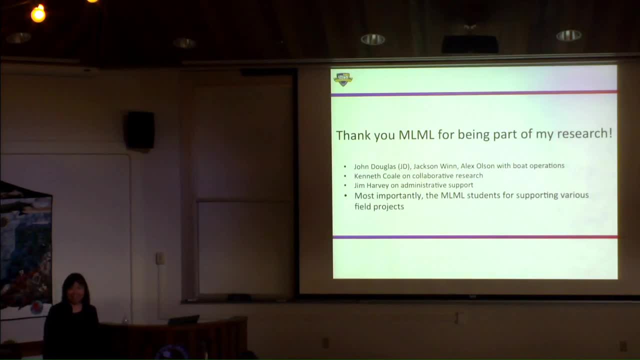 You know, I was like, oh yeah, right, right, oh, okay, I forgot about that. So that was really good, you know. So be careful, We are turning him into a meteorologist, So. and then, Kenneth, of course you know help, and so we are doing collaborative research. 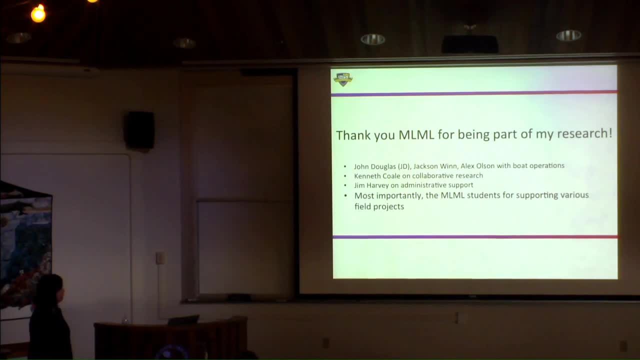 and Jim, you know, for all the administrative support And, most importantly, the students. You know these, you know these students. you know you are so helpful. you know I'm really grateful to what you have been doing for my research projects. 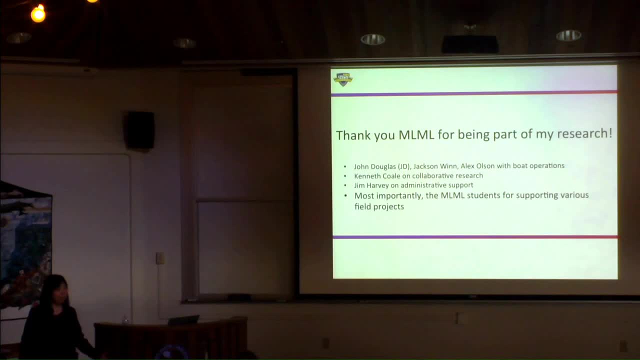 And I hope you had fun too And I'm hoping to involve you more in the future, you know so I can see I'm not short of field programs. So if you you like to get on to the sea or sometimes maybe get on the plane, you know. 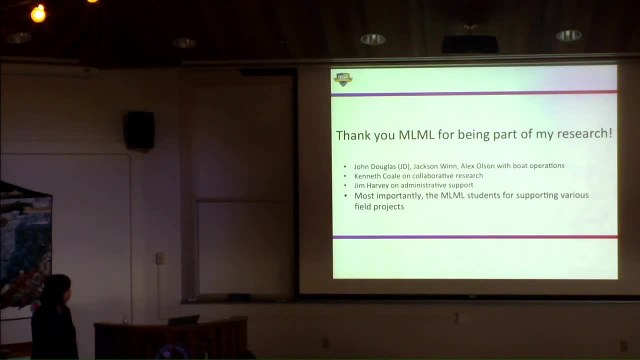 so that's also possible. So, yeah, if you are interested or have any questions about meteorology- general meteorology. so I'm still a meteorologist, even though I have the boundary layer in there, okay, And so feel free to e-mail me, ask questions, you know. so yeah, so hope to you know, enjoy. 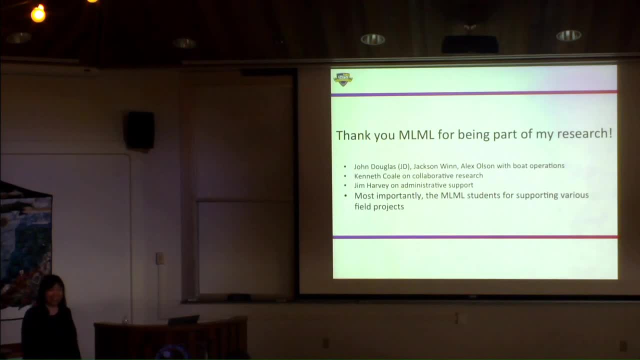 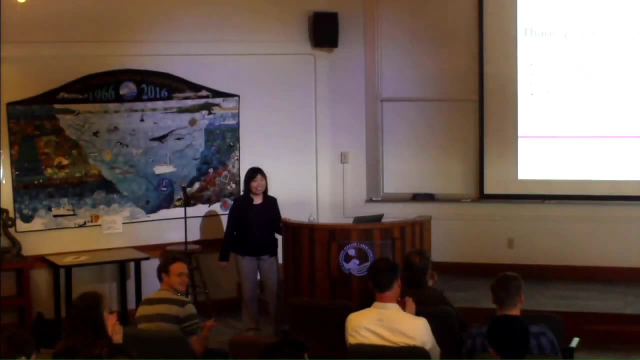 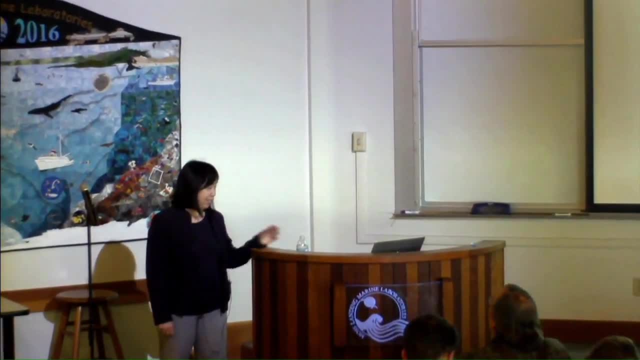 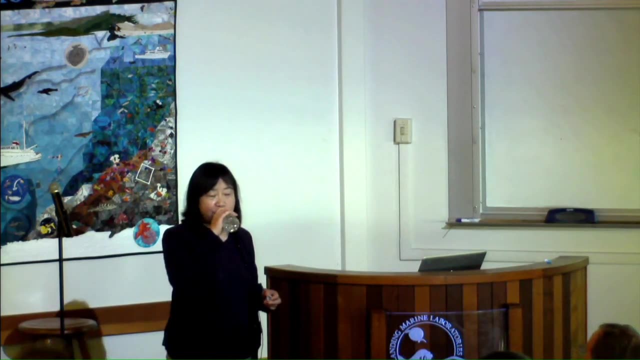 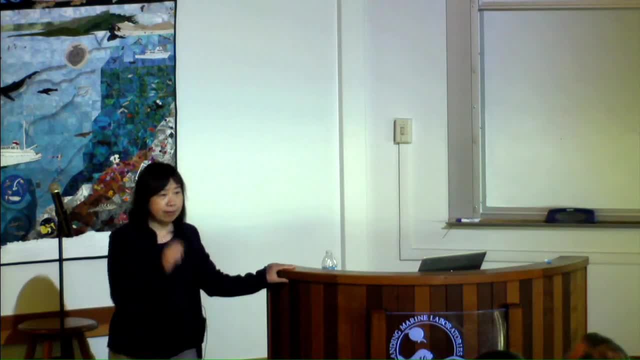 And so what? what's the extent? what's the range of the duct? Okay, The the duct ranges from like a meter to anywhere you know 30 meter, But most frequently we see 10 meter. Now, here when we make the measurement, 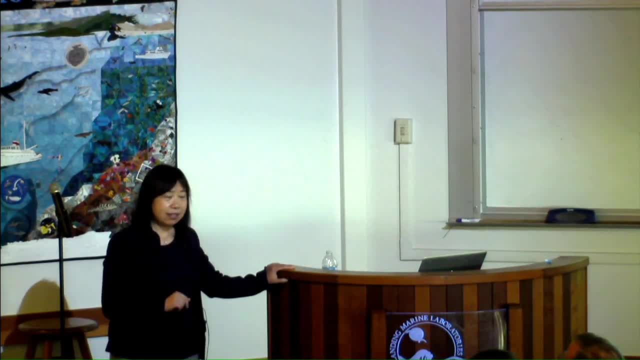 And we're looking at 4 meters, 6 meters, And so that's a bit too low, because I want it higher And that's why we're moving to. we're going to Southern California, where we have the higher sea surface temperature. 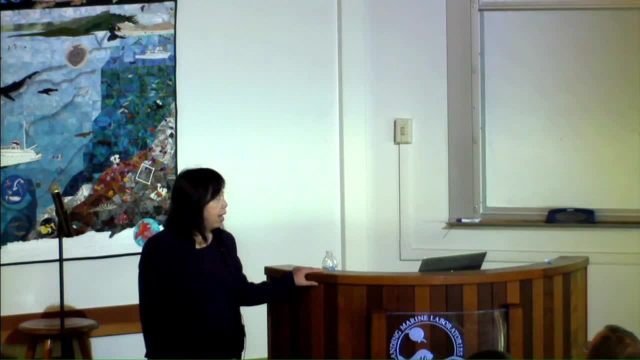 And that gives us a higher duct, And so, yeah, I would love it if the conditions here is right. That can save me so much heartburn going to Southern California. So there must be a relationship between the height of the duct and the propagation of the wave. 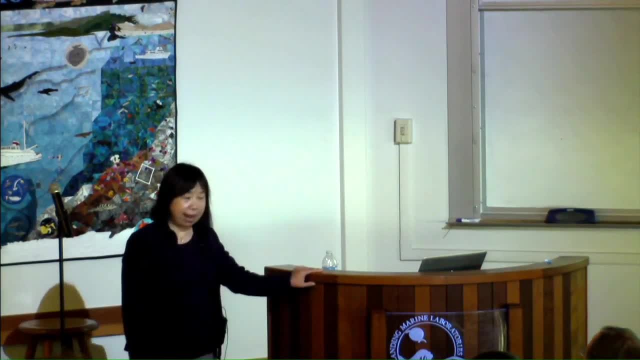 or the wavelengths of the electromagnetic signal to the body. Exactly, There is a direct relationship. So formulation you can calculate Like a certain duct height is going to trap certain wavelengths And some other wavelengths don't care. So there is a formulation for that. 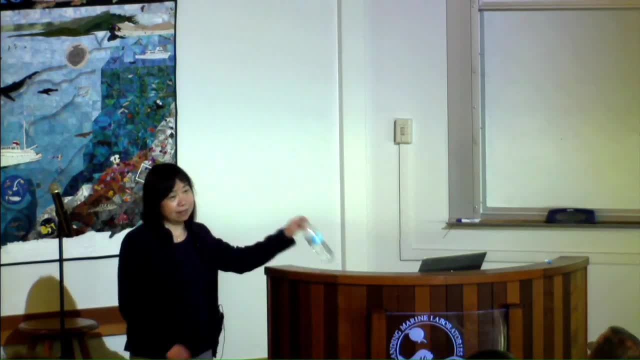 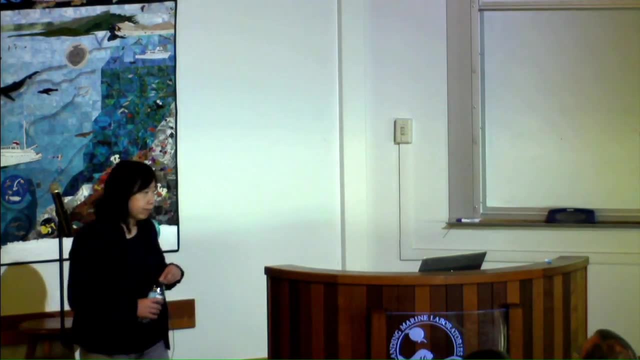 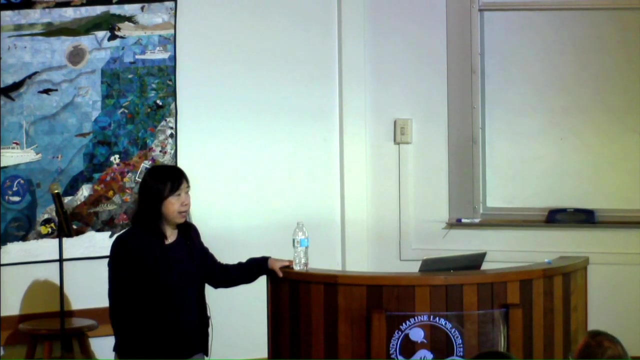 And so that's got to relate to aspects of the duct. So the mirage that you see right along the sea surface is that? because those signals will be propagated differentially along the water? I think it might be related. Now, however, the mirage is more of an optical phenomena. 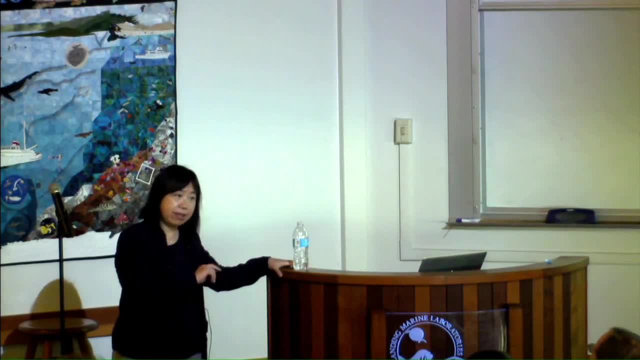 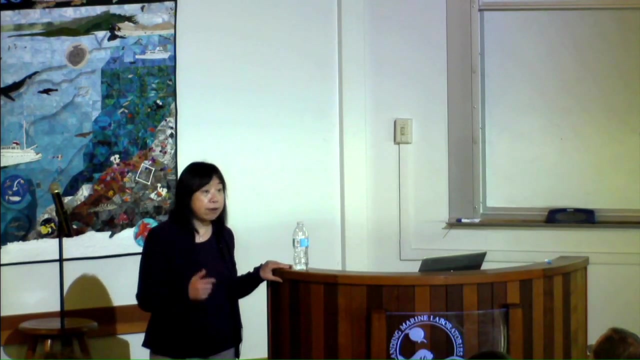 And the ducting is more in the radio waves, the longer wavelengths, So X-band right, X-band, C-band, S-band, so even L-band, solar. But nowadays there are more interest into the higher frequency, one go into the K-band. 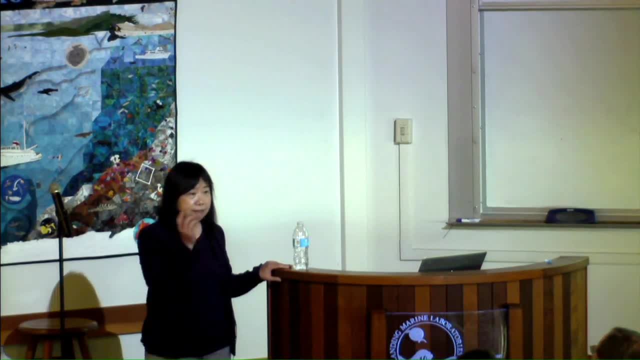 I think there is some classified research in that. So in my project the program manager always wants to have put like a trailer in there, And so we don't know what's going on. So there's a trailer there. So there are some frequencies of interest. 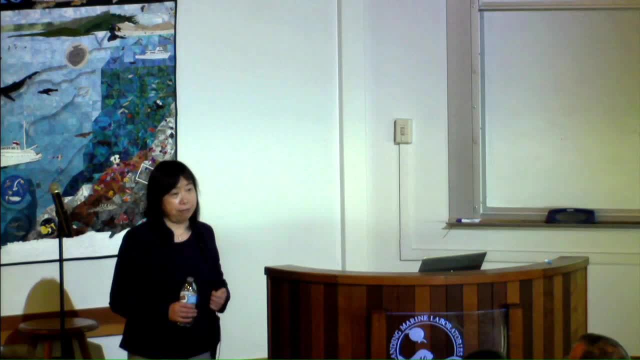 The higher the frequency, The harder it is to make measurement- And you also talked about the communications aspect- And those are typically in the 2-meter grade lengths And 2 to sometimes 4 meters in terms of radio. Are these grade lengths being affected by the ducting? I think it depends on the duct height, So I don't know exactly. You know, for certain wavelengths, But I remember I think in the old days when they started it's all for the lower frequency And it's only nowadays it's getting higher and higher. 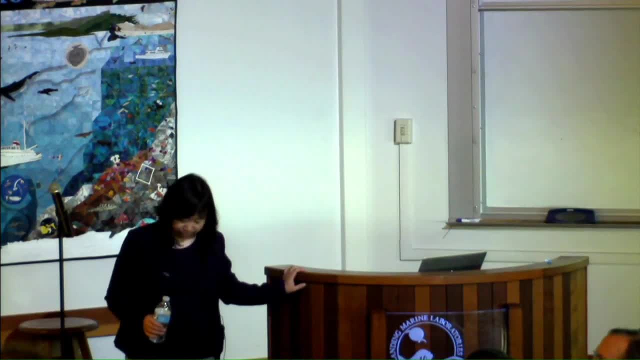 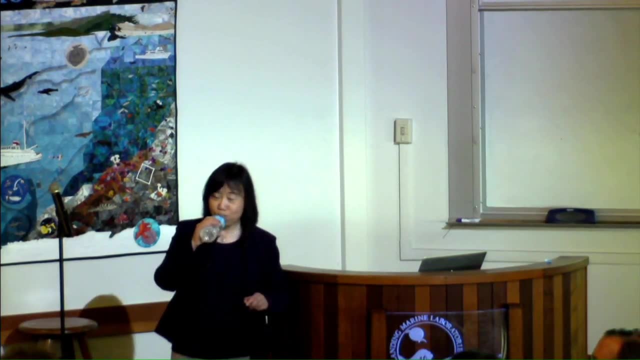 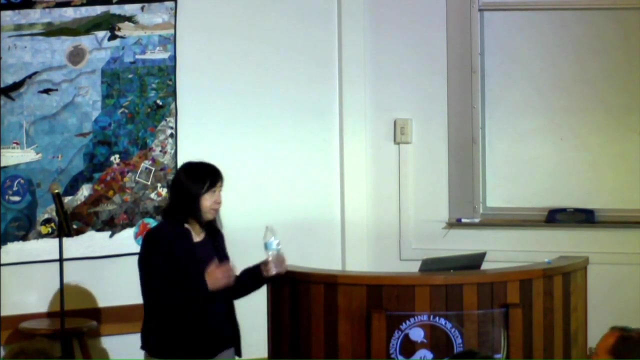 Well, my first question is: when you showed those aircraft measurements of temperature and you saw all those spreading in the data, all those spreading variations, how big were those And what do you think is driving that small scale? Well, if we're talking about gradient, 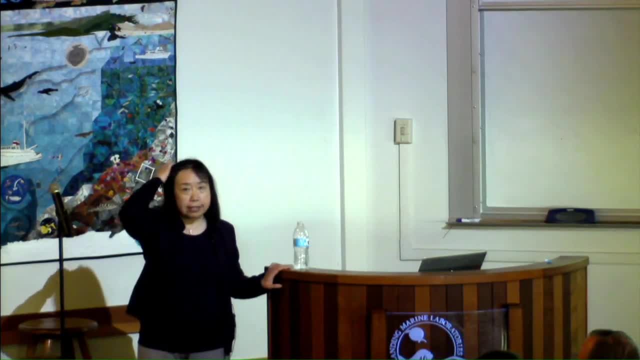 it varies quite a lot. Now, what I realized in doing, like my students working on coupled air-sea, coupled model forecast model, I realized the ocean, the diffusivity is so small, So it's the mixing. The time scale for mixing takes a long time. 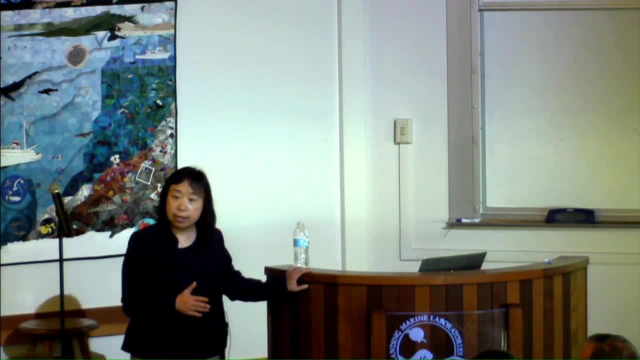 So the gradient. very often you see really sharp gradient And simply because there's just not much horizontal mixing, Unlike in the atmosphere, you have something warm air and cold air here And very quickly they mix out, But in the ocean this process is very slow. 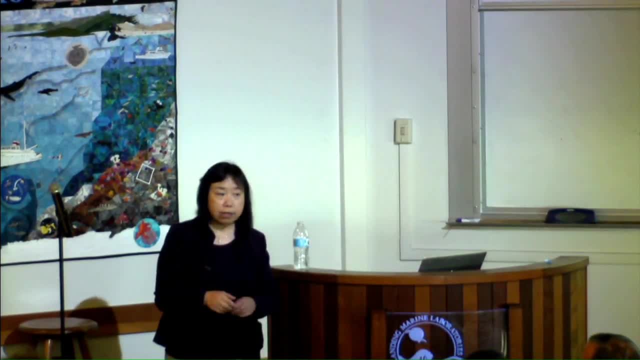 Now, when we were in Casper East and off by the Gulf Stream, and so there was one day we have this gradient like like two degrees within I don't know meters, So I thought my sensor was wrong. I look at my sensor: it's going like poof, like that. 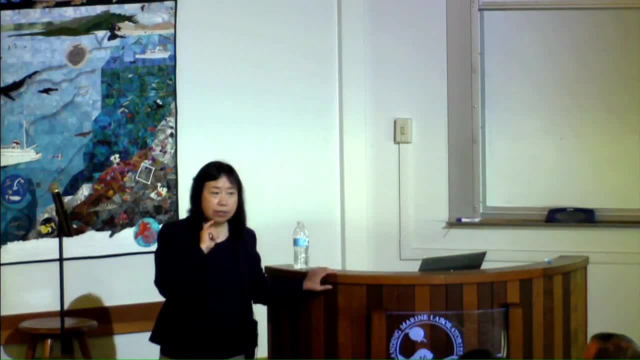 And then so I said, oh, this is not right. And so I went to the ship flow through and I see the same thing. So it was amazing. So this happens more often than not, So I think it may have to do with the ocean diffusivity. 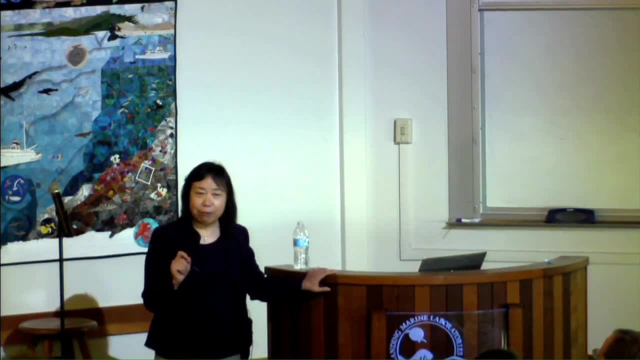 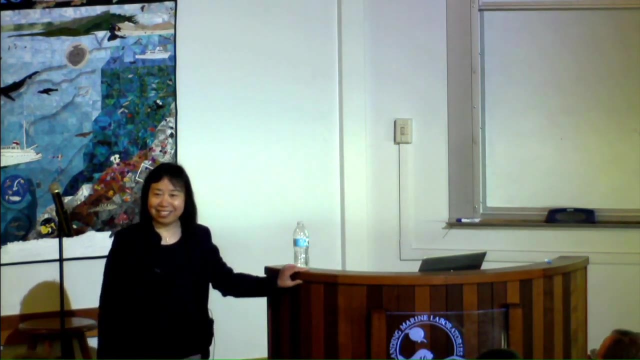 But I'm no oceanographer, so I think we do have an oceanographer on board And he's very interested in getting answers to these. So Kip Shearman from Oregon State- I don't know if you know him, But he's pretty good in these things. 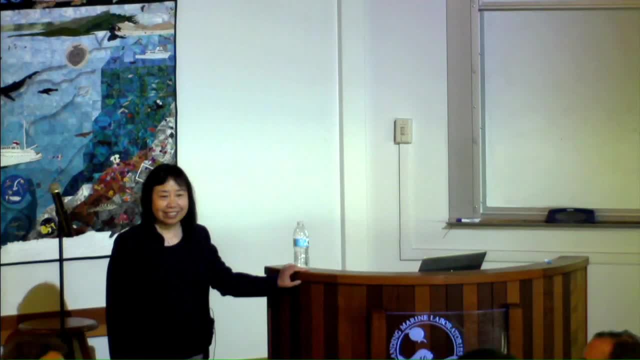 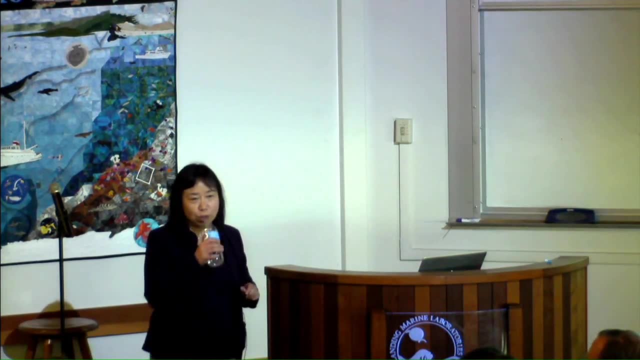 Yeah, I was going to ask. you mentioned that in the forecasting models the SST is one of the hardest timers to forecast. Are the sources of the errors in those forecasts relatively well understood, or is it completely unknown? Nope, that's a very good question. 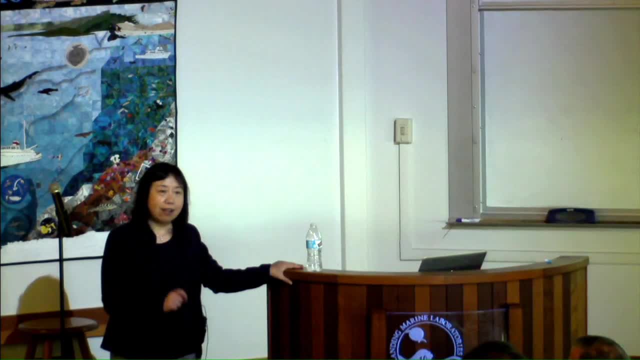 Now it's not only hard to forecast, it's also hard to validate, Because it's very difficult to measure it accurately Now. so what happens is at the ocean surface, at the very top surface, it's like at the cloud top. 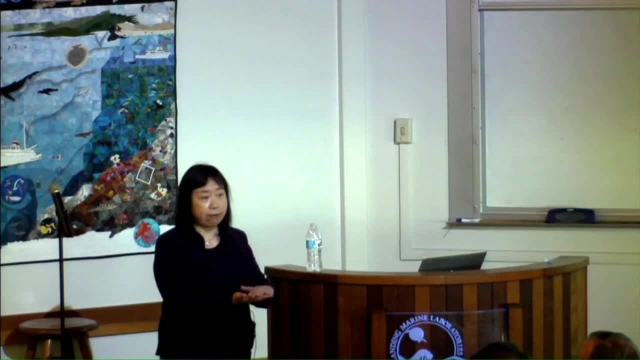 So the ocean surface is emitting more infrared radiation than what it's getting. So there is a cool layer At the very top of the layer. it's less than centimeter, maybe millimeter or less, And that's cool. And so it is this cool surface that's. 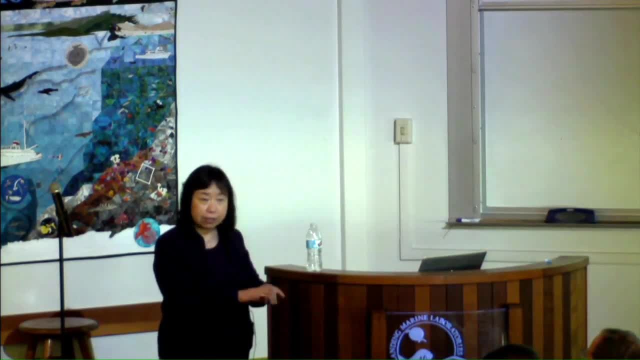 where the atmosphere feels. So we need to measure that surface. So imagine all the ship flow through data. It's way two meter, one meter. So we're not getting that. And then if you stick a thermometer in the water, you're also not getting that. 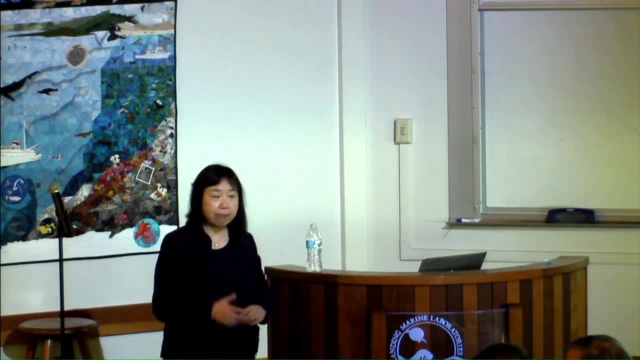 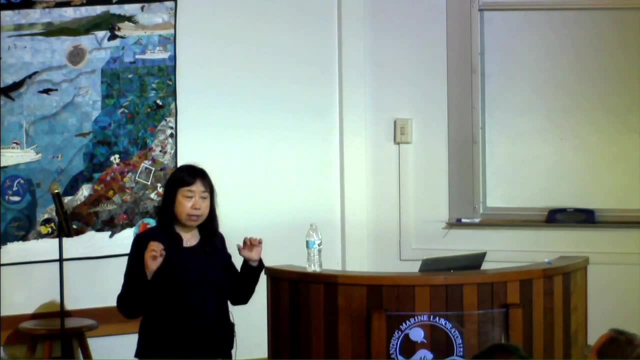 And not to mention you have the waves and stuff it's in there. So we want to use these radiometric method, So basically measure the radiation, But you are always some distance away from the surface, like on a ship, And then there is lots of water vapor in between. 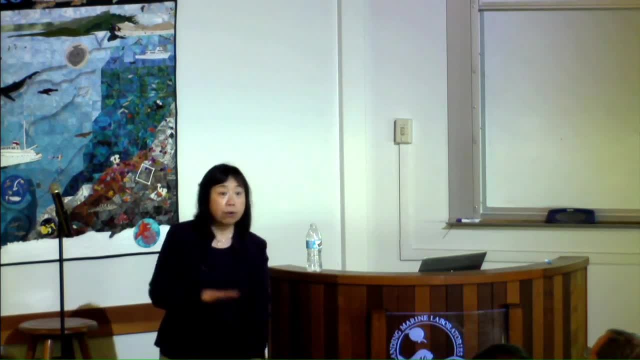 So you need to somehow get rid of those water vapor effects And in addition, you also have the reflectors from the sky getting into your camera, into your lens. So now my new gadget is called. it's called the Rosar, So it's a calibrated sensor. 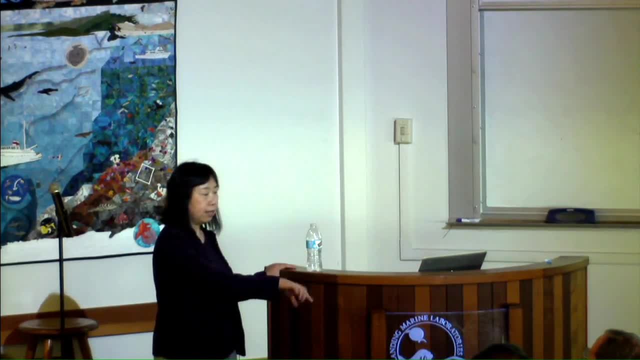 So it basically is looking at the sea surface And then it has a mirror to let it look at the sea surface and look into the sky, so for the sky correction, And then it looks back into two black bodies source, And so that way it's calibrated. 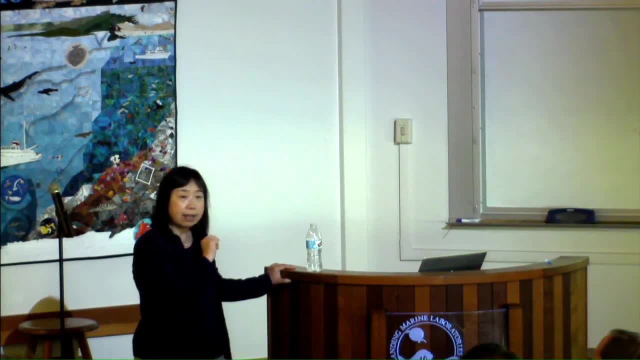 So we get the calibrated sea surface temperature Now I only get this for Casper East. I didn't have this. I had this before, So now it's a must have for my project, Because that's the only way I know what's the sea surface temperature. 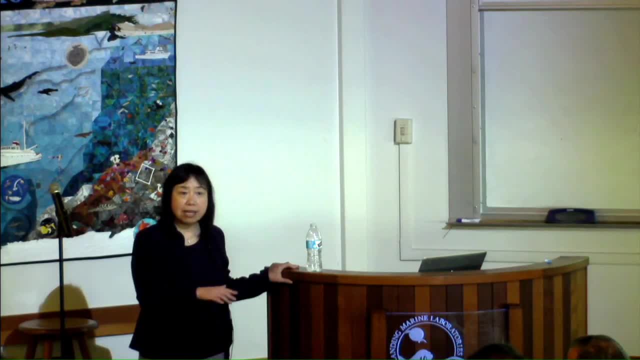 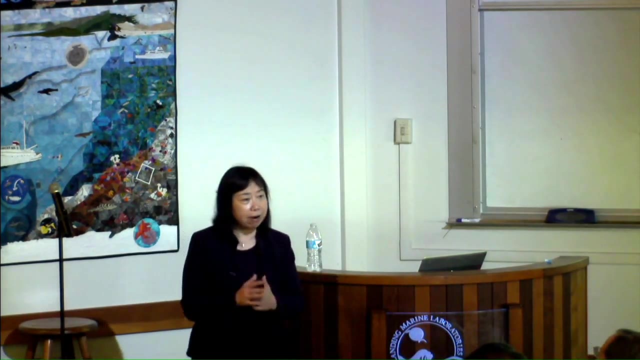 And we have gone through in the Casper analysis meeting, gone through so many times about exactly what is the sea surface temperature, Because the other ship don't have my gadget, So we're trying to find the time when that ship is close to where we are. 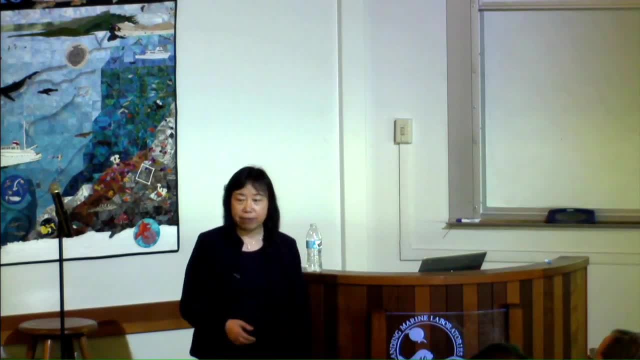 And then make the connection And then try to do the correction And we call it the cool skin and warm layer correction. The cool skin is that very top for infrared And there is also this warm layer because of the solar radiation absorption of the top water. 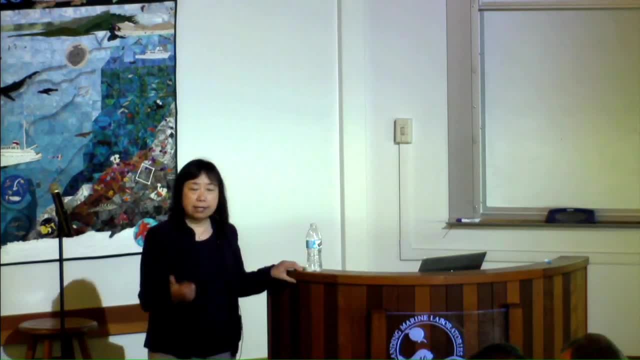 So these all? because now, when you want to use the flow through, and then that may be below or in that warm layer, So we need to make that correction using some mixed layer assumption. So there are some models for that. Yeah, that's a super good question. 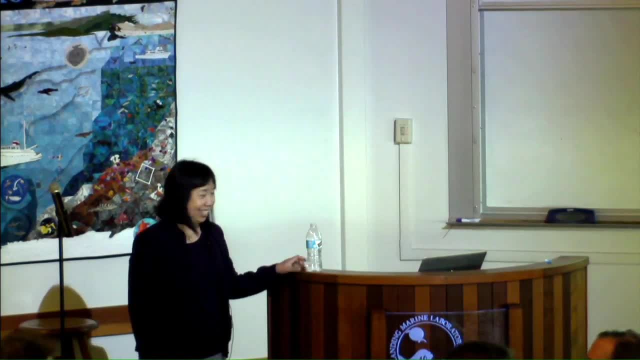 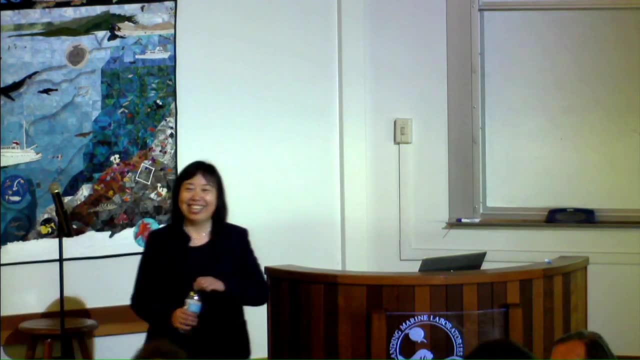 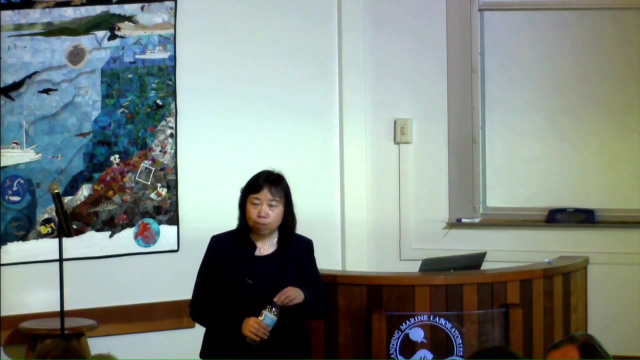 Well, thank you very much. Well, Alex, please The word state AUDs. was there any interesting information that came out of that? Because they were, we were sort of on the backboard on the track They were deployed. I don't know if anything interesting came out of that. 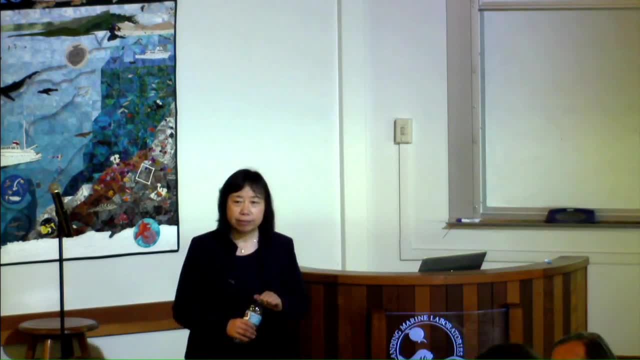 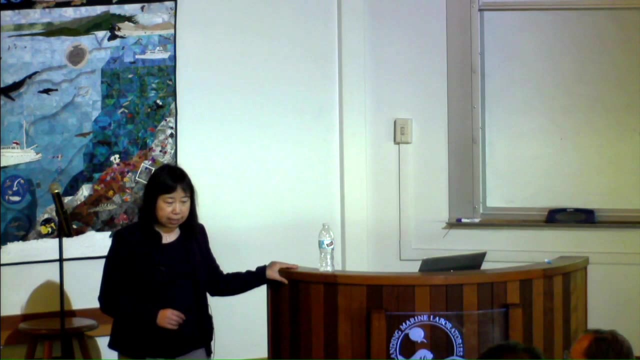 The AV, The AUD, I think it was the two, the torpedo, the fins, I don't know what you say. I think they were deployed in that. Oh, you mean the? yeah, the ocean gliders, Yeah, Oh, okay.